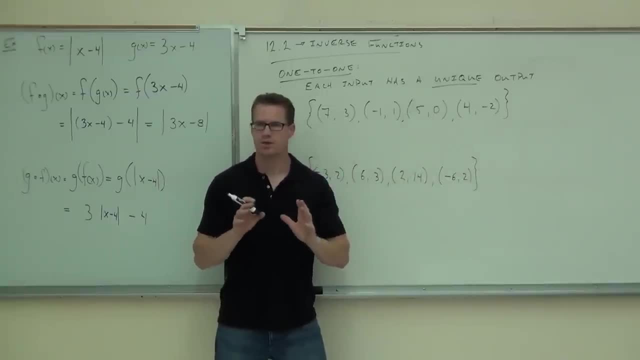 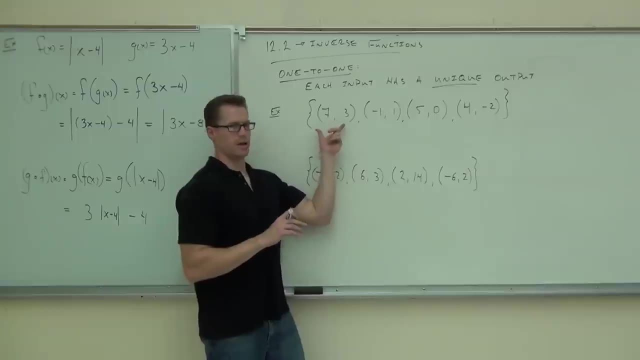 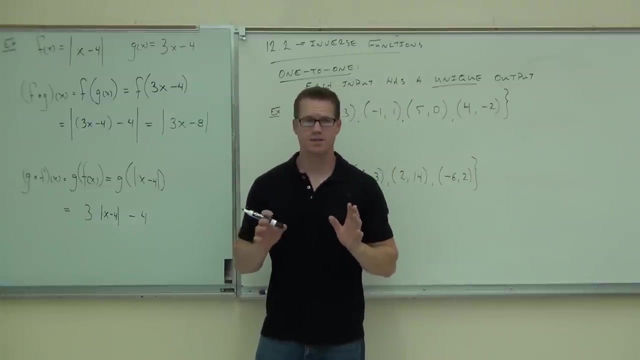 What's your, what's your x coordinate for this point? What's your y coordinate? everybody 3,, 1, 0, negative 1.. X's are known as inputs. yes, Y's are known as Outputs. 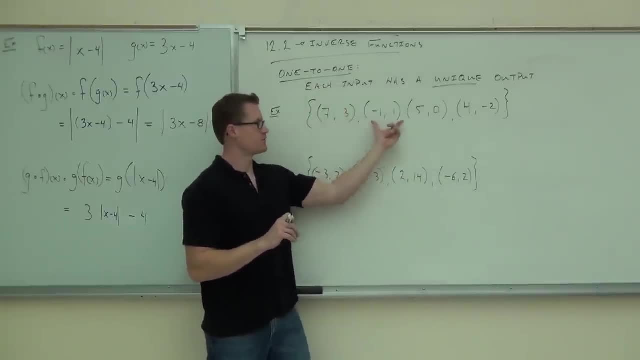 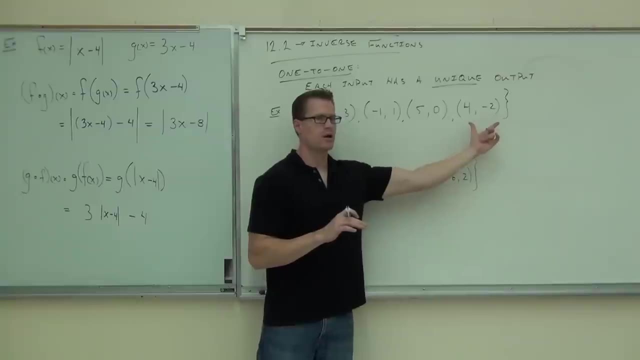 Outputs. What are your inputs here? Negative 1.. Negative 1.. What are your outputs here? 3, 1, 0, negative 1.. Here's what 1 to 1 says. It says you look at your outputs. 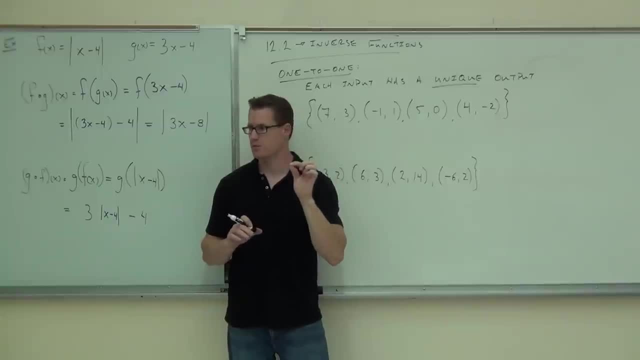 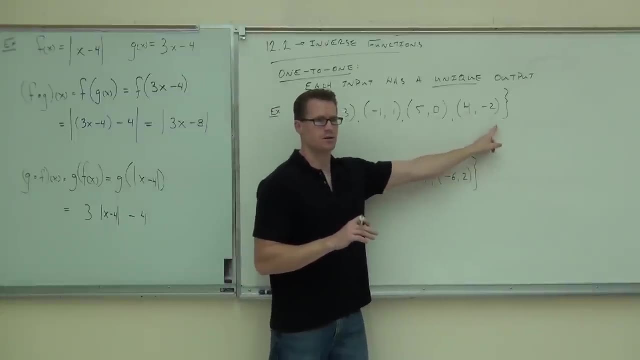 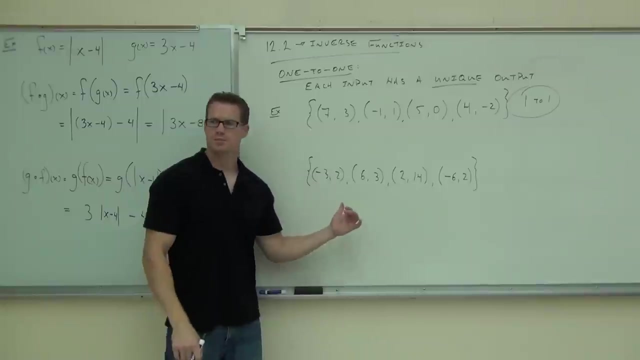 For each different input you must have a different output. So every output has to be unique, has to not happen again. Do any outputs happen twice? No, This is 1 to 1.. Read me your inputs here, ladies and gentlemen, please. 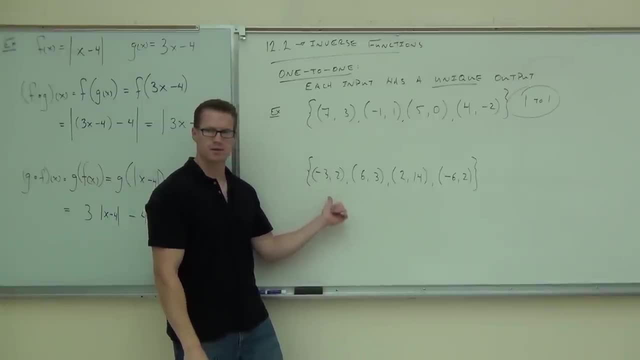 Read me your inputs, please. No inputs. No inputs: 3, 6,, 2.. Yes, What are your outputs, please? 2,, 3,, 14,, 2.. Do any of your outputs happen twice? 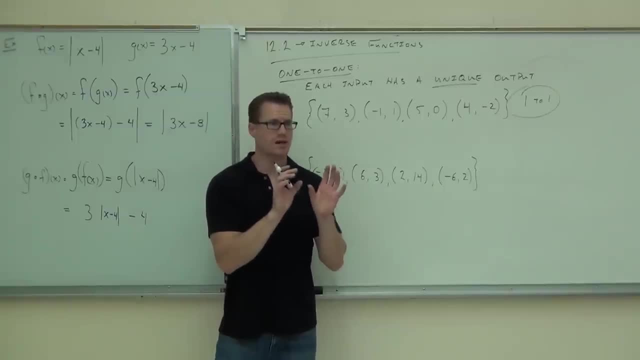 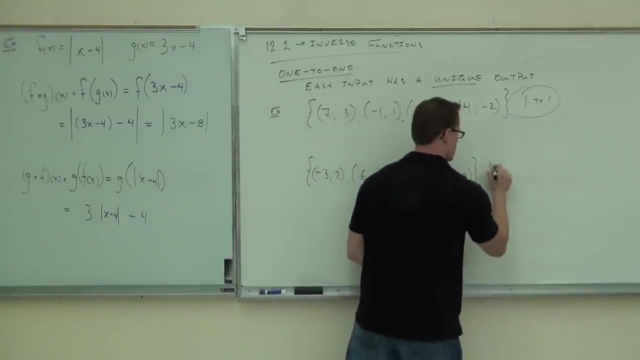 Yes, do. If your inputs happen twice with a different output, it's not a function. If your outputs happen twice, it's not 1 to 1.. Do you understand the idea of 1 to 1?? Yes, Outputs are unique. 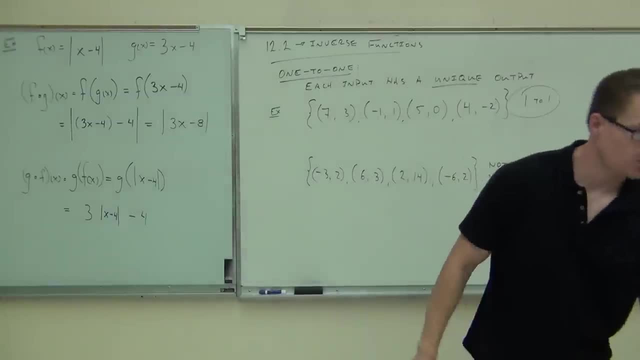 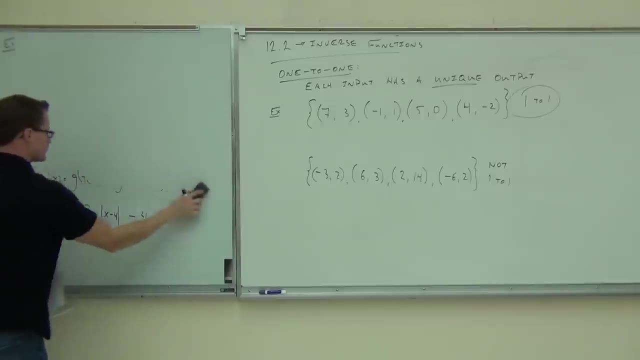 They don't happen twice. Now, one thing that we can do: oh, we have, that's awesome. One thing that we can do: We can talk about this according to the horizontal line test. Now, you've already had something called the vertical line test. 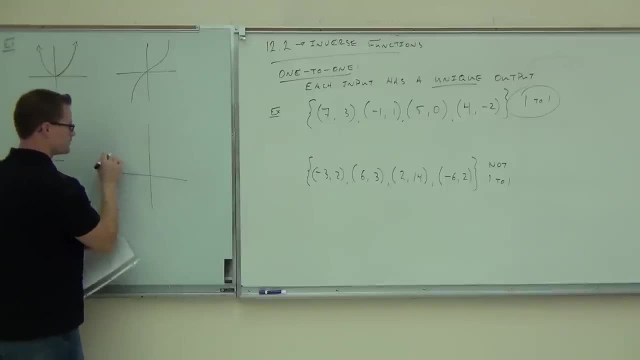 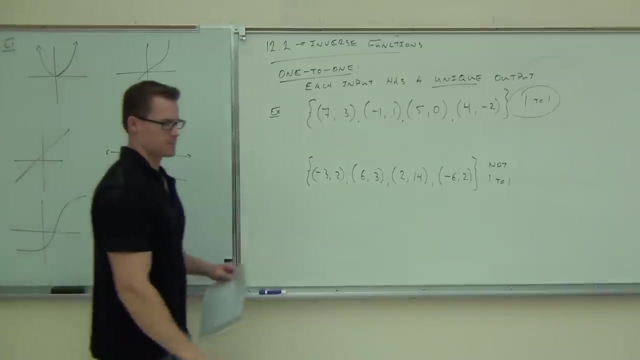 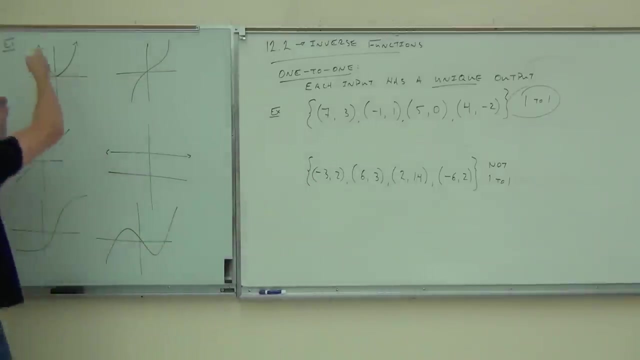 The vertical line test tells you whether something's a function or not. The horizontal line test will tell you whether something's 1 to 1 or not. So first thing, let me refresh your memory on vertical line test. Vertical line test says: imagine a vertical line. 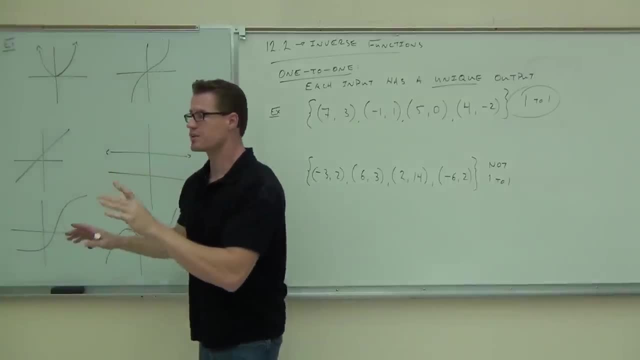 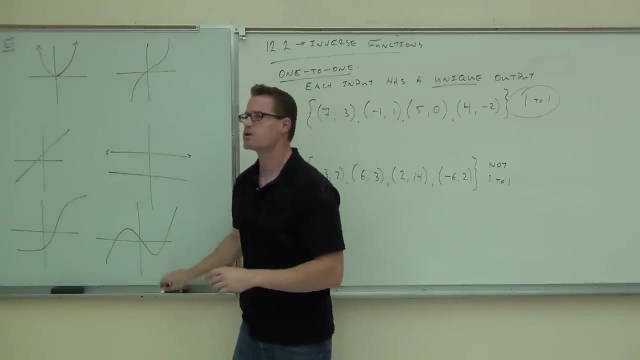 If it hits the graph at more than one spot, it's not a function. Note that all of these are functions. Everyone passes the vertical line test. Do you agree with that? Okay, Horizontal line test says: instead of vertical, this means horizontal. 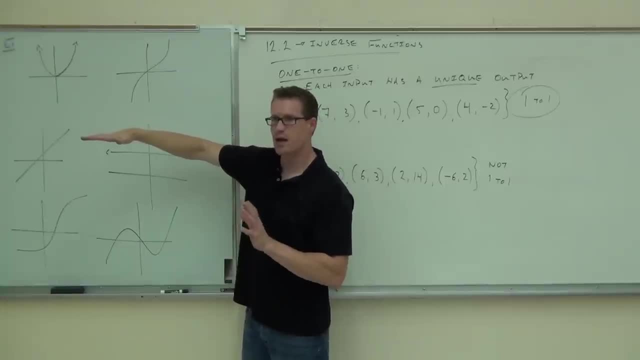 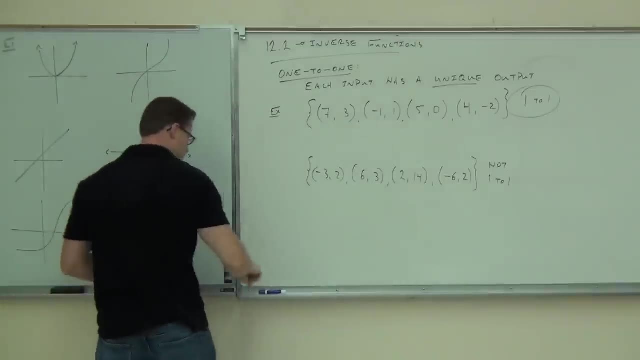 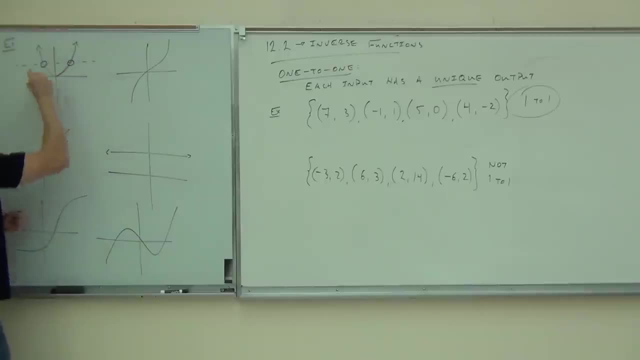 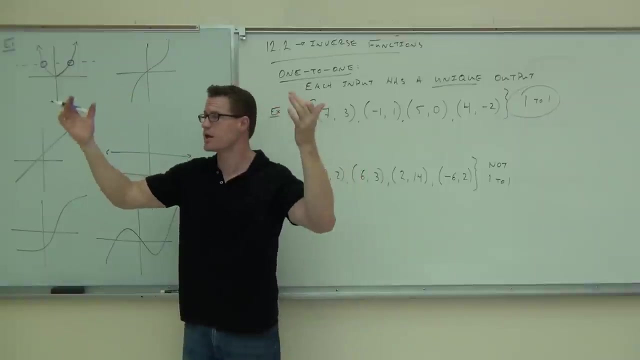 Horizontal line touches this at how many spots? That means you have the same output twice. Do you see it? Same output twice. That means this is not one-to-one. So the horizontal line- this will tell you that This is not one-to-one. 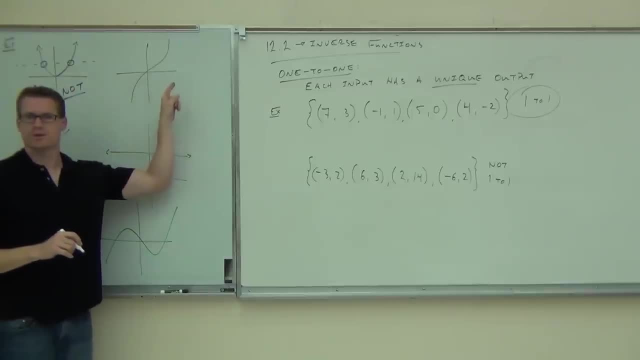 Is this one one-to-one? What do you think? Horizontal, Horizontal- Does any of those touch it twice? No, That's one-to-one. How about this one One-to-one or not? folks, What do you think? One-to-one? 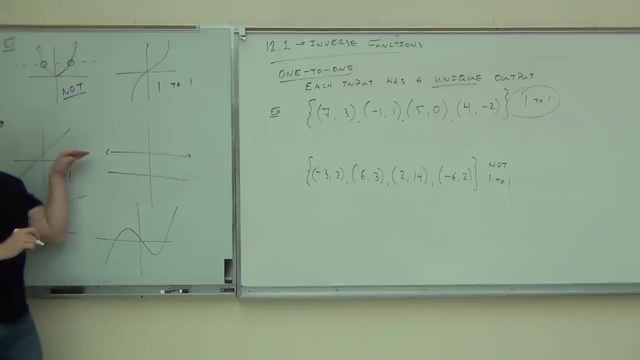 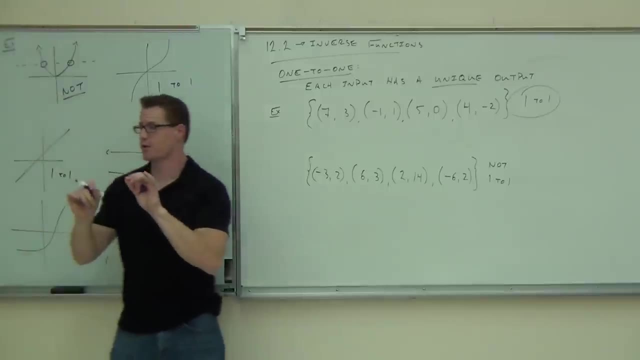 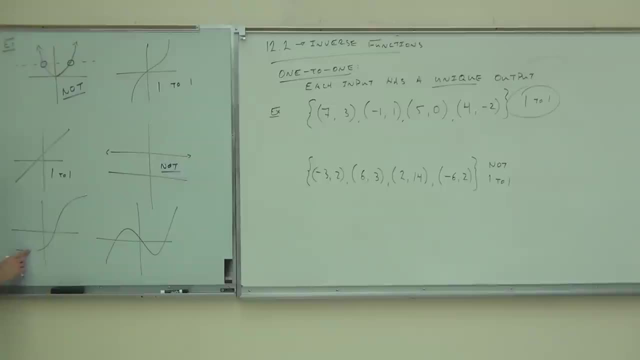 How about this one? Look here, Well there, How about that one? Is that one-to-one or not? What do you think? Yes, Absolutely, It doesn't cross over anyway. right? That means that every output only happens one time. 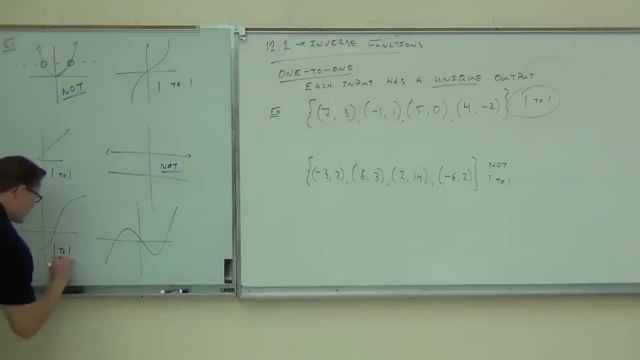 They're unique outputs, So one-to-one? How about this one? Is this one one-to-one or not? Definitely not. In fact, you get three spots here, not one-to-one. How many people understand the idea of one-to-one? 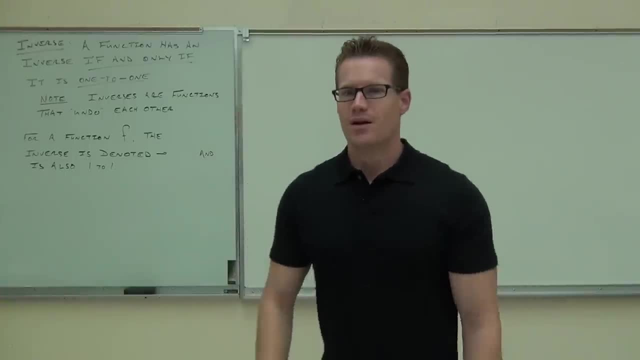 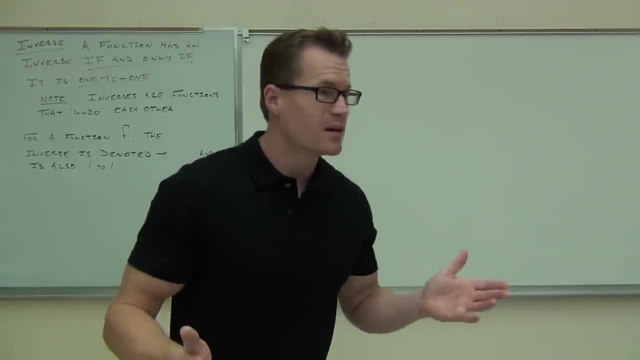 Good, That's fantastic. Well, good, It's annoying. OK, So we have these things called inverses. Now I haven't even told you what an inverse is yet, So let's talk a little bit about what an inverse is. 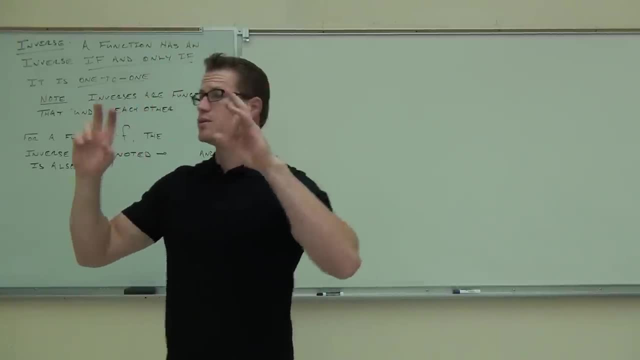 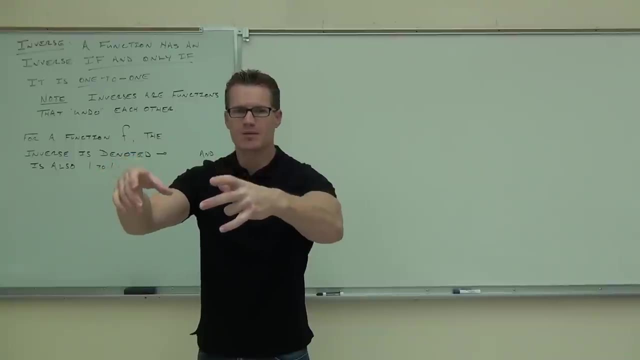 An inverse are these functions that quote unquote undo each other. So here's what that means. It means if I plug something into a function, then the inverse should take what I got out and give me back what I plugged in. 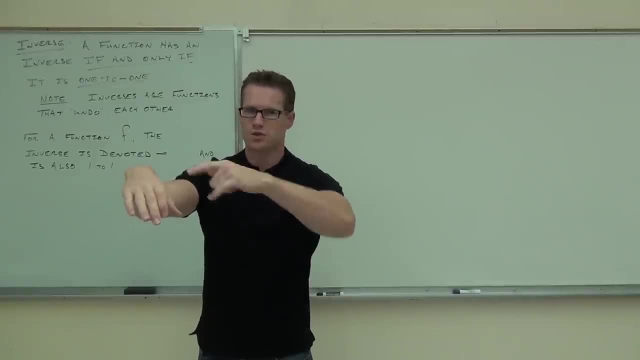 So it's like if I plug in a number three, it goes through this function. The inverse will take that output and give me back what I got out. It will give me back three, So it will basically undo everything that you did. It's kind of like this: 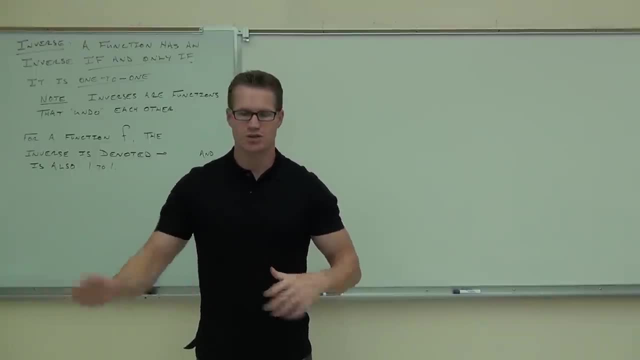 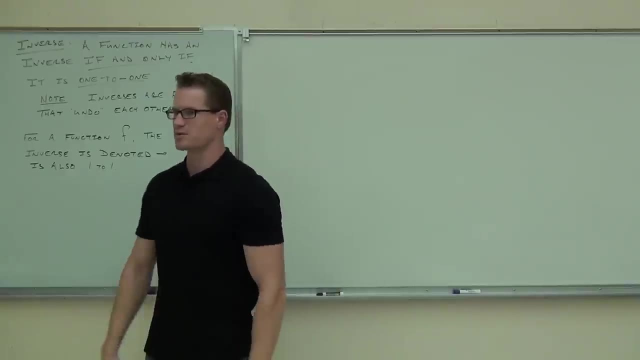 Like if you were cleaning a house and this guy came behind you and just messed up everything that would be your. he would be your inverse. So like you'd go clean the kitchen and he would come along and put everything back the way it was before you cleaned it. 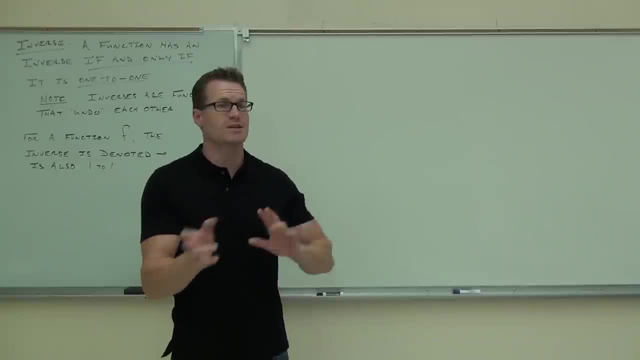 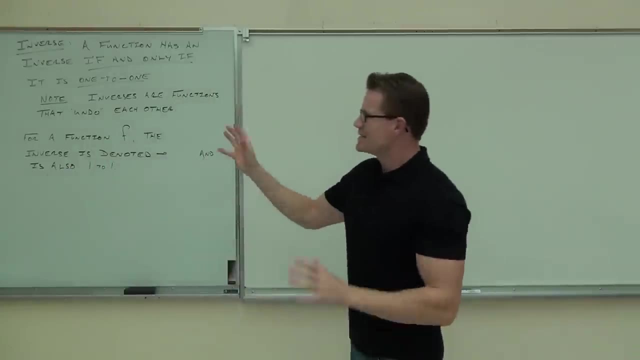 Does that make sense? So it's like undoing everything a function did. That's how an inverse works. It takes operation and undoes it, So it puts everything back to where it was originally. That's this idea of an inverse. It undoes a couple of things. 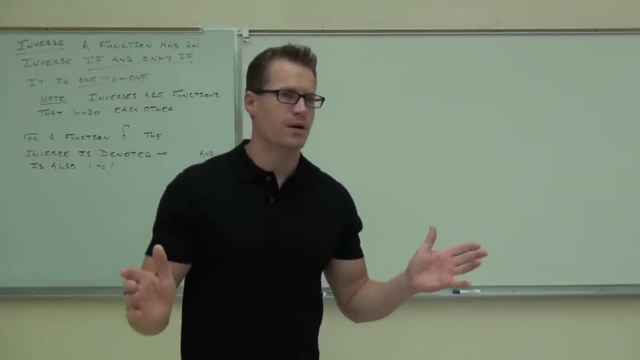 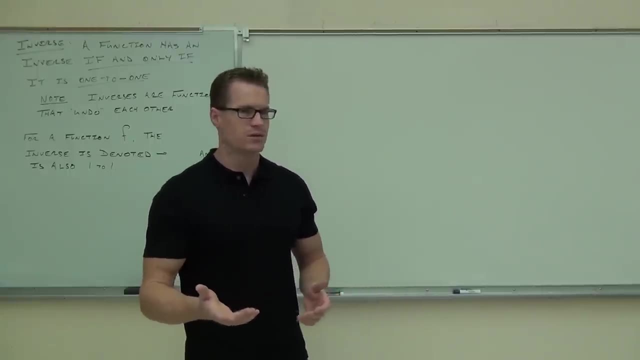 Now we've actually talked about inverses your whole math career. An inverse of addition. What's the inverse of addition? Yeah, it undoes it. What's the inverse of division, Sure, what's the inverse of squaring a number? 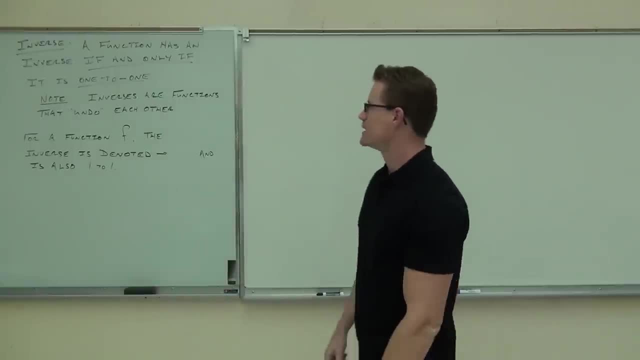 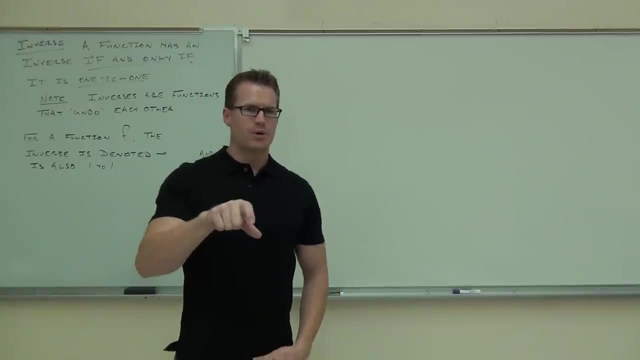 A square root. Yeah, that's the inverse idea. Now, what we learned last time was also something called one to one. One to one meant that if a function has an output, every one of those outputs is unique. So we have all these different outputs. 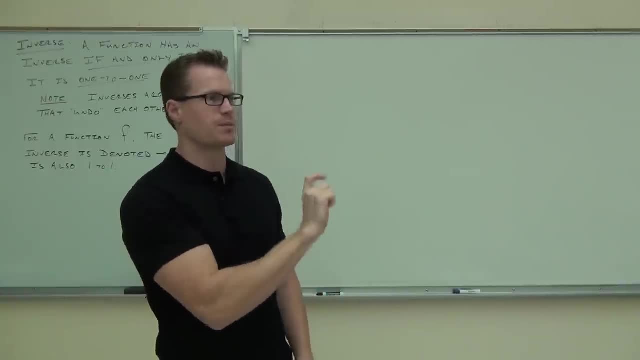 It's going around. If a function is one to one, it means that none of those outputs is ever repeated. So we talked about that last time with the horizontal line test, and that's where we're left off right now. Now, the cool statement is this: 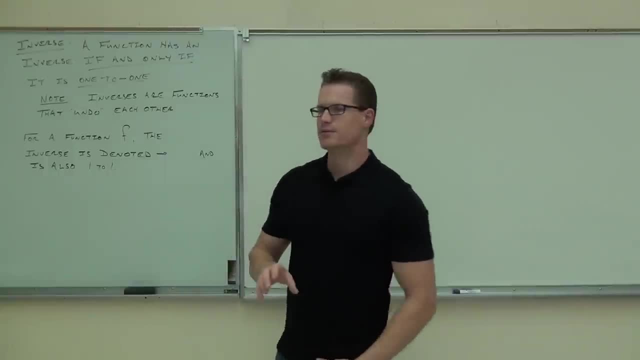 A function has an inverse if, and only if, it's one to one. That's called a biconditional statement. Biconditional means it goes both ways. So a function has an inverse if it's one to one, and automatically if it's one to one. 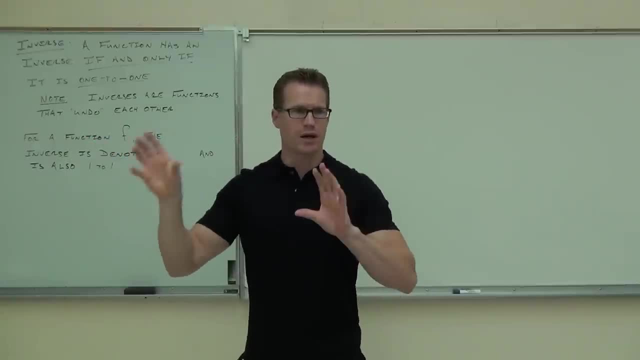 it must have an inverse. Do you see how that works? It goes either way. So if a function has an inverse, it must have an inverse. If it's one to one, it must have an inverse. If a function does have an inverse, it is one to one. 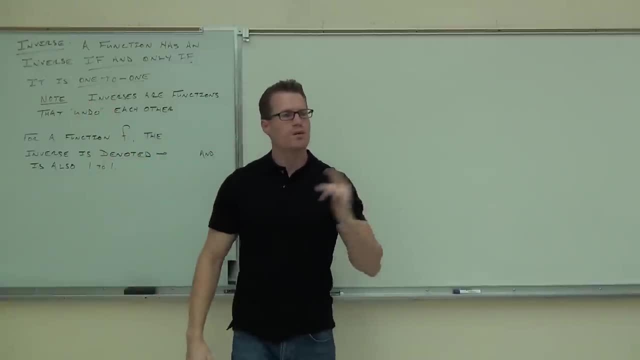 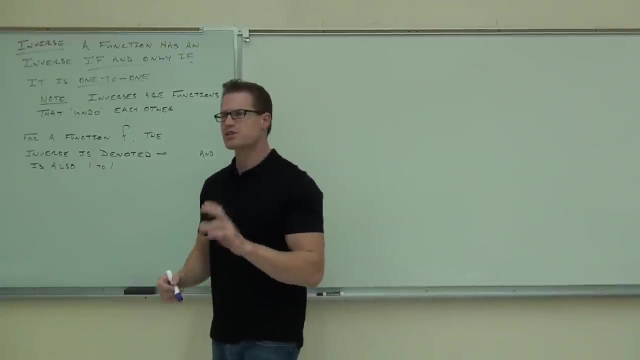 And if it is one to one it must also have an inverse. The way we write an inverse for some function like f, so for a function f the inverse is denoted. we use the same letter, f We use the same letter. 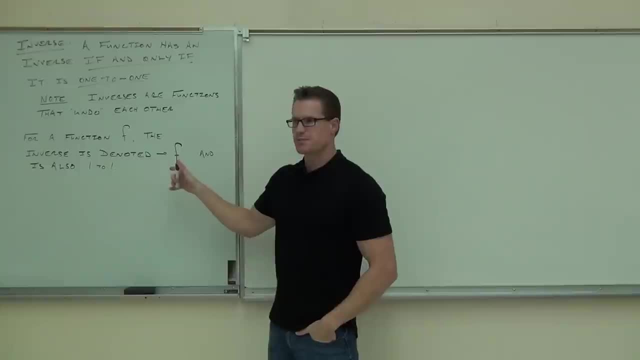 However, if we don't want to call this thing an inverse, here's how you write it. Watch carefully on the board. So for a function f, the inverse is denoted still f, but you've got to show it's an inverse and here's how you do it. 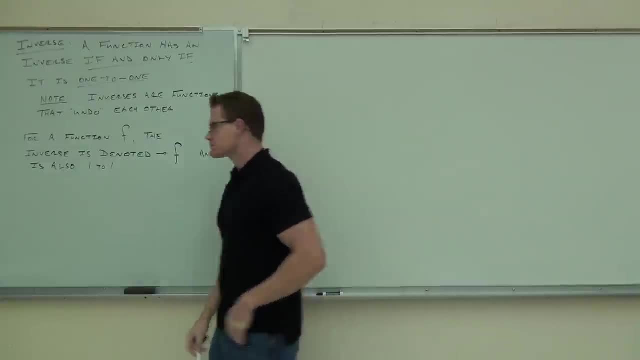 Now please listen carefully. I don't want you to get confused on this. To write an inverse, you say this: There, you put that negative one right there. That's a negative one. You don't say f to the negative one. 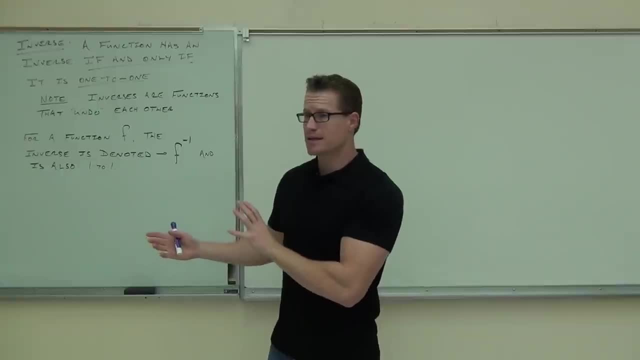 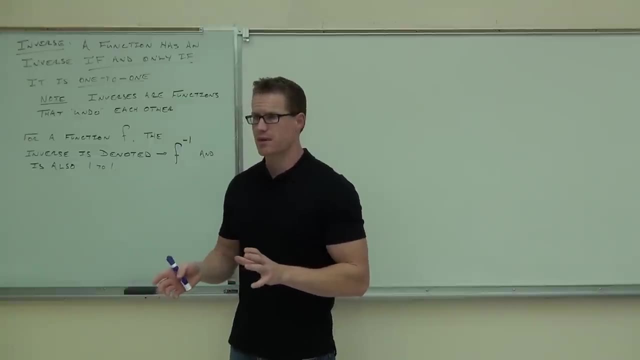 Okay, here's the thing. That is not an exponent. It doesn't mean one over f. That is not what it means. It's simply the only way that we have to put an inverse of a function. Are you with me on that? 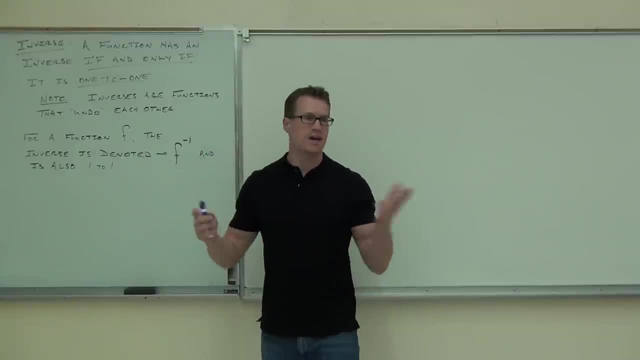 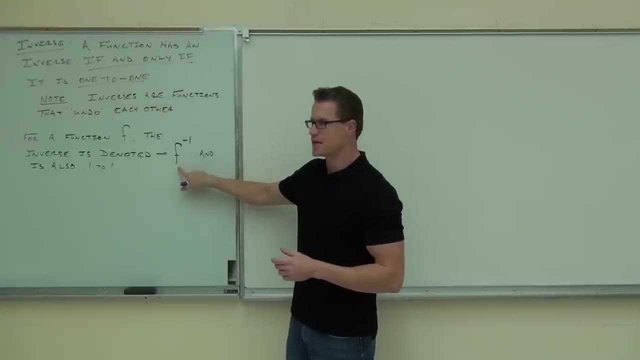 So is this an exponent? No, No, It just it's pronounced f inverse. So let's all say this with me: For a function, f the inverse is denoted. what is that f inverse? f inverse Don't say f negative one. 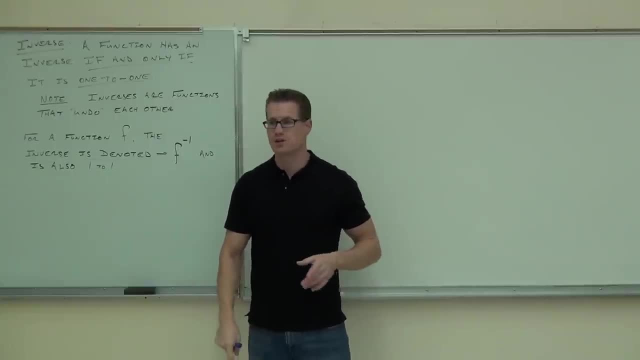 Okay, don't say that That negative one. we're not even calling it negative one. It's called an inverse. So that is f inverse. You're going to be okay with that. And also one thing you need to know is that this thing is also one to one. 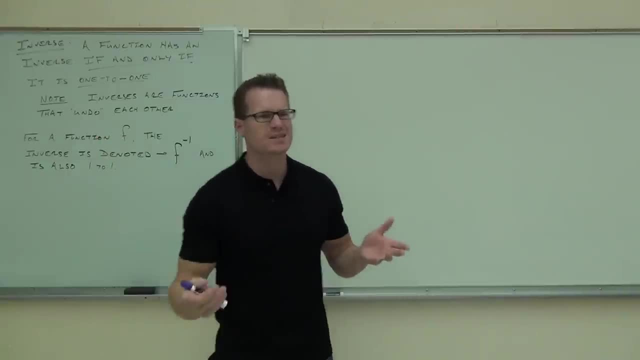 So a function and its inverse will both be one to one. That has to make sense, because they are inverse operations, They're inverse functions, They have to undo each other. So if this function has an inverse, it's this, But then this is also the inverse of that function. 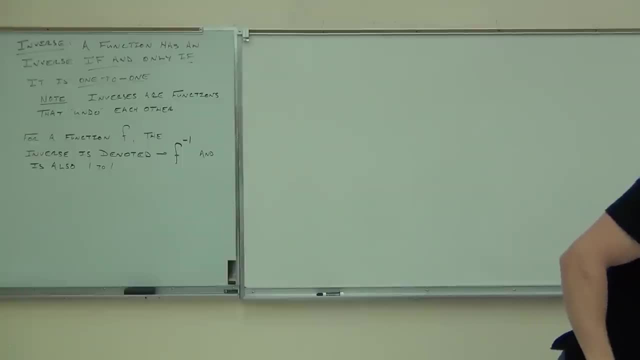 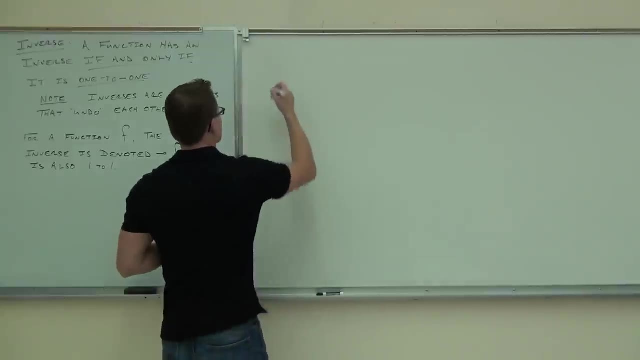 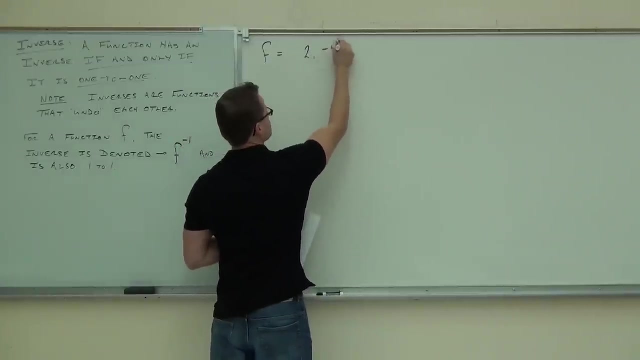 So those two things work together. Now we're going to do a very simple example to illustrate an inverse. Are you guys ready for it? All right, So let's pretend that our function- again function f- has only four points. We need to increase f. 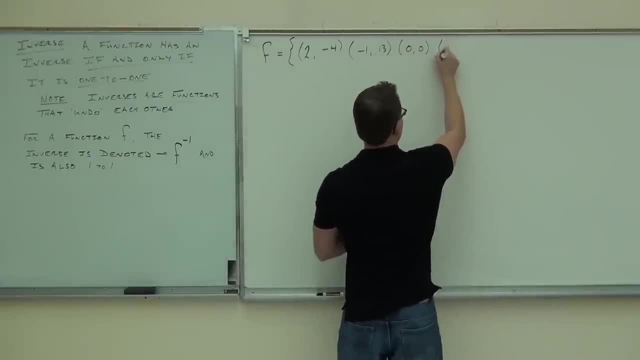 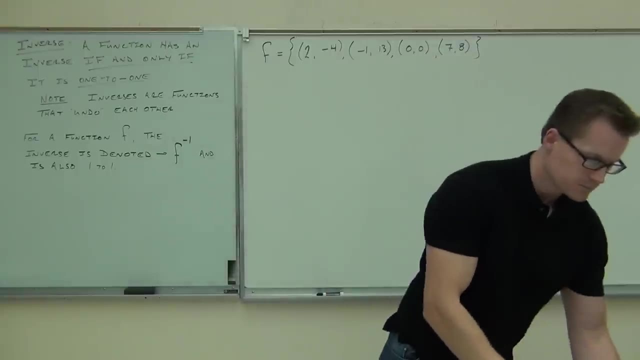 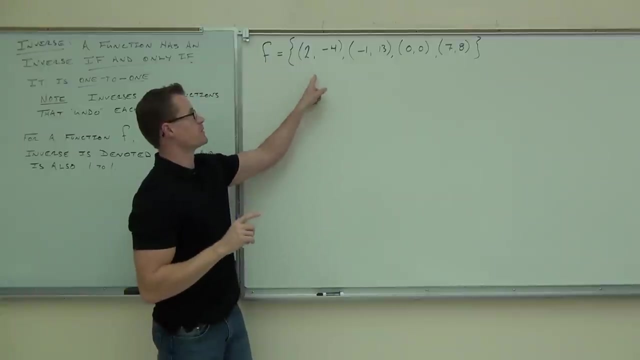 We need to reduce the ability of f to be one to one. We need to reduce the ability of f to be one to one or to get more points. Okay, Watch carefully. I'm going to explain to you how an inverse works. First thing, can you tell me my inputs, please? 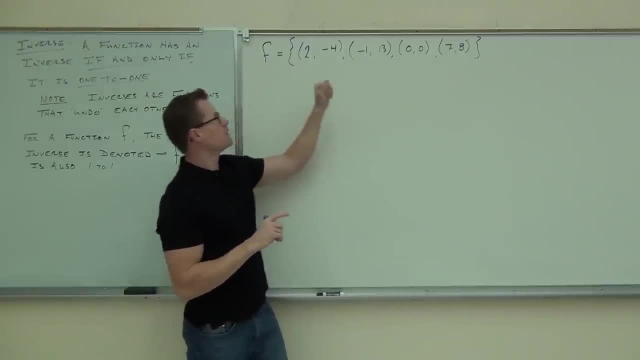 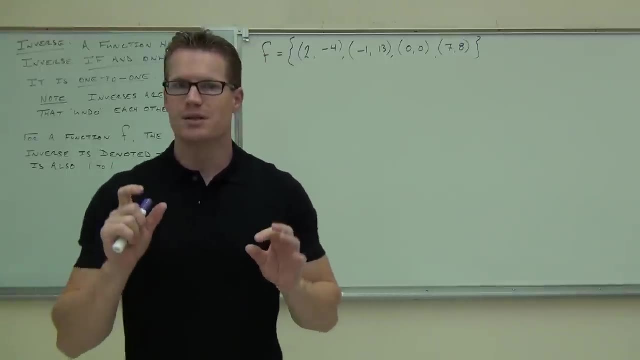 What's my input here? Negative 1 plus zero plus F Outputs Negative 4 times 13.. Zero. Good, Here's what an inverse must do to give you back what you started with. Now pay attention, here's the whole operation of inverse. 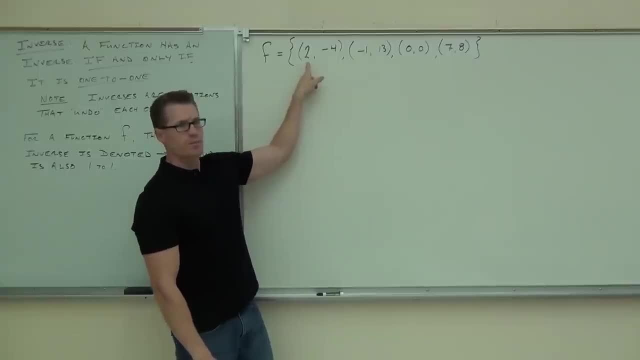 What this function does is this: takes this number, does something to it and gives you out that number. Are you with me on that? So you plug in two, but you get out negative four. You follow, You plug in negative one, you get out 13.. 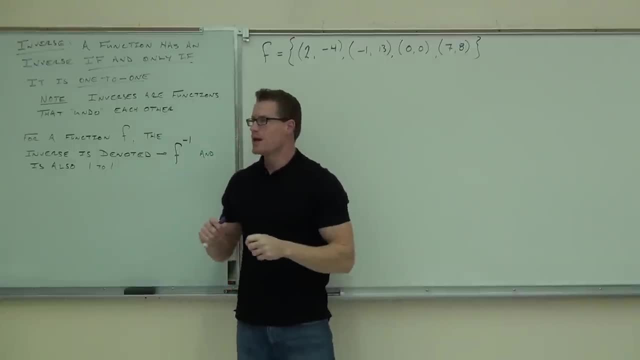 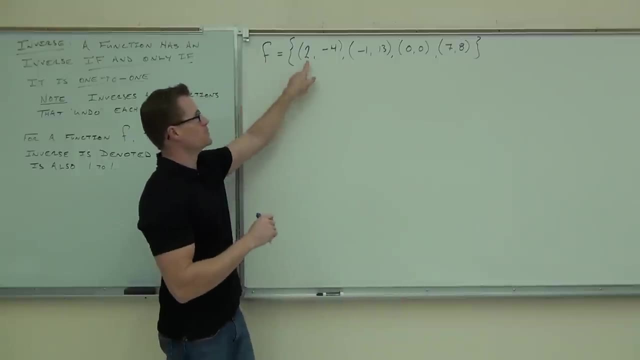 You plug in zero, you get out zero. You plug in seven, you get out eight, And inverse has to undo that. So tell me if I originally plugged in two and it gave me out negative four. think outside the box here. 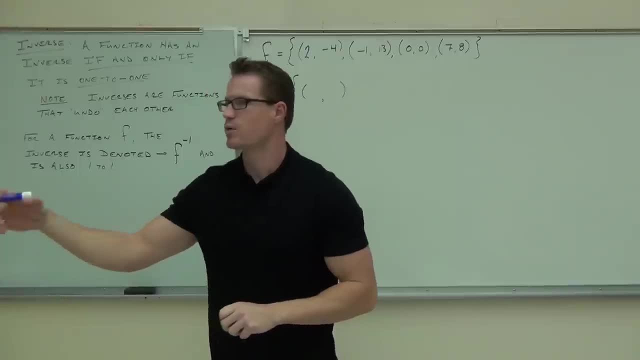 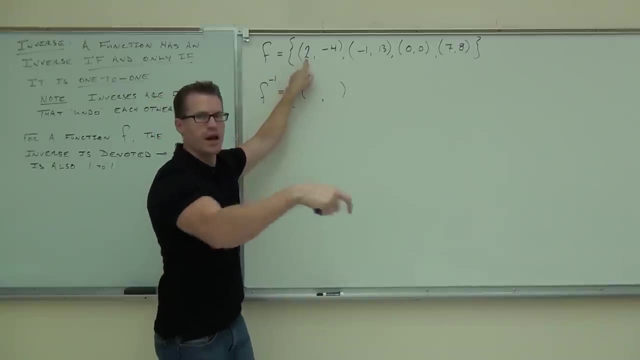 can you tell me what our inverse has to plug in and what it will give me out? I'll give you a hint here. I'll give you a hint If I plug in two. that's what our inverse has to give me out. 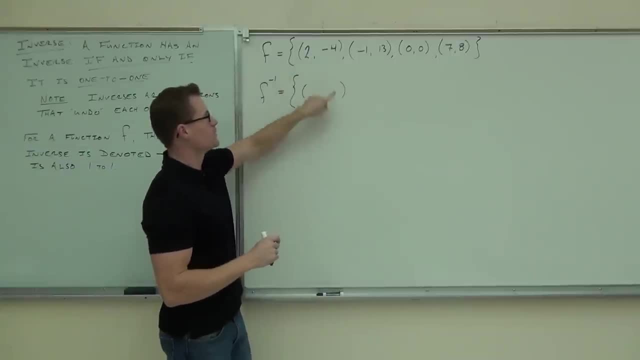 Does that make sense? It's gotta undo everything. So what number has to go here? A two has to go there. What number has to go here? Negative four, Negative four. Here's what an inverse does. Watch, Check it out. 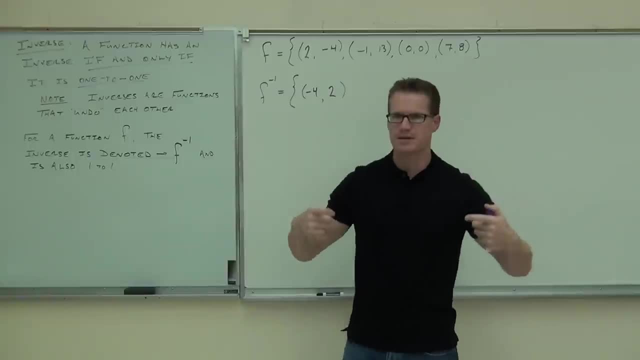 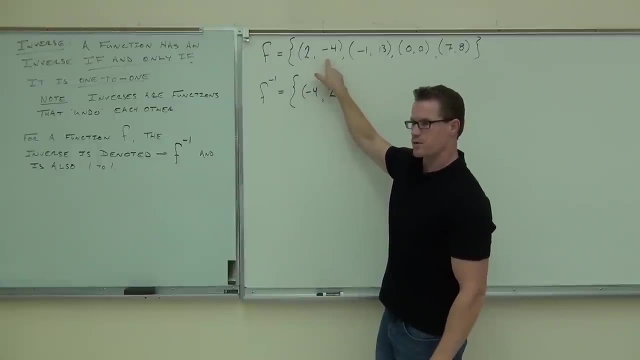 If you're not following that, here's the whole thing. Some of these people were kind of thinking outside the box and get this idea already. but watch if you don't. My original function took the point two and gave me out negative four, correct. 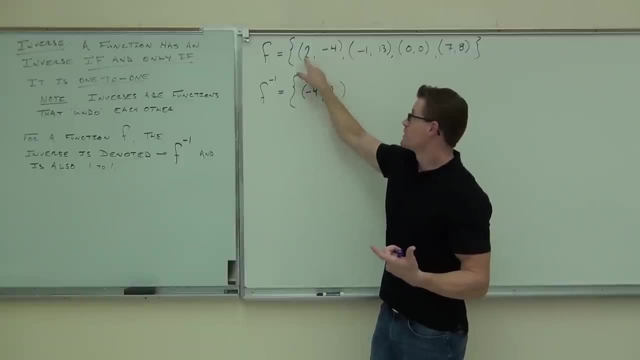 My inverse has to undo that. So it says: well, if you're plugging in two and you're giving me out negative four, my inverse has to undo that. So it says: well, if you're plugging in two and you're giving me out negative four, 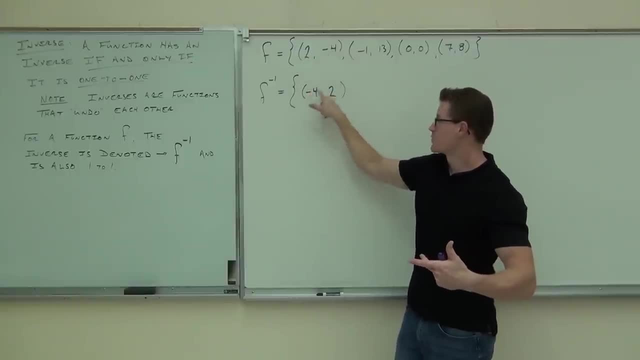 my inverse has to undo that. So it says: well, if you're plugging in two and you're giving me out negative four, I'm gonna take your negative four and give you right back the two. Does that make sense to you? 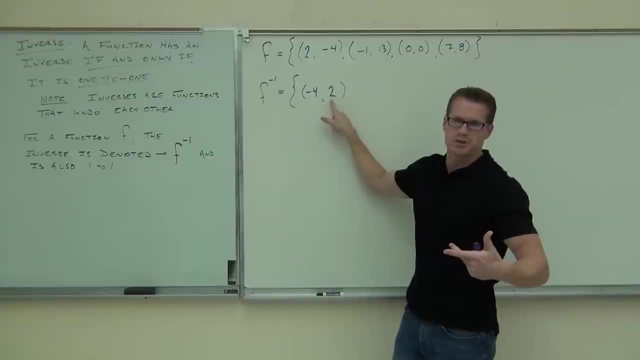 That's what it's doing. It's undoing it. Let's try this next one. This function says: okay, you're plugging in negative one, I'm gonna give you out 13. My inverse has to undo the operation. 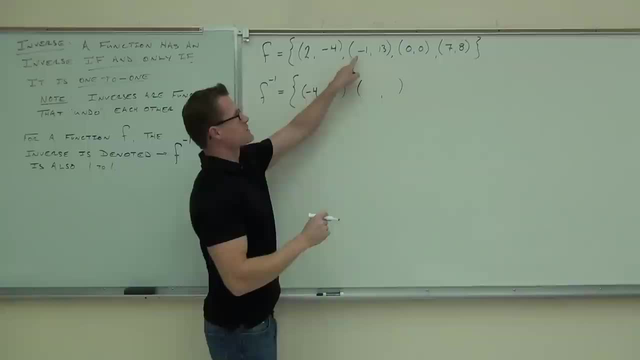 So it's taking my 13, and giving me out how much Negative one. Are you following this? Yeah, Okay, good, Oh, It's taking my 13, and giving me out how much Negative one Are you following this? 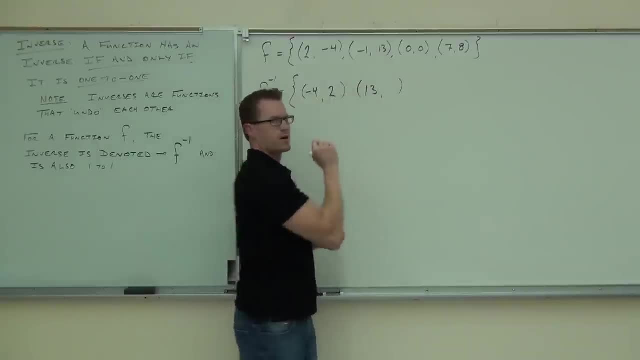 Yeah, Okay, good, Oh, It's taking my 13, and giving me out how much Negative one. Are you following this? Yeah, Okay, good, Oh, It's taking my 13, and giving me out how much. 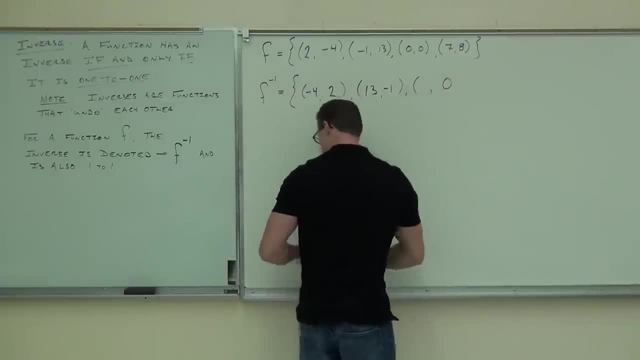 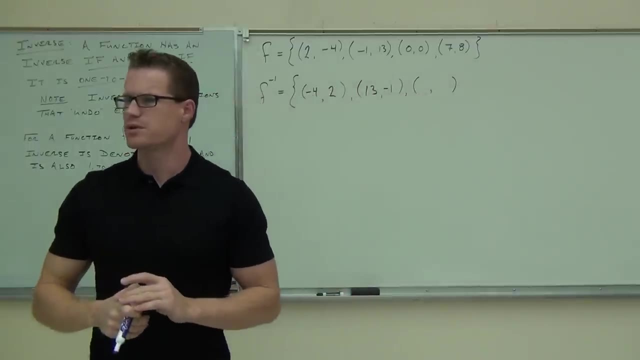 Negative one. Are you following this? Yeah, Okay, good, Oh, Why? Oops, How about the next one? Can you figure out what the next one's gonna be? My original function takes zero and gives me out zero. What's the inverse gonna do? 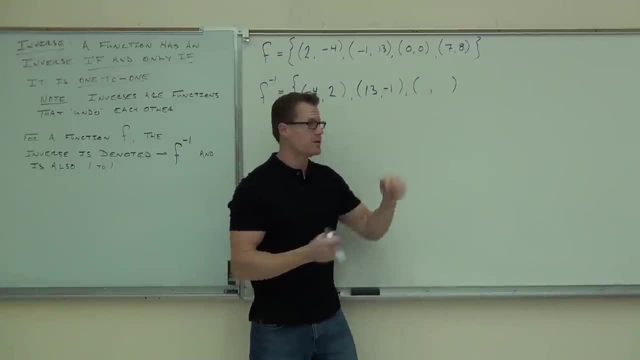 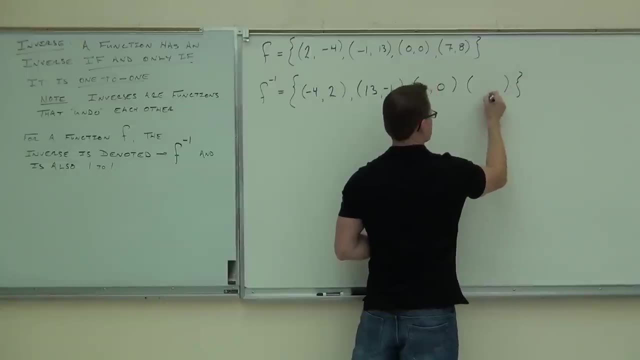 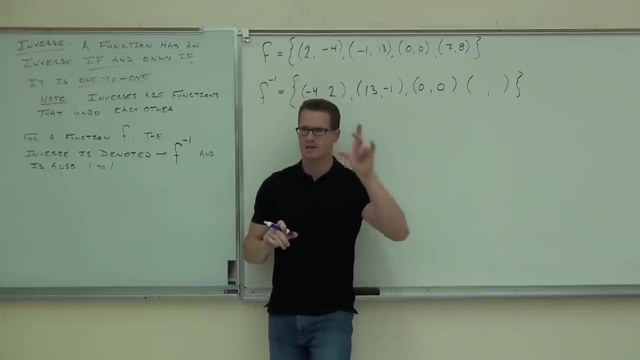 Zero, Zero, Yeah, That one doesn't change at all, right, Yeah, Yeah, Yeah, Yeah, Yeah. Yeah, You did it all right. And last one: My original function gave me 7.. I'm sorry, You plugged in 7 and gave me 8.. 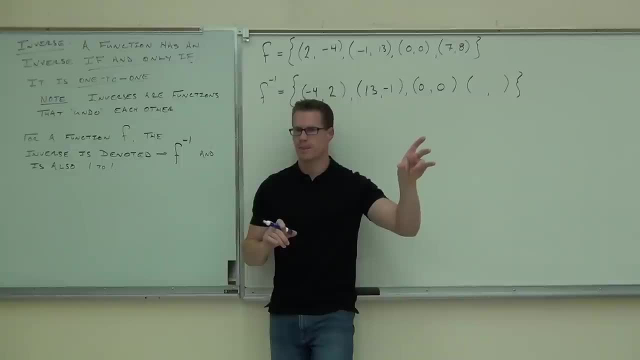 What's the inverse gonna do there? Can you guys figure that one out? It says it: he Yeah. it says: well, I'm gonna take the 8 that you gave me out and I'm gonna give you back the 7.. 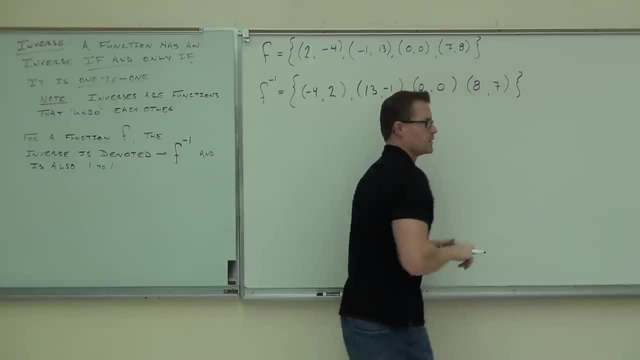 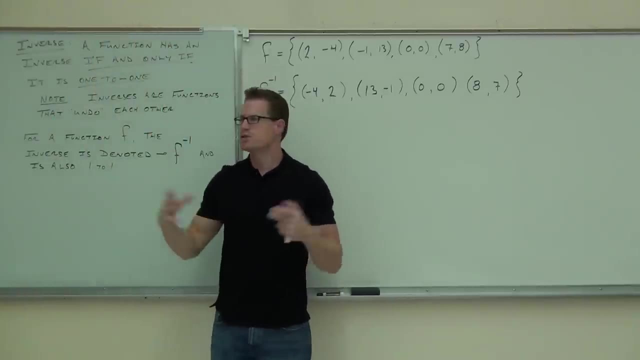 It's undoing that whole operation. So basically, what your inverse does is it gives you back what you started with. How many of you understood this idea? So how would you say in English for someone who really doesn't understand the inverse: 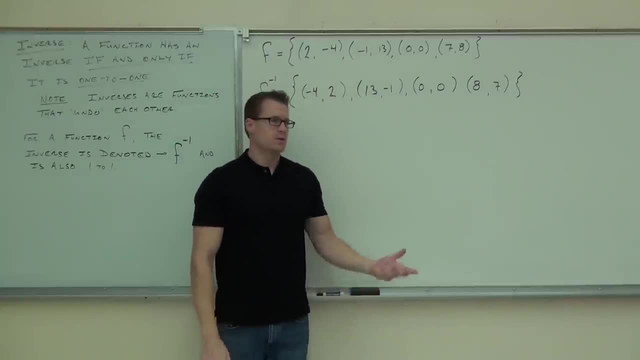 what are you doing from here to here? What are you doing? You're going backwards. sure, you're finding the inverse, But what are you actually doing? point by point, You're switching. Switching what? What are the inputs and outputs? as far as the coordinates? 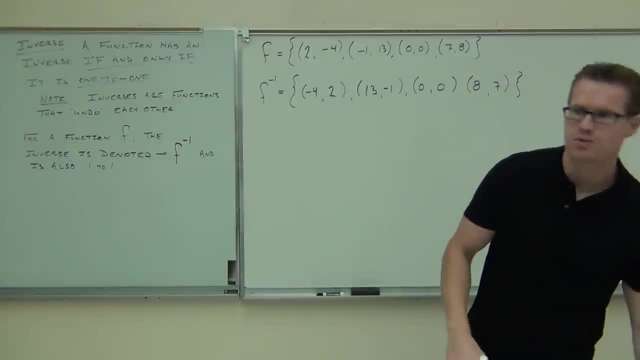 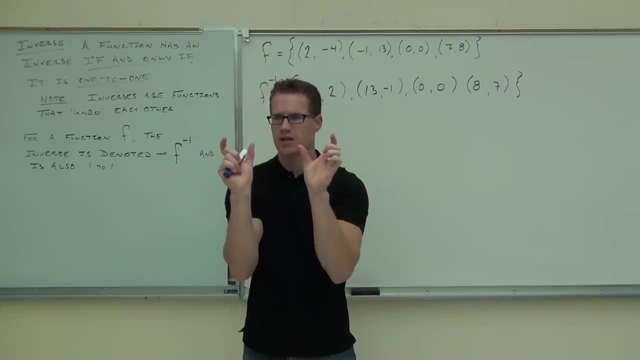 You're switching x and y. That's what you're doing. That's what the inverse does. It switches x and y. It says: well, think about it guys. Think about it. If you're trying to get out what you plugged in, all you've got to do is switch your x and y. 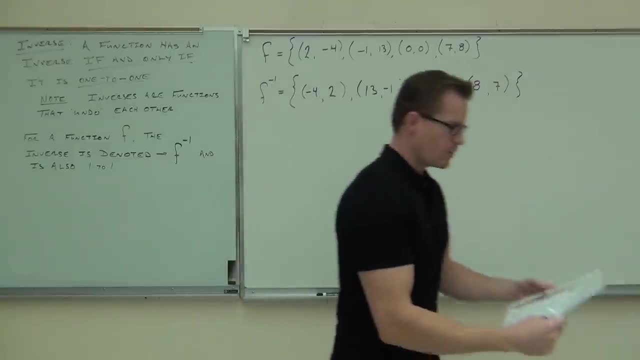 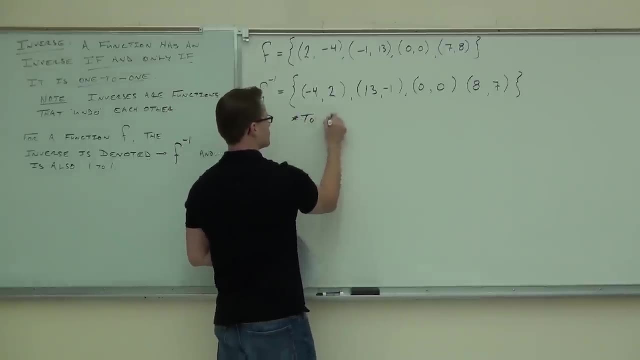 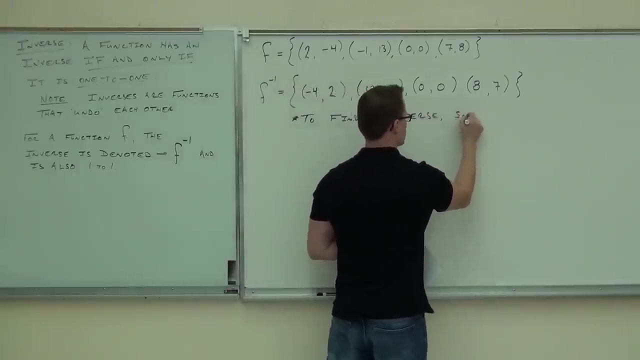 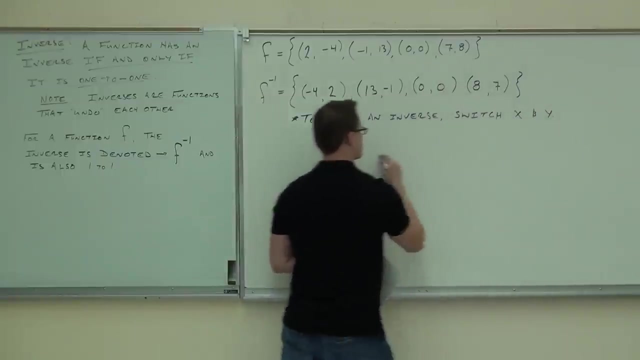 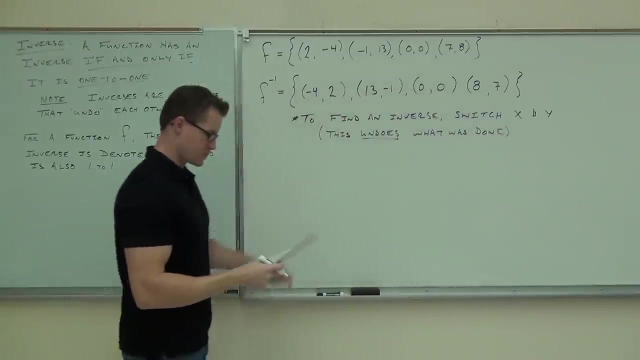 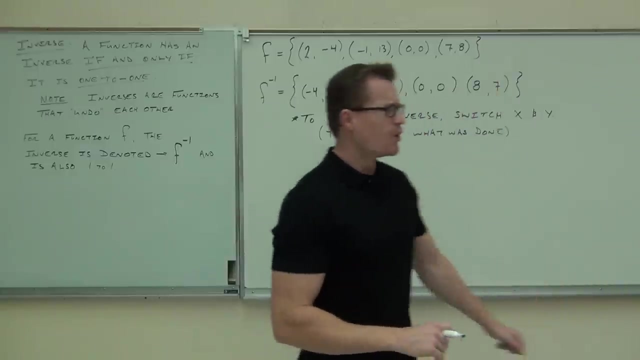 That's switching inputs and outputs. So to find an inverse, we just switch x and y. This undoes what was done. It's as simple as that. Now, the problem is, we normally don't see functions like this, do we? 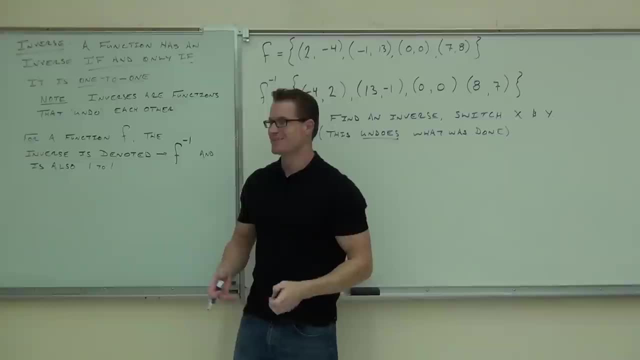 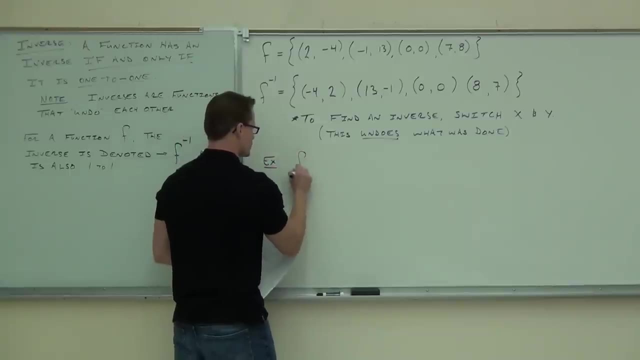 We normally don't see that. We don't see. oh, here's your four points. Do something with that function. We don't see that. How we normally see functions is something like this: We see: f of x equals some sort of an equation here. 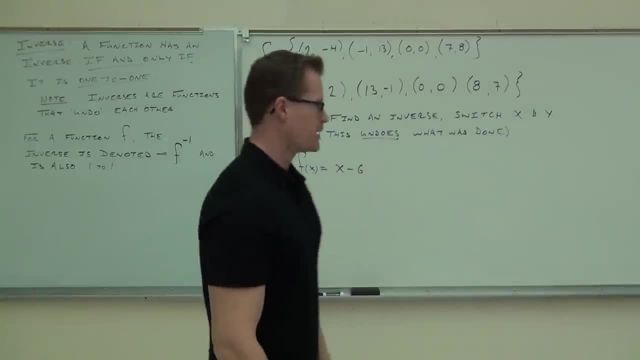 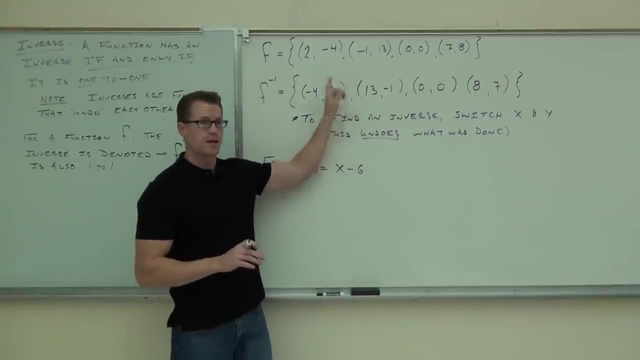 That's typically how we see functions. Is there a way we can find the inverse for this thing? Well, I'm going to say to you that it's going to be really, really similar to this idea. In this idea- were you with me- that all you've got to do is switch your x and y? 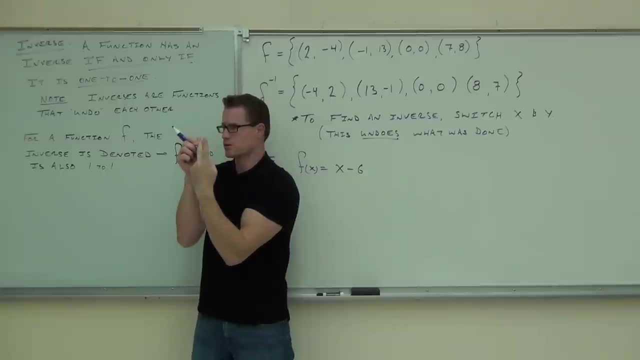 Because it's taking what you got out and making it what your, what you're plugging in right. That's what it's doing. It's going to give you back your original. We can do the same thing here. Here's your steps. 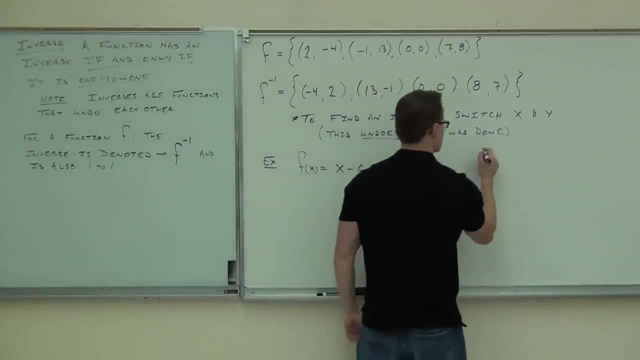 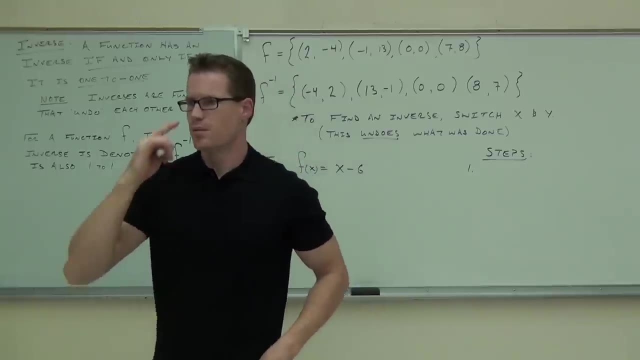 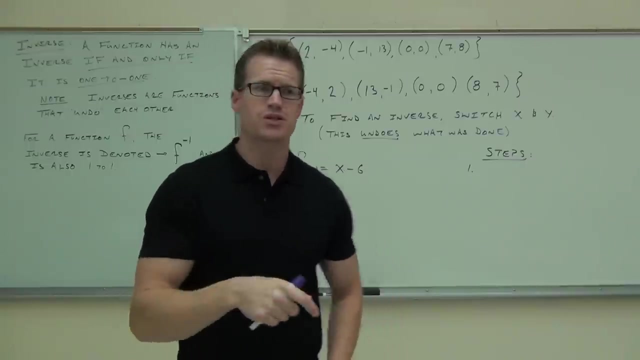 There's only- let's see, there's four steps, but they're very, very easy steps. Number one, number one: the act of finding an inverse really comes down to: can you switch x and y? The problem is, do I have a y up here right now? 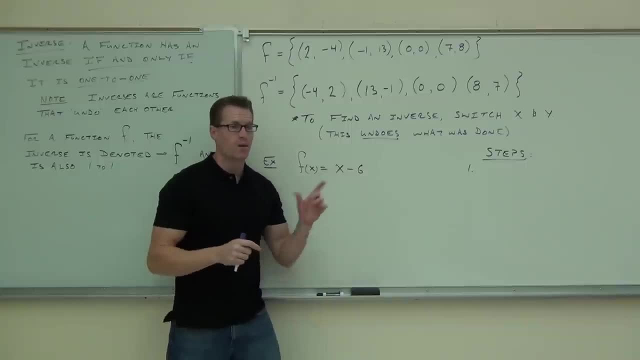 Yes, I don't see a y. However, some of you are saying yeah, because you probably understand that one of these things stands for y. What up here stands for y. So instead of f of x or g of x or whatever your function is, write that as y. 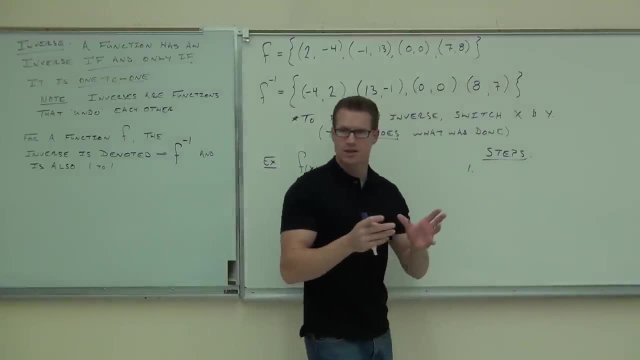 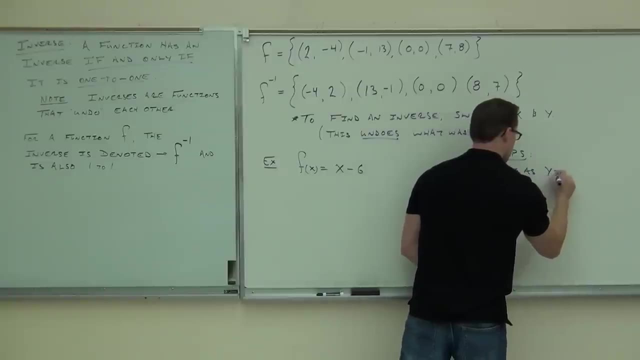 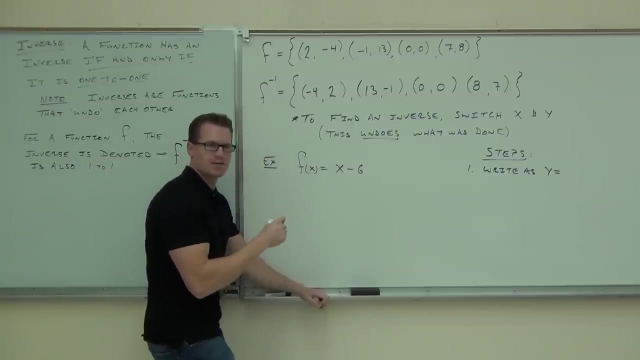 That's your very first step. So write as y equals instead of f of x equals, or g of x equals. Write as y equals. So up here on the board: instead of f of x equals x minus 6,. what am I going to have, ladies and gentlemen, please? 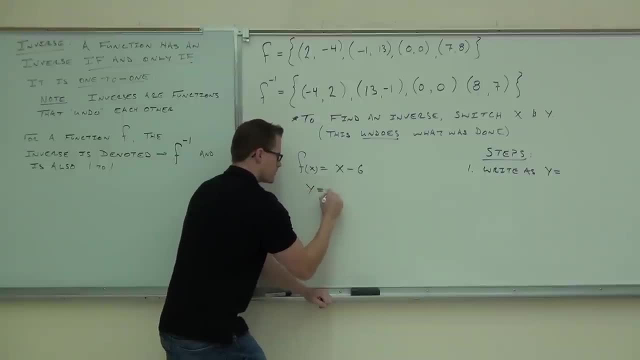 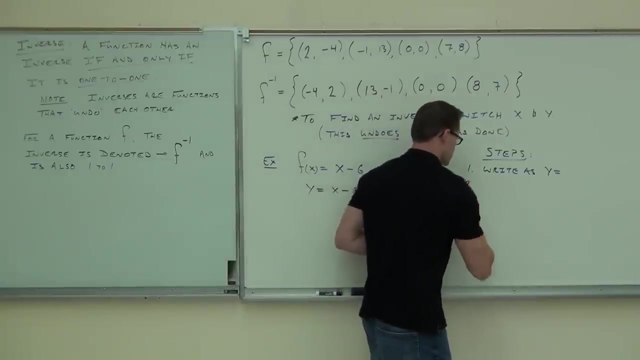 Yeah, that's all I'm doing. I'm switching my f of x with my y. You okay with that so far? Okay, Now the next step. next step says: now you're going to go through the action of finding an inverse. 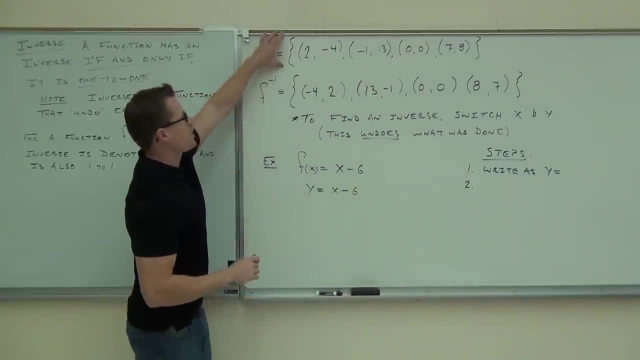 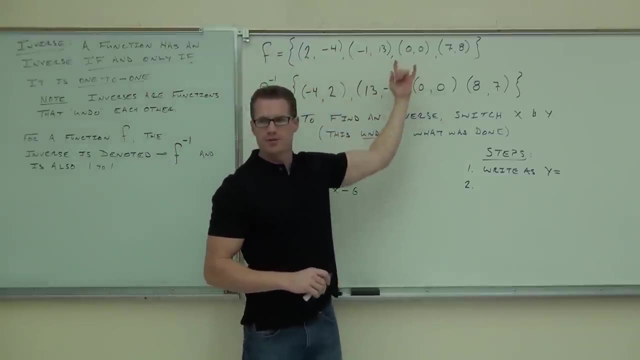 Watch carefully what I'm going to do up here. all right, To go between this problem, this function and my inverse, I had to switch my x and my y. Are you with me? I had to switch my x and my. I did that for every single point. 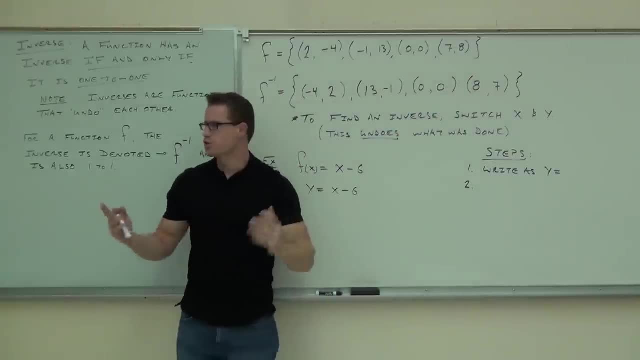 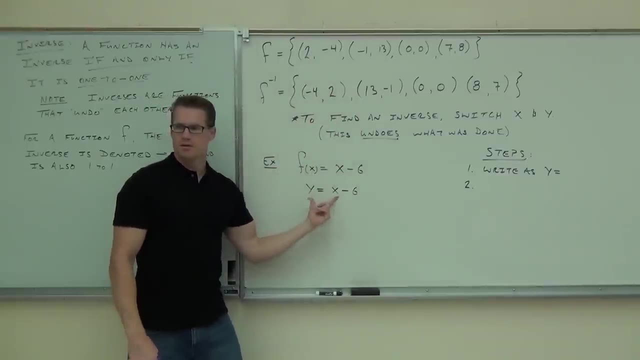 How can we do that for every single point in general in a function? Well, you're going to do exactly the same thing. If finding an inverse means I'm switching my x and my y, what do I have to do here? That's going to do that for every potential point that I ever get. 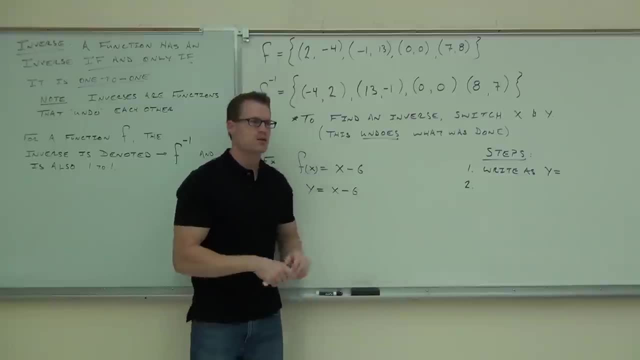 Are you with me on that? It's going to switch my x and y forever, So what I'm going to do is: you're not moving anything around. Where do you see a y, what are you now going to put? And where you see an x, what are you now going to put? 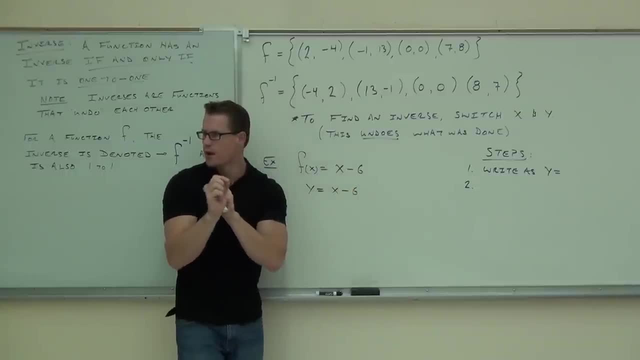 Y. That's switching your x and your y. You're making your y's x's and your x's y's. Now do you have your okay on that one? That's how you find an inverse. That's what we did here. 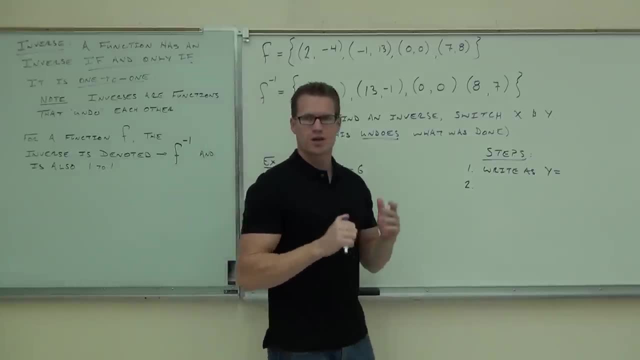 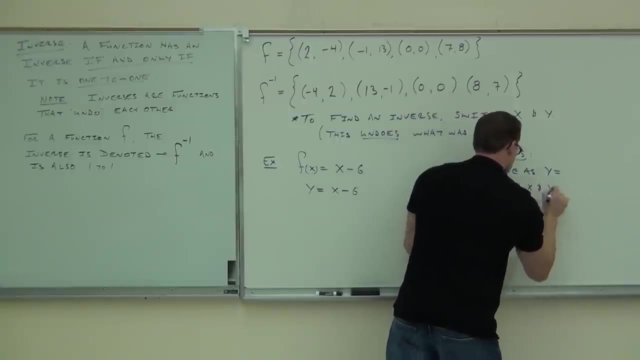 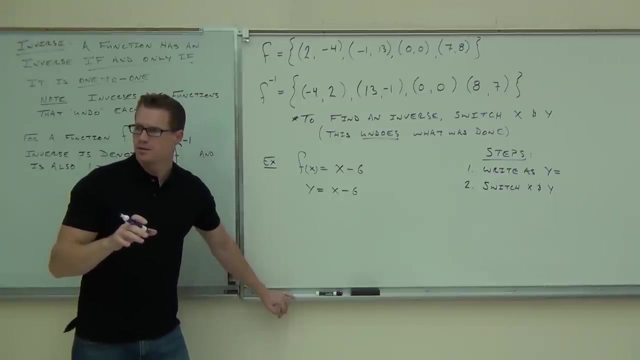 That's what we're going to do up here as well. So step number two: you're going to switch x and y. Can somebody up there read me what I should have down on my paper? please Say that louder. Good, Good. 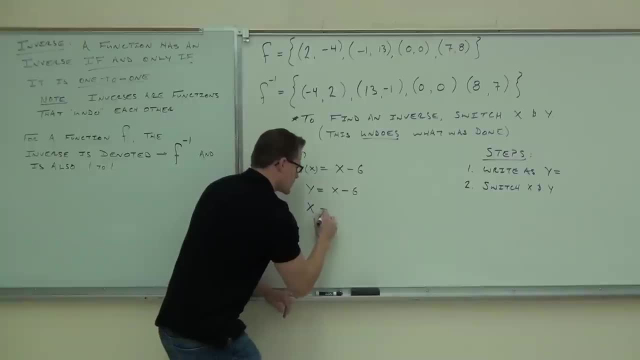 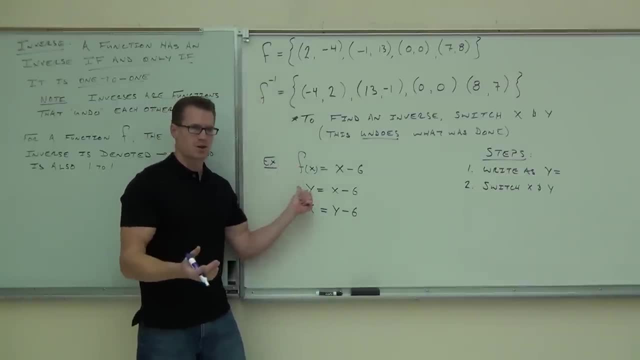 things here. One f of x becomes y. That's how we have to get started, because we're going to switch our x and our y. We add: I have y somewhere. Then we switch these two things. We say, oh, y's now become x's. 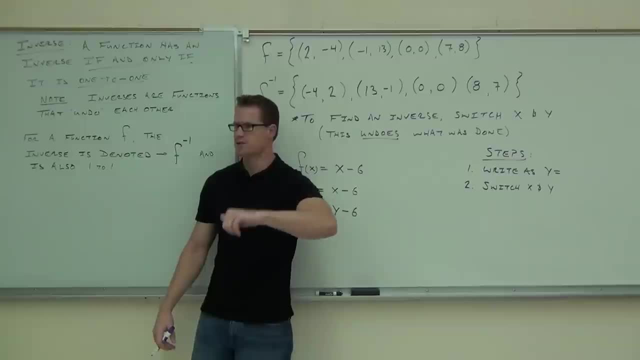 X's now become y's. So instead of x's, you write y's, Instead of y's, you write x's. X is not as good, if you're okay with that. Okay, Well, what? now We're almost done. 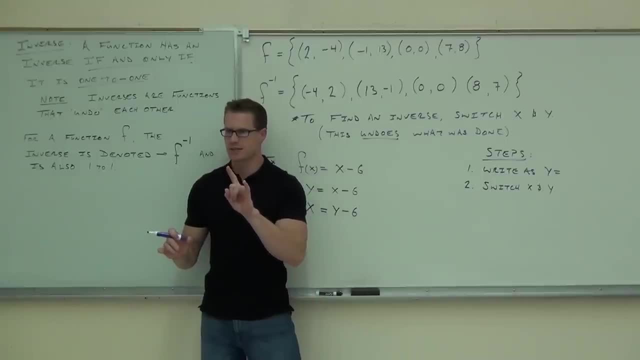 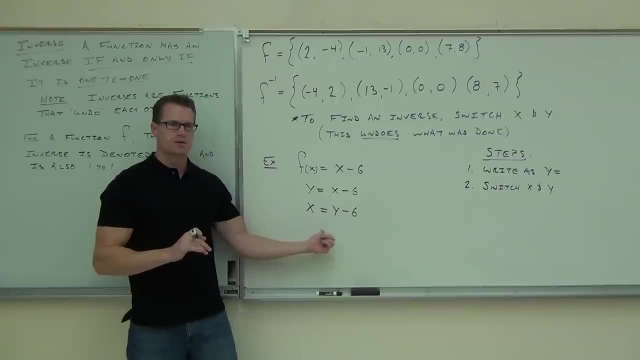 We're almost done. We have two little steps left. The first one takes a little bit more work than the second one. The third one takes more work than the fourth one. Can you solve that for? y? Yeah, that's what you're going to do now. 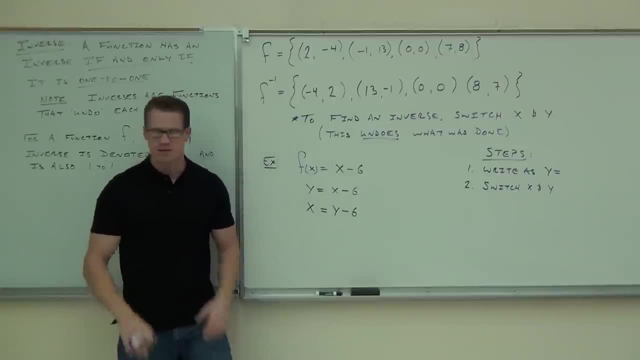 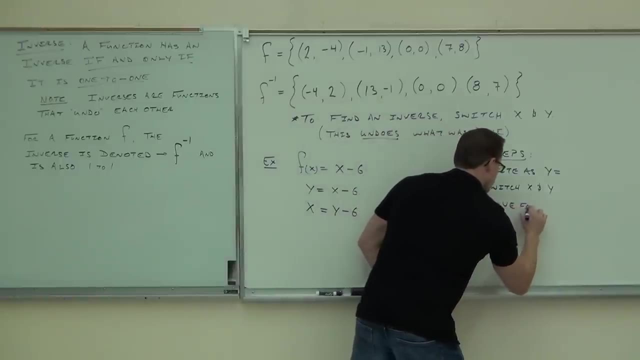 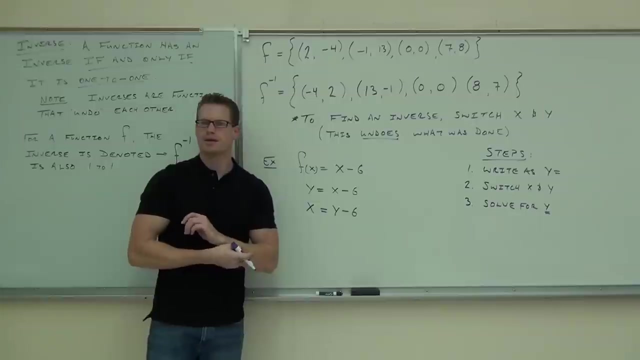 So solve that thing for y. It shouldn't be very hard. You shouldn't have a whole lot of steps there. So step number three you're going to solve for y. How do you solve this problem for y? ladies and gentlemen, 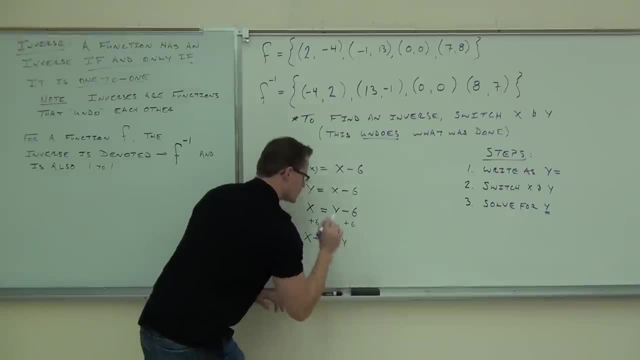 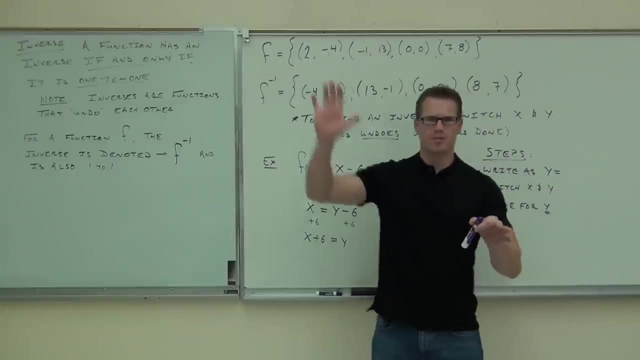 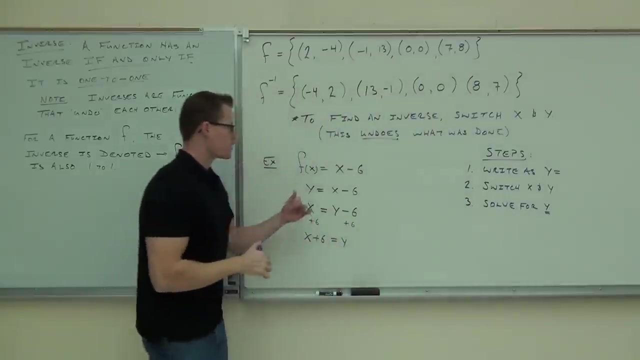 So I'm going to get x plus 6 equals y. Okay, I want to show again how many people are with me on this. so far, Good, I have a few people, not. Yes, no, Yeah, Okay. So what we're doing? we're writing our f of x as a y. 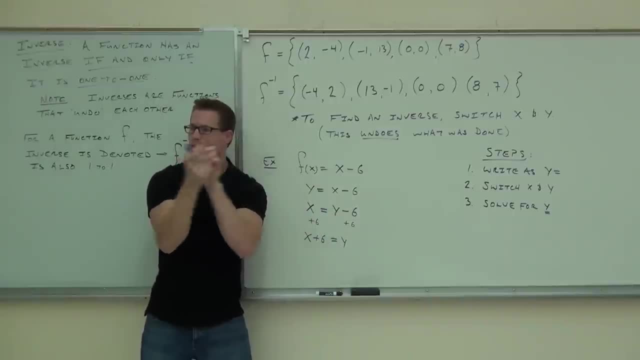 No problem. The whole idea behind an inverse is: you're going to switch x and y, because what you're plugging in now becomes what you're getting out. That's the whole idea. So our x's become y's, Our y's become x's. 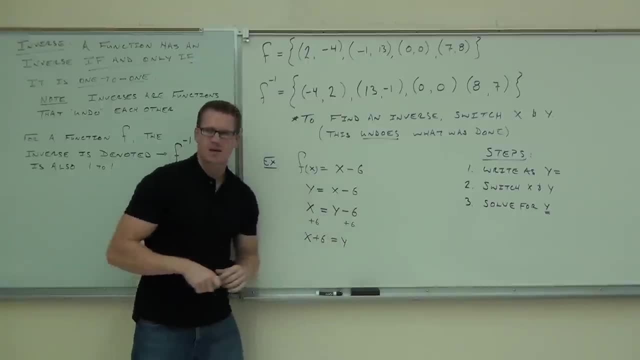 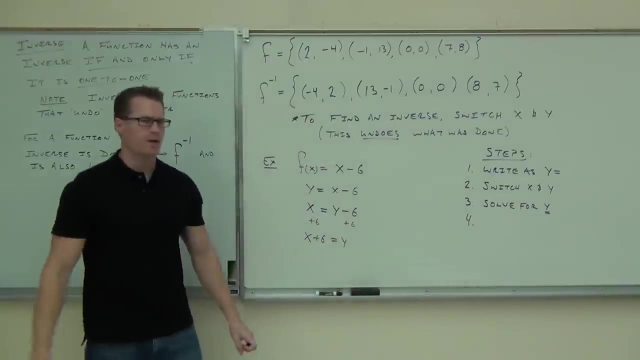 Then we're going to solve for y And the last step. the last step's an easy step because you're done. You actually have your inverse on the board right now. Here's the idea: You're going to write your y back as your function's name. 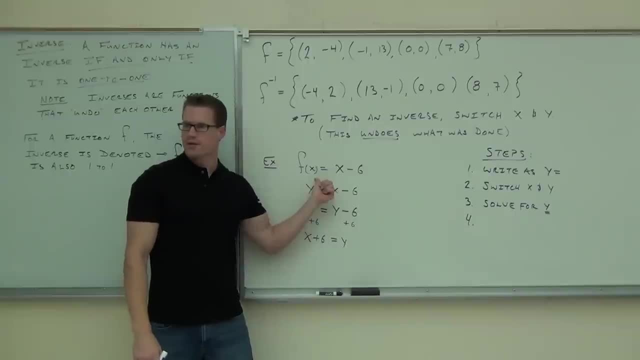 So my function was the function f. yeah, I want to write this as an inverse, Inverse function of f. So this is f inverse. I just have to write that. So I'm going to replace my y with f inverse, with that inverse. 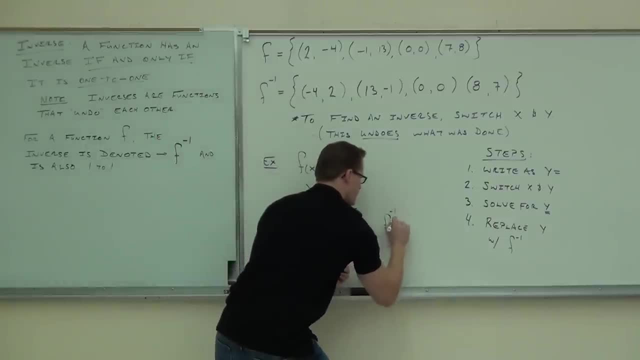 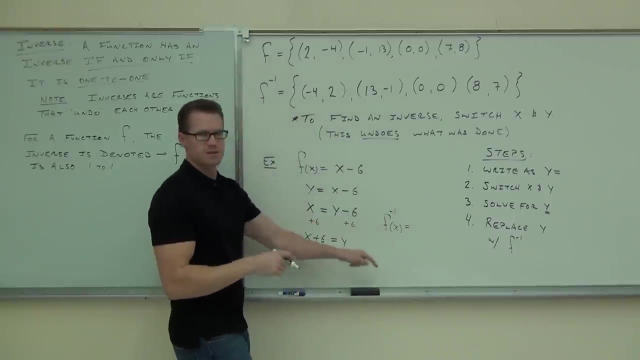 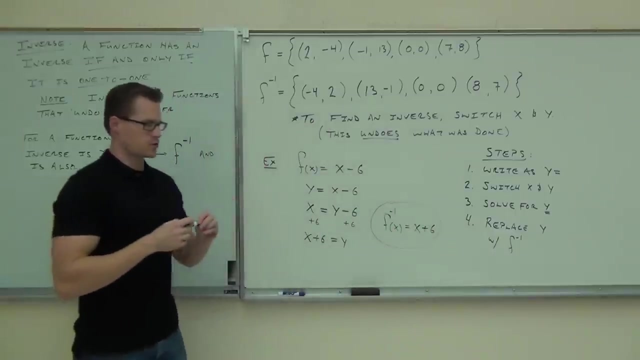 So instead of y I now have f, inverse of x. You've got to have the x there to tell me what your variable is. equals x plus 6.. That's my inverse function. Raise your hand, if you feel okay with how to get that thing. 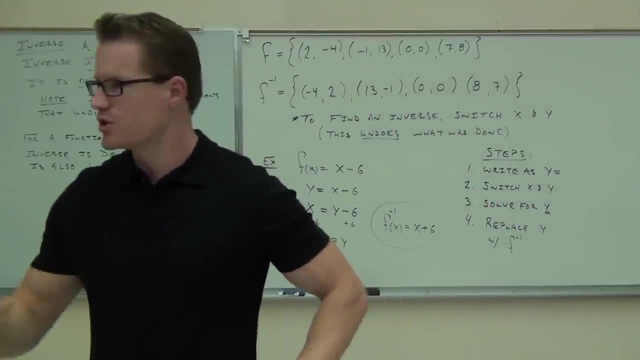 Now, do you want to see why it works? Do you want to see why it works so that it would do this every single time that it's going to do this for you? Check it out. Give me a number between 1 and 5.. 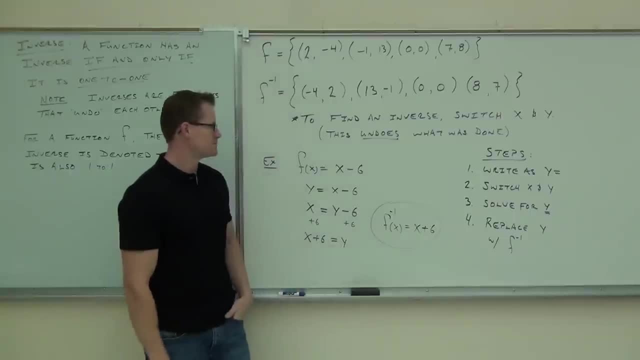 3. 3. Okay, I like 3.. I want you to do this for me. Plug in 3 here. What do you get out of it? You plug in 3.. You get negative 3, are you with me? 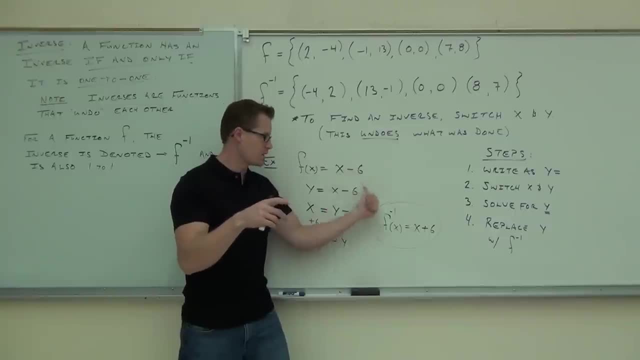 Take the negative 3.. I hope you're all with me on this. Take the negative 3, plug it into here. What's negative 3 plus 6?? Isn't that what you plugged in originally? Do that with any number. 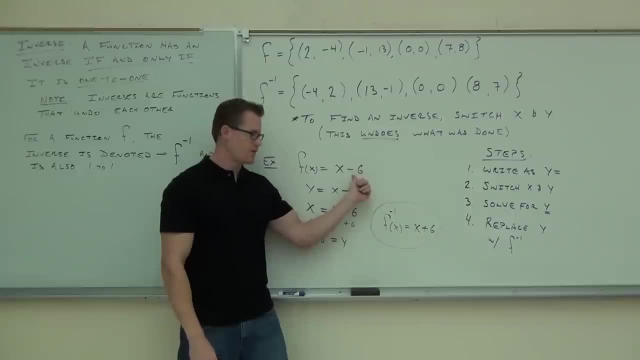 Take 10, if you want. What's 10 minus 6? 4.. If I plug in 4, it should give me out 10.. It has to do that. That's the inverse. Plug in 4.. What does it give you out? 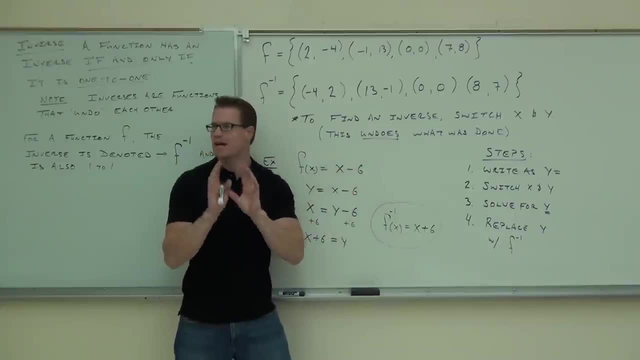 Do you see how it's undoing the whole operation of this function? It's undoing everything you started with. It's giving back what you started with. That's the idea of finding an inverse. It's not hard to do. It's not hard to do. 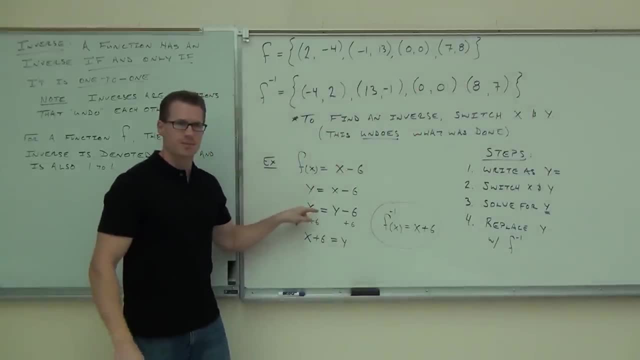 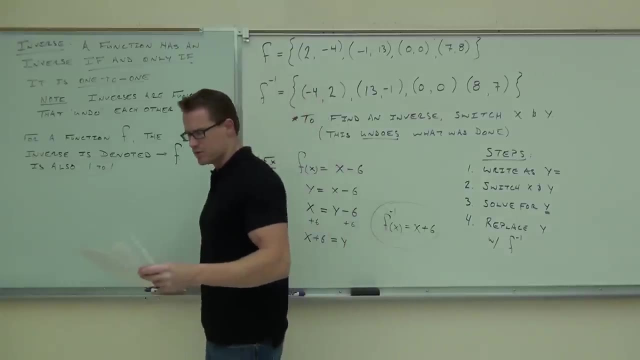 You replace it with y, You switch your variables- That's the key step. You solve for your y and then you replace that with your f inverse. Let's do a couple more examples. I'll give you one of your own. Talk about two more of them and we'll show you graphically. 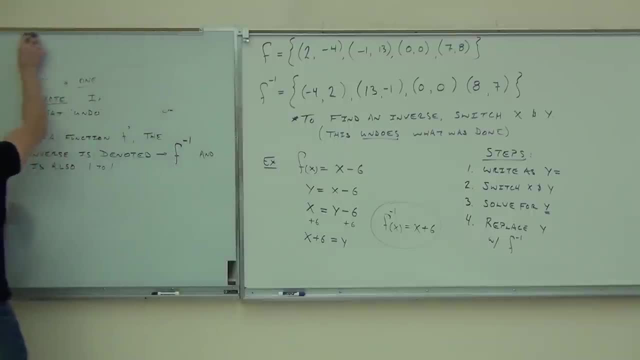 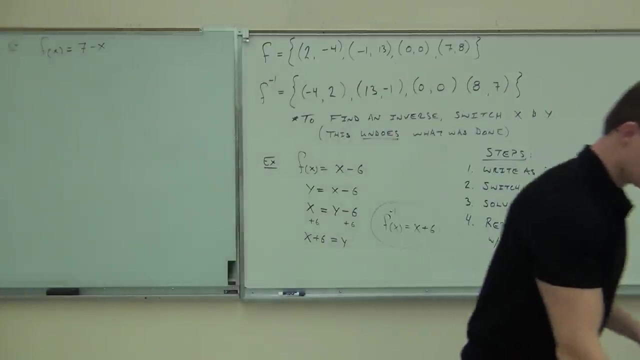 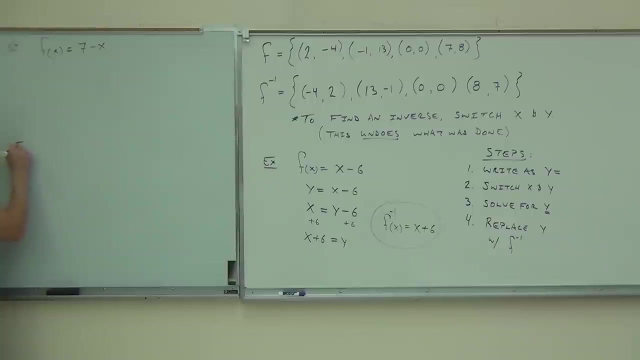 what these inverses are doing too. Find the inverse for me. There you go. Find the inverse for me. If you're feeling like a rock star and you do that one really quick, why don't you try the next one? It's not any harder. 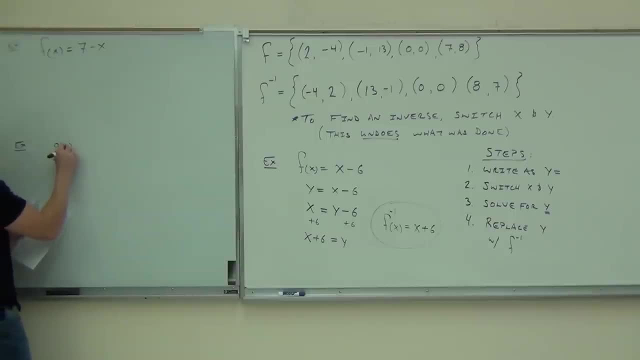 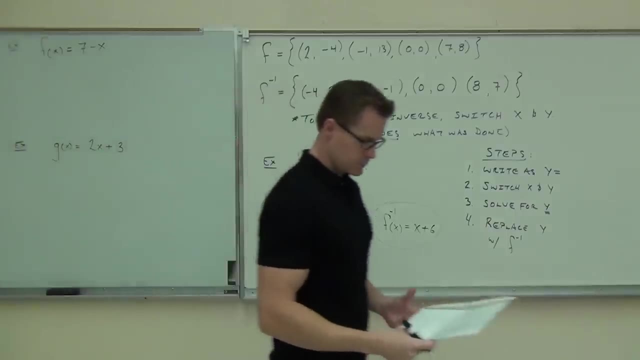 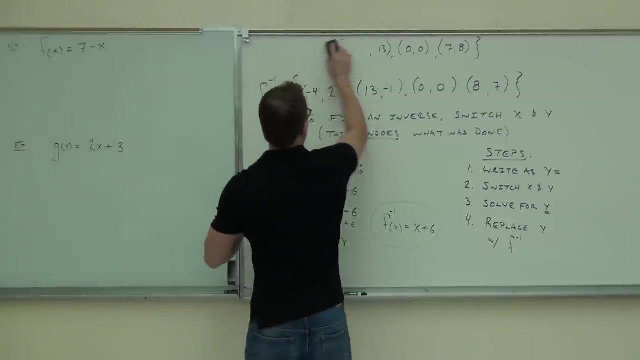 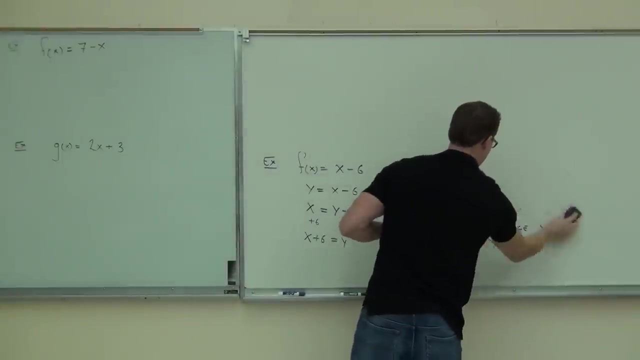 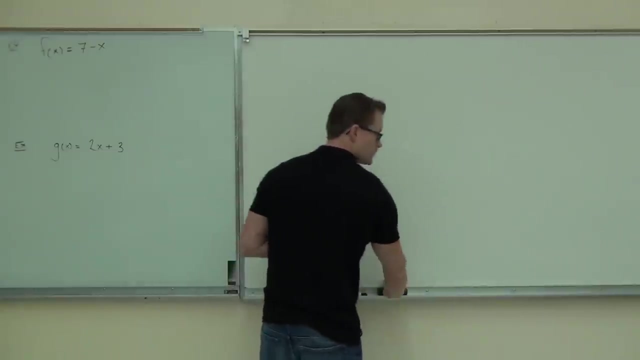 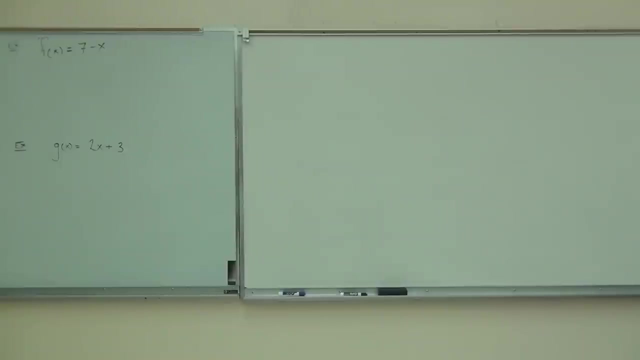 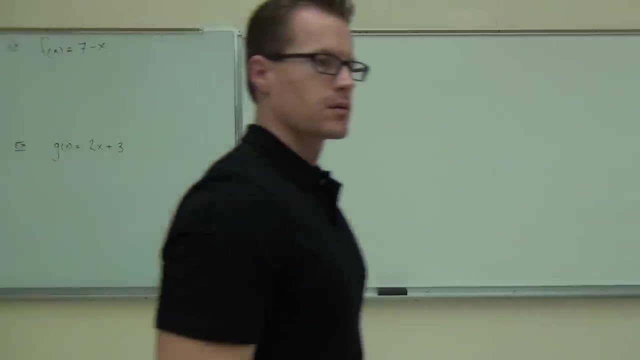 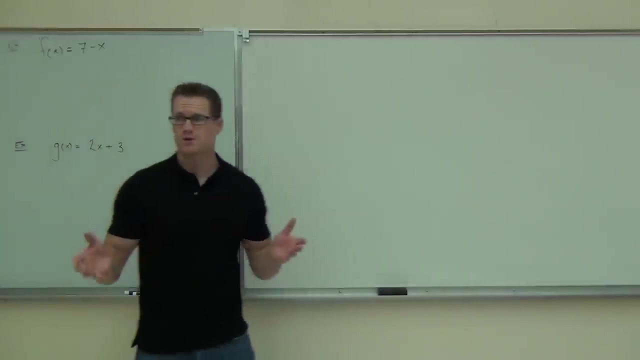 But we're going to do this one together in just a bit. There you go There. If these are� All right, It's OK, Well done, Thank you, Thank you. So let's see here. So first example: well, we know that finding an inverse means somehow we're going to be switching our x with our y, right? 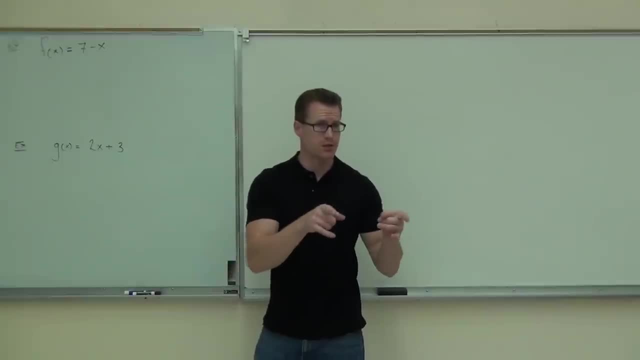 So we're going to have to have a y up there. So the first thing you do- hopefully the first thing you did- is replace your f of x- whatever your function is- with a y. Did you all do that? 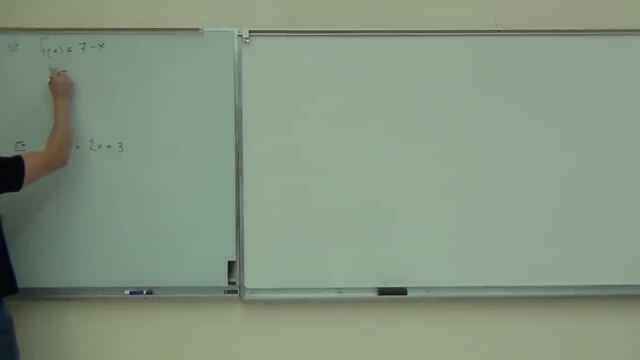 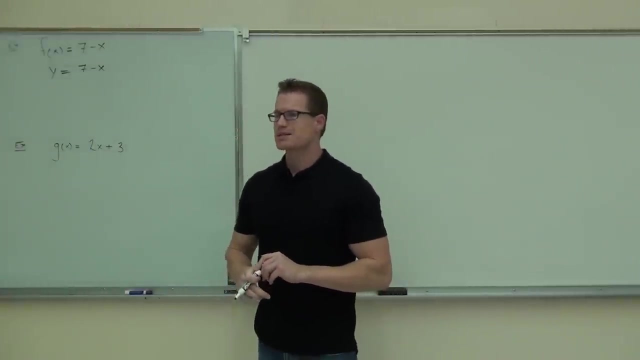 Good. So here we're going to go. okay. well, now we're going to have y equals 7 minus x. Just a little change there: Instead of f of x, you put y. Yes, no. Next thing is the most important thing. 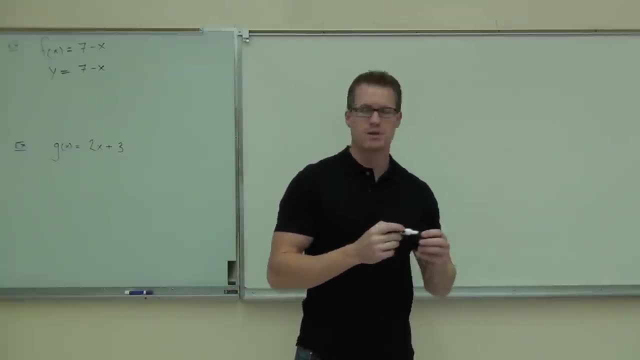 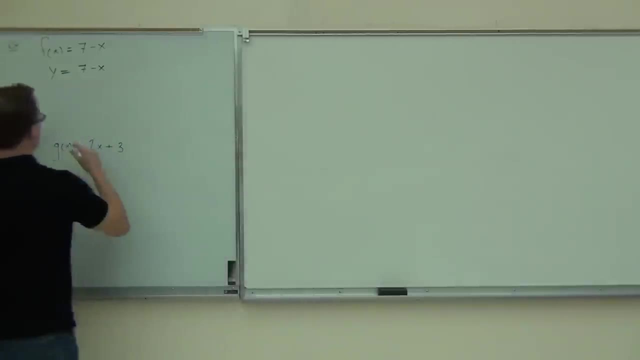 Now you're switching your variables. This is the act of finding an inverse. That's what we did up here with our simple points. That's what we're going to do here as well. So if you flip your, if you flip or you switch those variables, instead of y equals 7 minus x, you're going to have x equals 7 minus y. 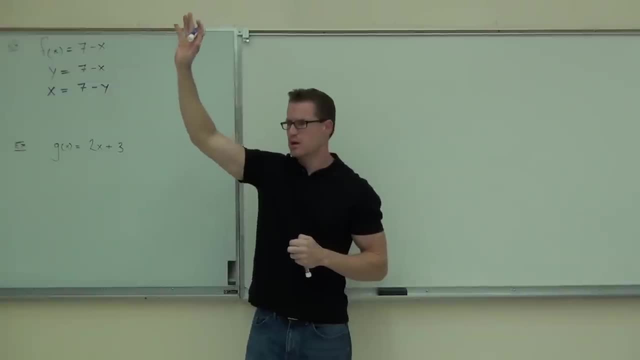 Raise your hand if you made it that far. That's an important step there. Good, Okay, that's great. Can you solve that for y? Can you solve that for y? Because that's your next step. You need to solve this thing and get y by itself. 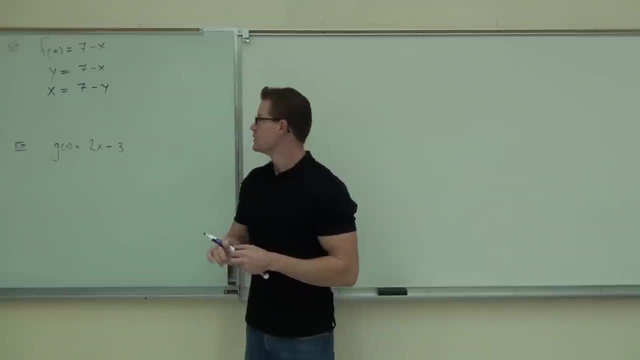 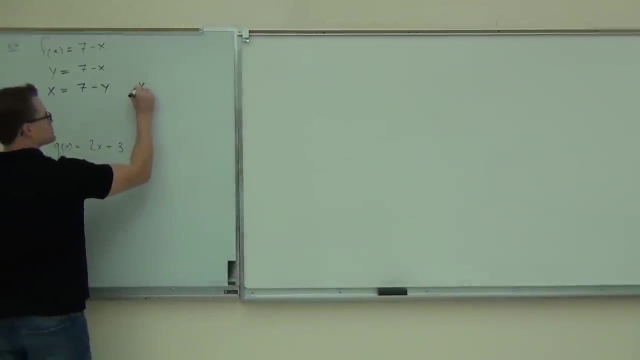 How do you do that? You can subtract 7 if you want. Sure, You're going to get x minus 7 equals negative y. If you do that, though, check it out: You're going to get x minus 7 equals negative y. 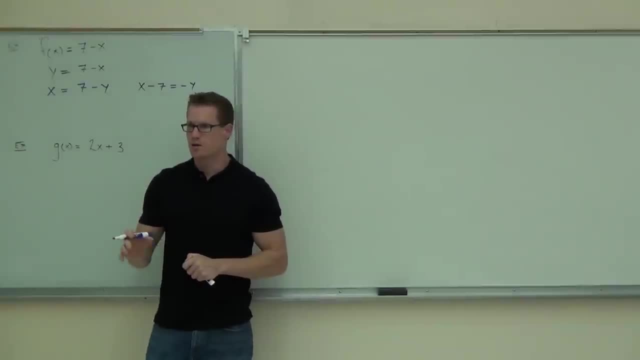 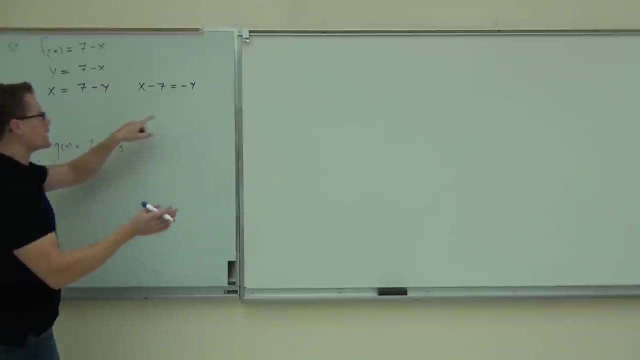 Yes, You're going to leave it negative y. No, you're going to change the sign by dividing by negative 1.. That means you're going to have negative x plus 7 equals y, Or you could do this a different way. 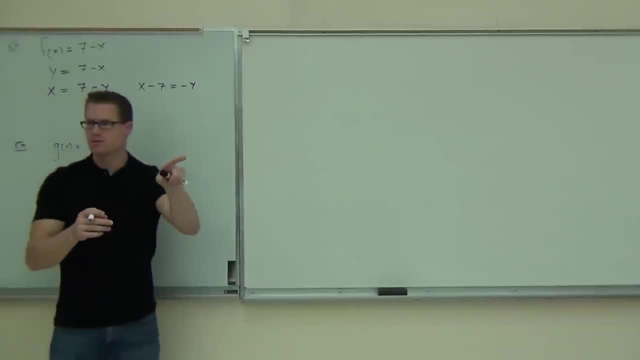 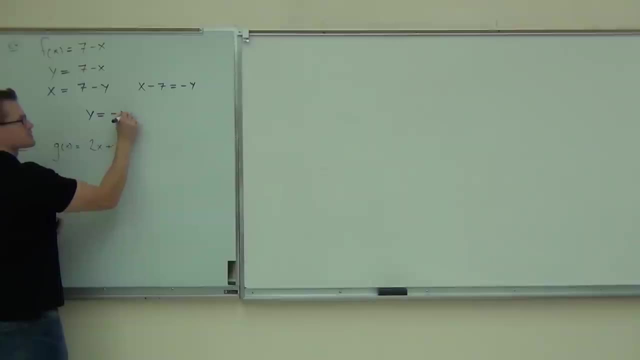 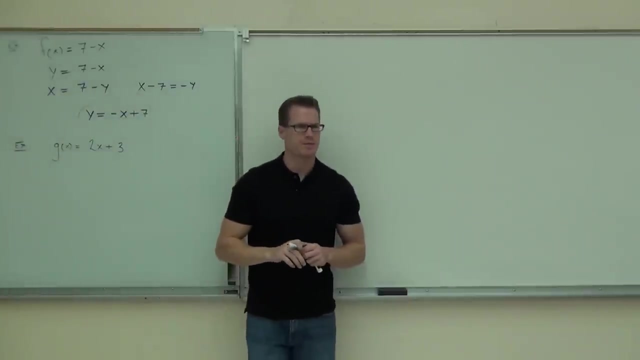 Over here. you could have added y And subtracted x. you know You could have done that as well. So either way, you're going to get y equals negative x plus 7.. It's a little head nod if you made it that far. 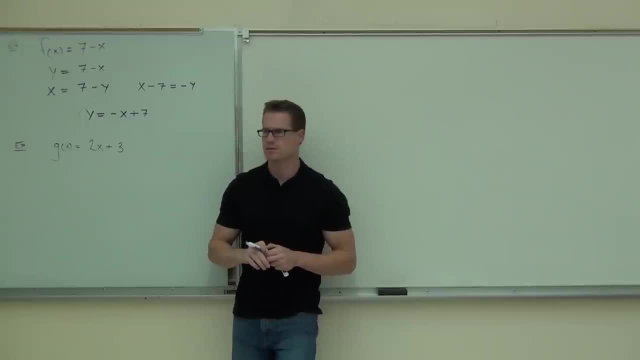 Did you make it that far? Some people yes, Some people no. Okay, If not, where did it happen? Did you make it all the way down to here? Yeah, Hopefully, If you made it to here and you couldn't make it all the way down to here. 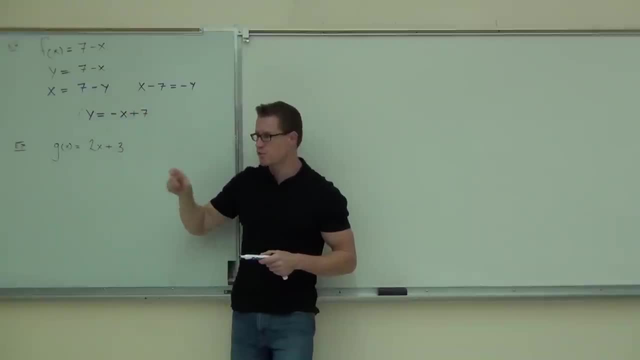 it's algebra, It's our basic algebra- moving things around. So watch that next time. Be careful on that little part. If you know you're making mistakes right there, go a little bit slower next time and try to figure that one out. 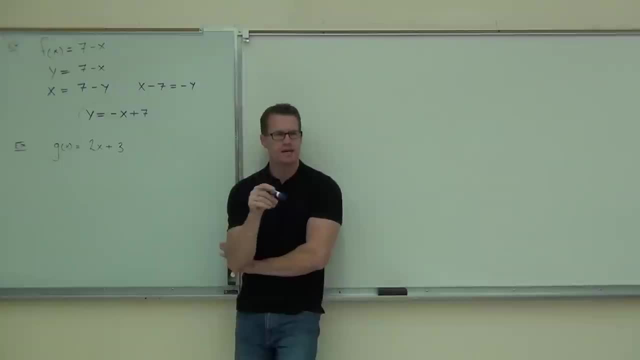 Hey, are we done? Should I leave it as y equals? You see, we invented that y, right? It's kind of like a dummy variable. It took the place of our function so we could work with it. You have to list it back as whatever function you started with. 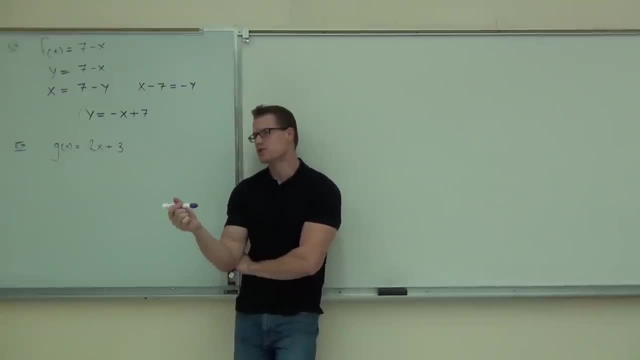 So if we start with the function f, we better write these things at inverse. You see, right now this is an inverse function of that one, but it doesn't say that yet. That says we just have another function named y. You have to write this back as the inverse function. 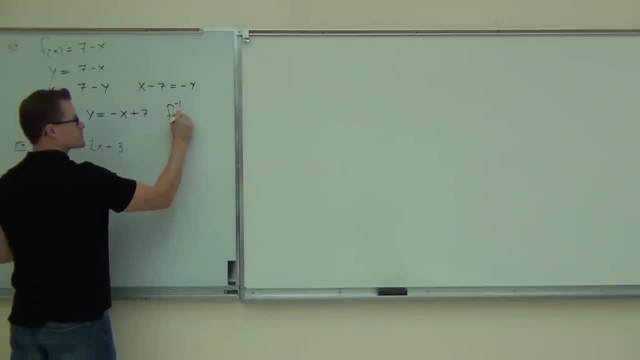 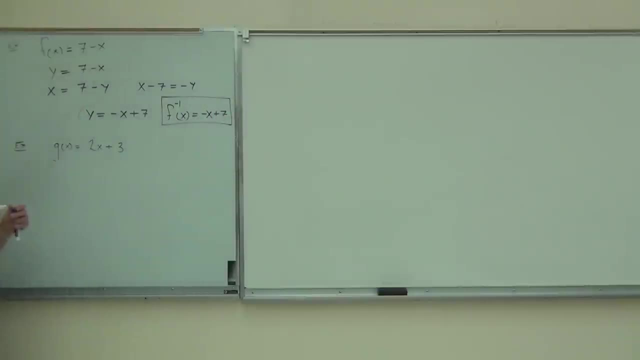 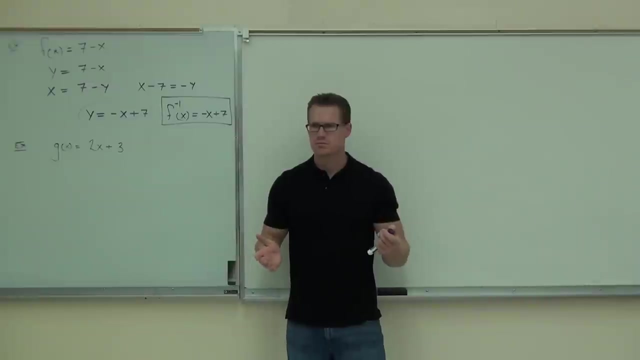 So instead of y, we write f, inverse of x negative x plus 7.. That's our final answer: Yes, no, Yes, you got it, Or no? Some people? yes, Everybody. That's good, All right. 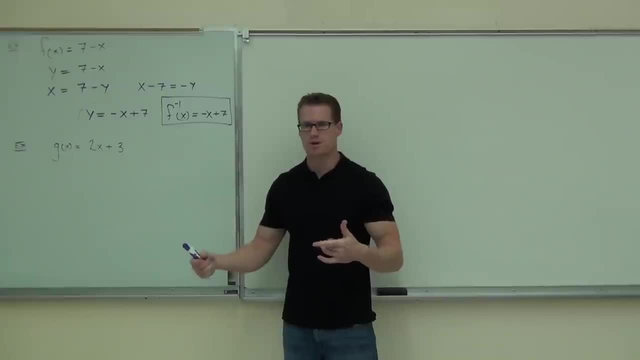 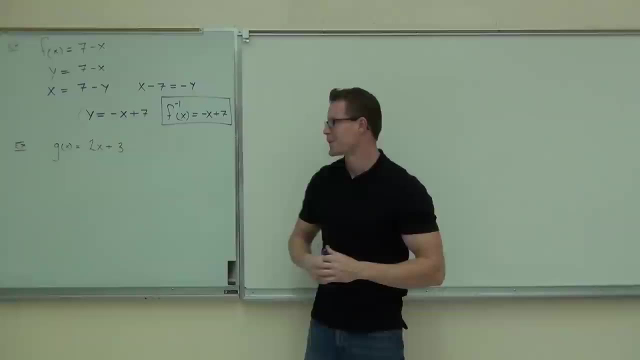 Do you understand the idea of why we're doing this, why we're finding an inverse? We're trying to find out what function is going to undo this one. That's really important for a lot of your later classes: finding an inverse function there. 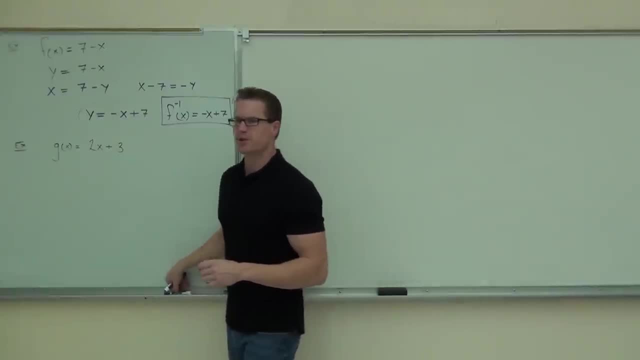 Now the last one. we'll do this together, But I want your help on it. The first thing we're going to do: if we have g of x equals 2x plus 3, y'all tell me what's the first thing you'd want to do here. 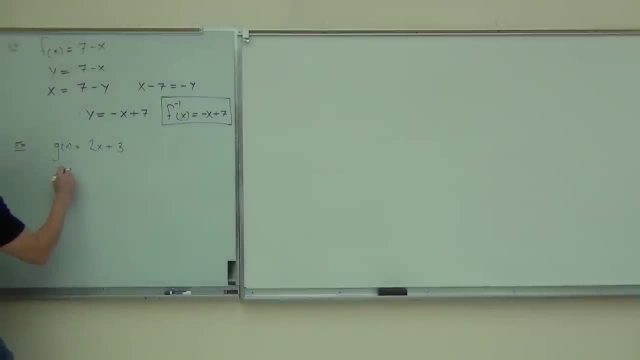 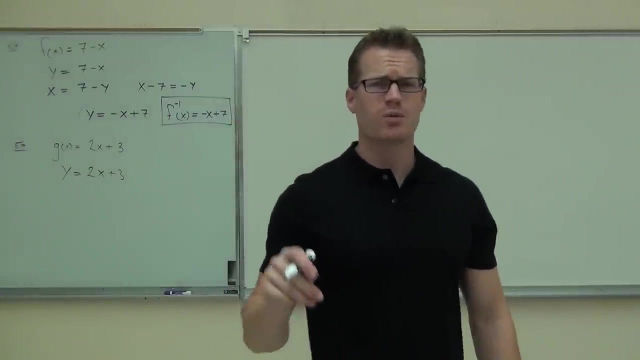 Y, Y, great. Okay, so we're going to have y equals 2x plus 3.. Very good If we have y equals 2x plus 3, the next thing we want to do is what? Okay, switch x. 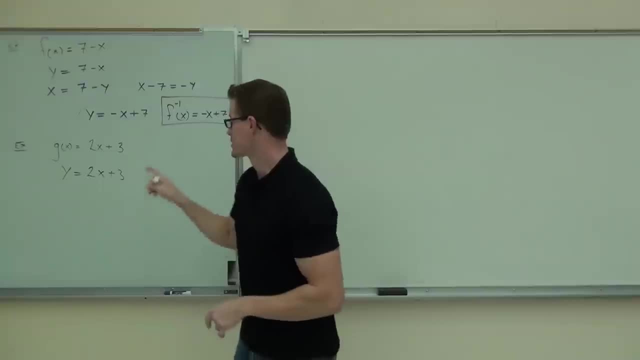 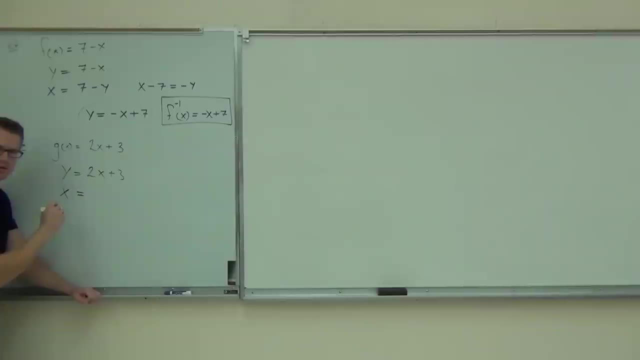 Someone in one of these two rows tell me what I should have exactly if I switch my x and my y. What's the first thing? Okay, good, So x because y becomes an x. What's now? 2y plus. 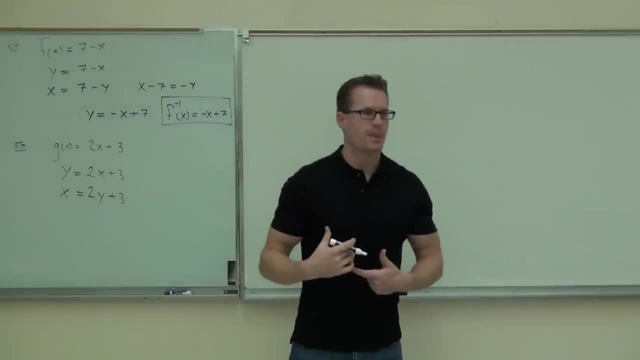 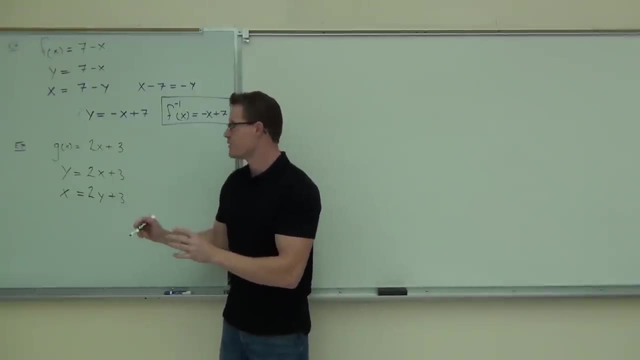 Yeah, that's exactly right. Can you follow how she did that? You follow how she did it. So the x now becomes a y, The y becomes a y. That's all you're doing. You're not doing any other, like mathematics in your head or anything. 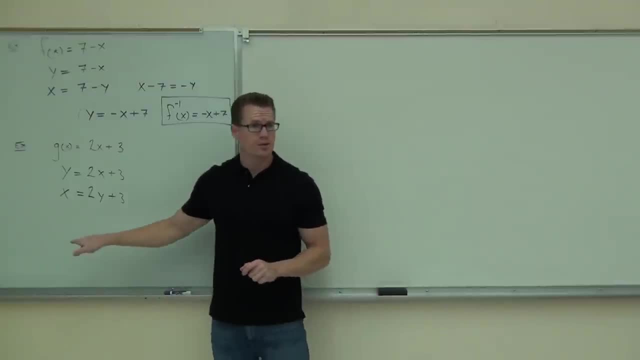 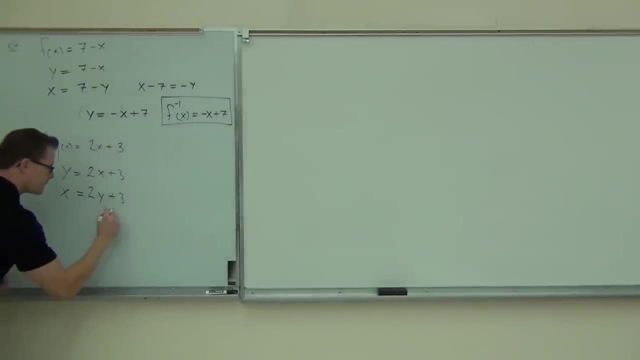 X becomes y, Y becomes x. That's it. Now can you still solve this thing for y? Sure, Let's do that. How do you do it? So x minus 3 equals 2y. You're going to leave it like that. 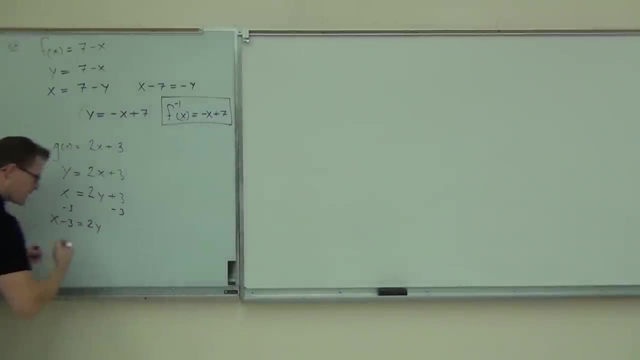 Ah Yeah, we do that. If we divide both sides, that means everything everywhere. You're going to get x minus 3.. You're going to get x minus 3 over 2 equals y. That's great, That's great. 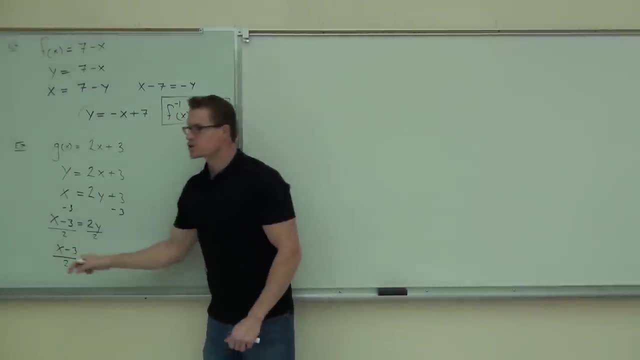 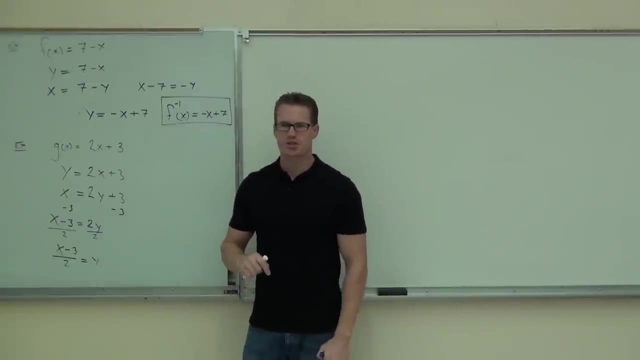 Are we done? No, You're very close, though. You do have the inverse function. That's right here. You've just got to make sure you call that an inverse. So can you tell me, if I want to change my y to something that says inverse, what am I going to change it to? 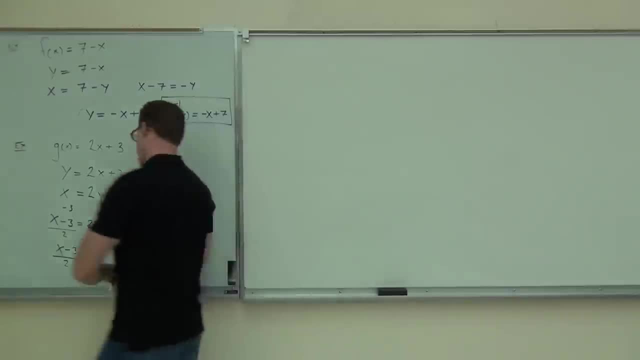 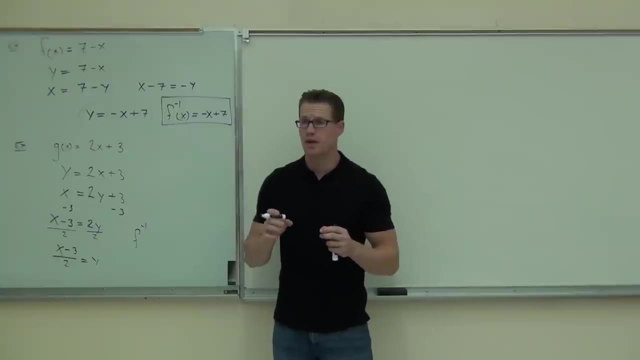 g inverse. Wait now, is this appropriate? No, because the function is not enough. So be careful: You don't always put an f inverse right, Because if you do, you're not going to be able to solve it. 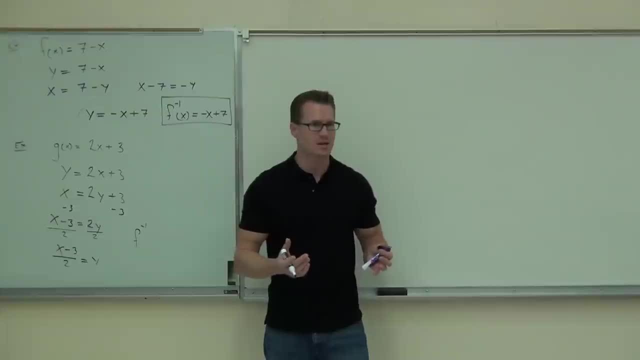 You're not going to be able to solve it. You're not going to be able to solve it Because if we don't have a function f, well, that doesn't make any sense. This would be like: well, go look for your function f. 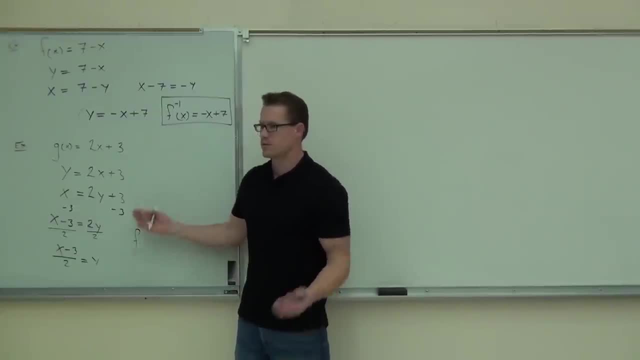 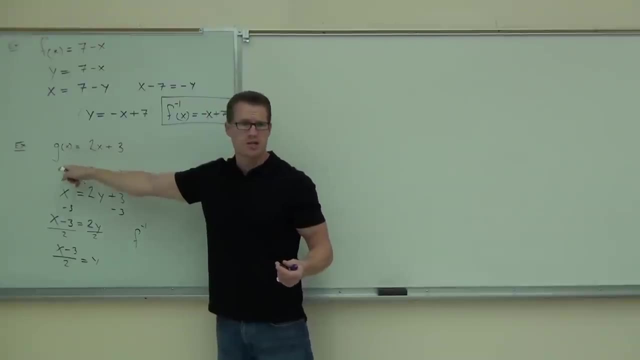 And you're like: what function f If that's not on the board? what function f? right? So it doesn't stand for that one anymore. We're trying to say this one: If you had a letter g there, we want to say that the inverse is now not f inverse. 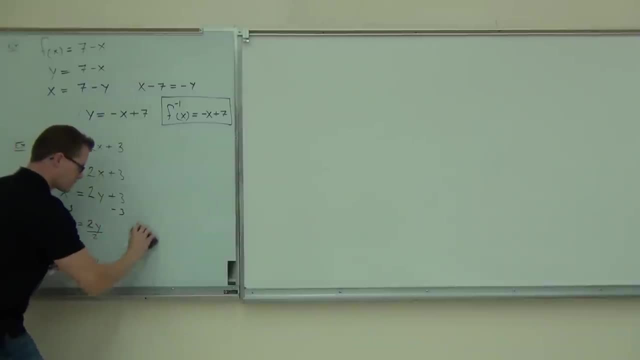 It's g inverse. Do you follow that? So you get what's the letter that you're using? How about we just rewrite this part: x minus 3.. x minus 3 over 2.. And we're done. That's our inverse. 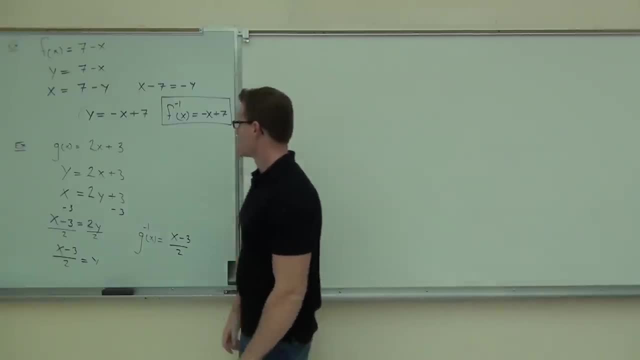 And in fact you could check it right, You could plug in a number. If you plug in a number like, oh, I don't know, 1.. You plug in 1 here, you're going to get 5, right. 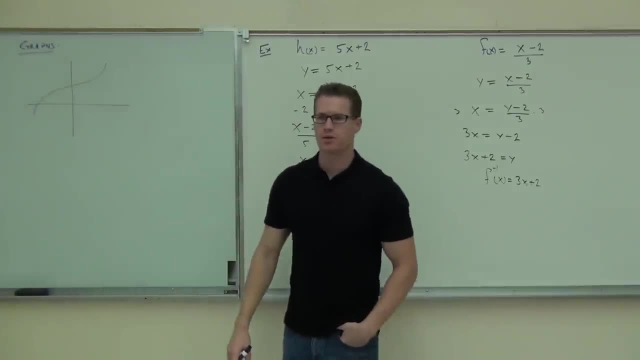 Firstly, can you determine that this thing is a function? Function would be vertical line test. Does it pass the vertical line test? Is it a one-to-one function? One-to-one would also pass the horizontal line test, saying I don't have any non-unique. 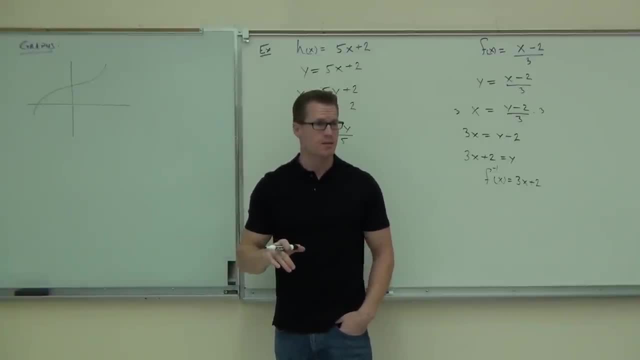 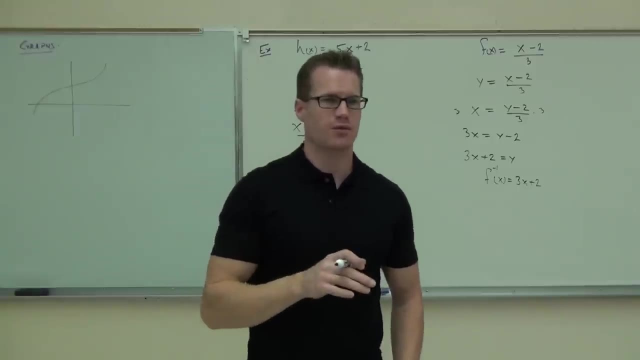 Output says everything is unique. Does it pass the horizontal line test That says this is one-to-one? If it's one-to-one, it will have an inverse. Here's what an inverse does. I want you to think carefully, okay. 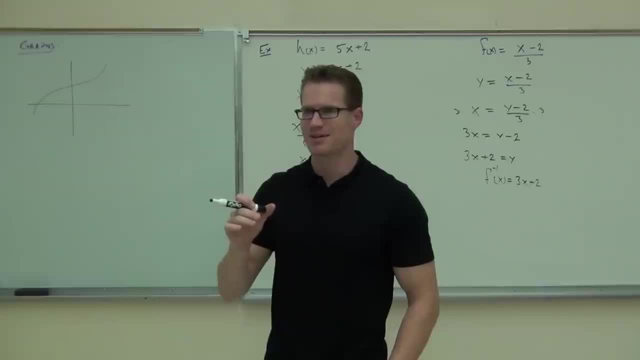 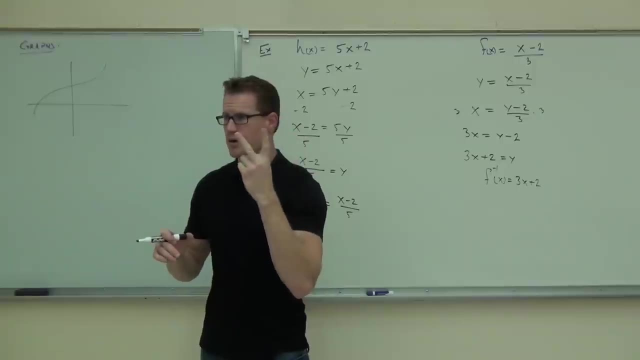 Are you ready for this? Are you ready for this? Are you guys awake? It's kind of cool. What we've been doing the whole time to find inverses is simply switching our x with our y, You follow. So if we switch our x with our y everywhere around here- take a random point, for instance. 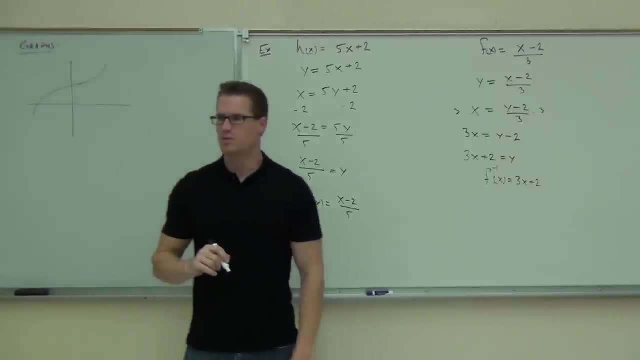 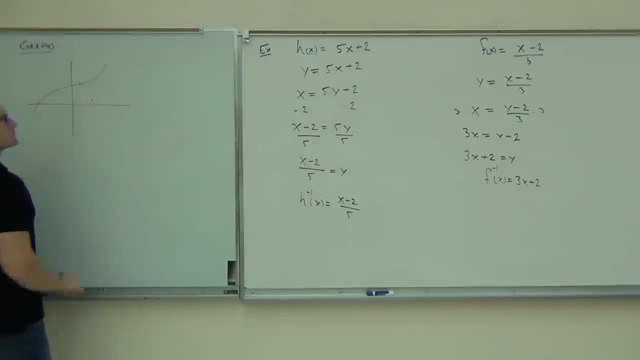 That's the point. It's going to be 1 comma 3, you follow, That's 1 comma 3.. If I switch that, that would give me 3 comma 1.. That would be about here, True. If this is, let's see: negative 5, 2, negative 5, 2, it would give me 2 negative 5.. 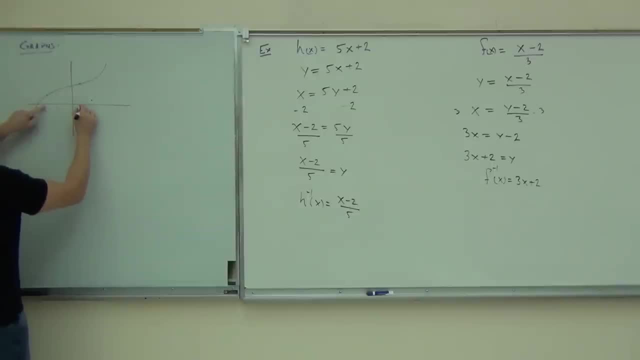 Negative 5, 2, it should give me 2 negative 5.. It's right down there What this does. if you imagine this line, that diagonal line, what an inverse does. it flips a function across that diagonal line. 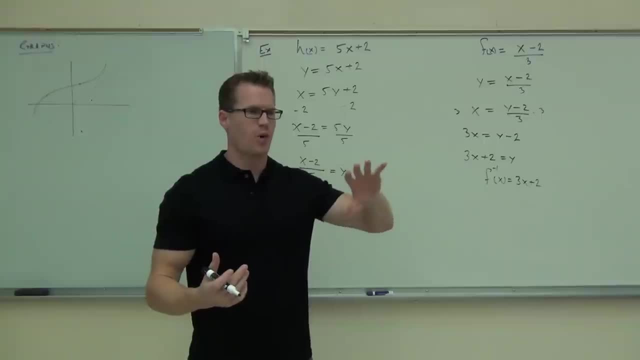 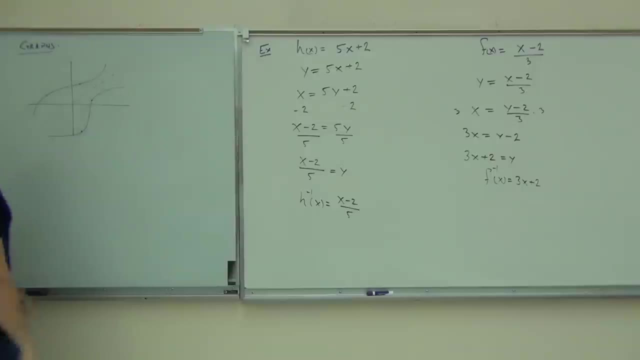 That's all it's doing. It's flipping your x and your y right, So x's become y's and y's become x's. So it's taking this thing and saying, oh, now you are that thing. I tried to draw that as good as I can. 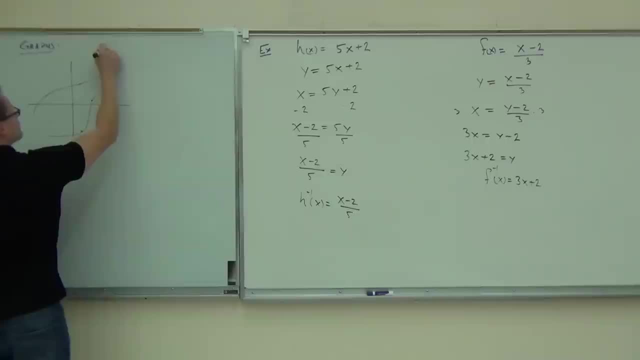 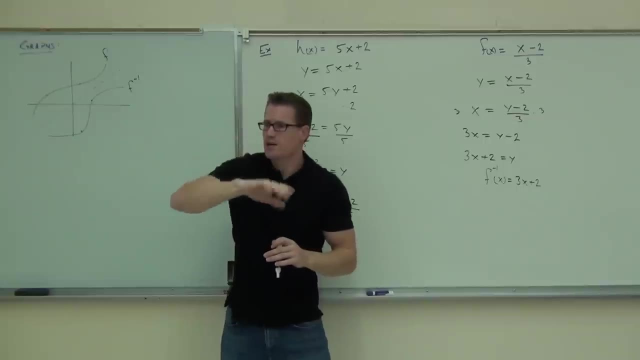 It's kind of weird. I'm not a hard, I'm not an artist, But if this is f, that's f inverse. It says you take your function, it's flipping it across that diagonal line. That diagonal line, by the way, is the y equals x line. 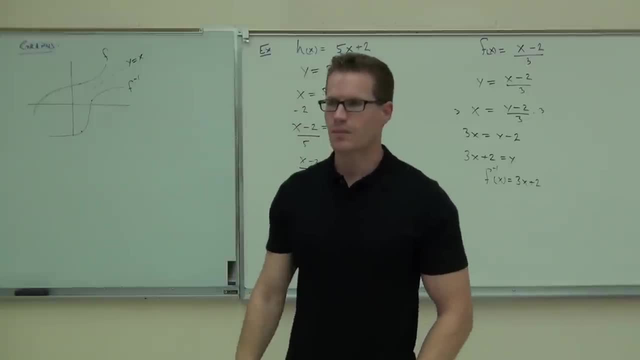 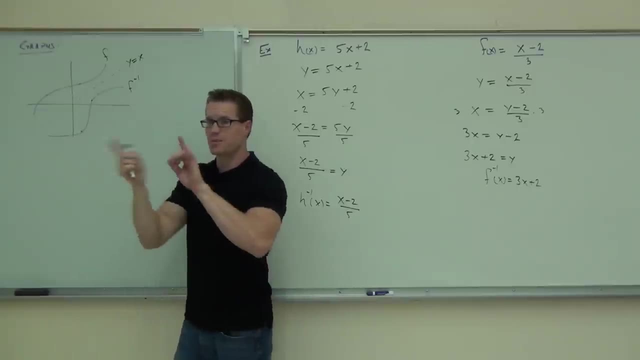 The y equals x line. It's a simple diagonal line. But by flipping your x and your y coordinates it's taking all of your y's and making them x's and all of your x's and making them y's. It's flipping those two things. 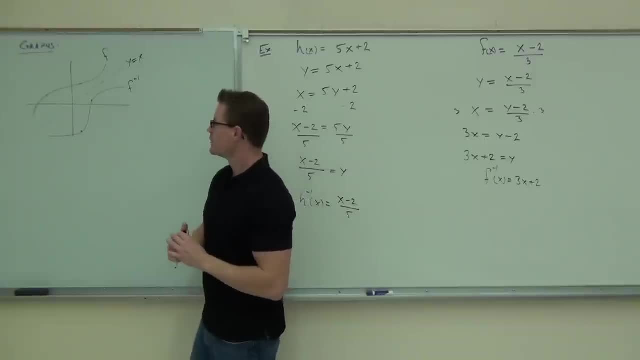 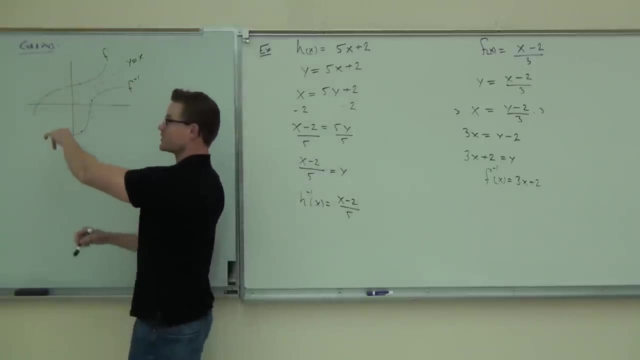 Yeah, So it just makes it parallel. No, they're not parallel. They're reflections of each other. They're reflections. It's saying it's a mirror image across that line. Now I know it doesn't look like a mirror image. 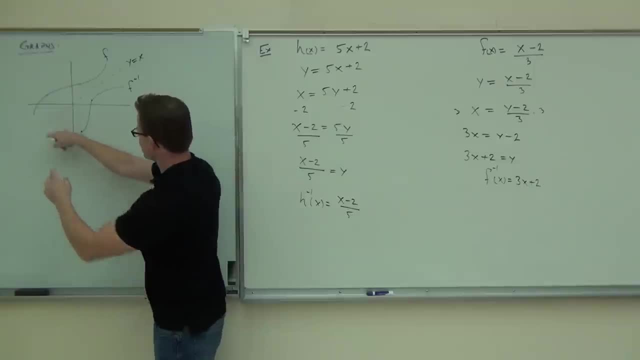 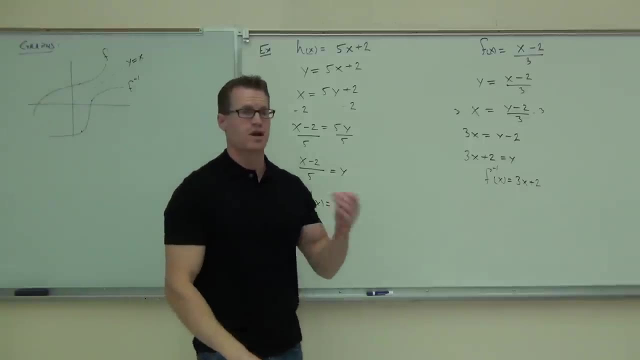 It's whatever, But it needs some weight across the line. That's okay, But this is- this should be a mirror image of that function. By switching your x and y, that's exactly what happens. Do you guys understand graphically what's going on here? 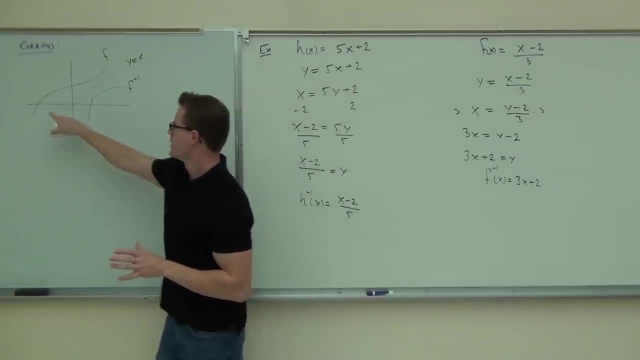 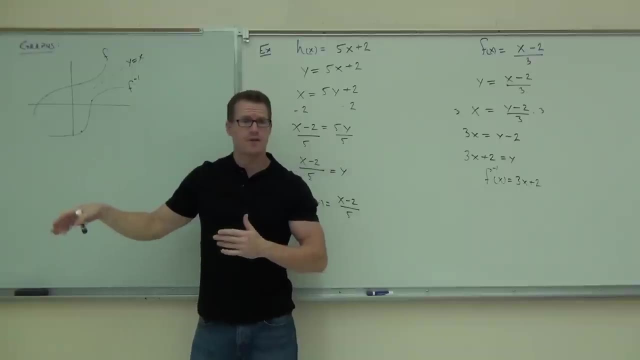 The reason why you cannot have a non-one-to-one function, because if you have a non-one-to-one function when you reflect it, it's not even a function. The horizontal line test would become the vertical line test for inverses, And these have to pass both. 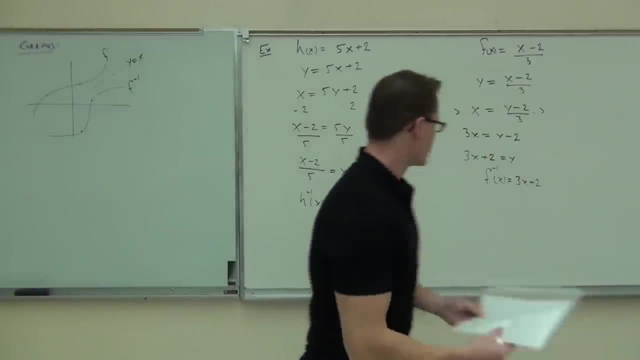 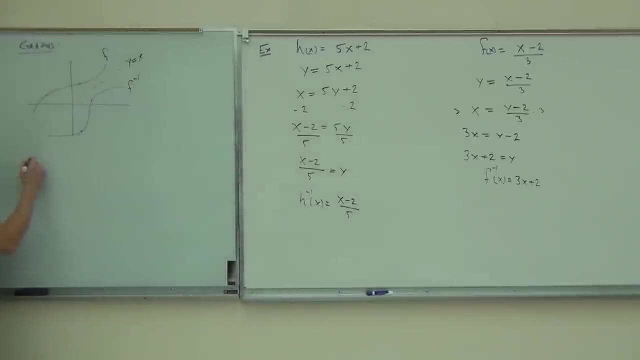 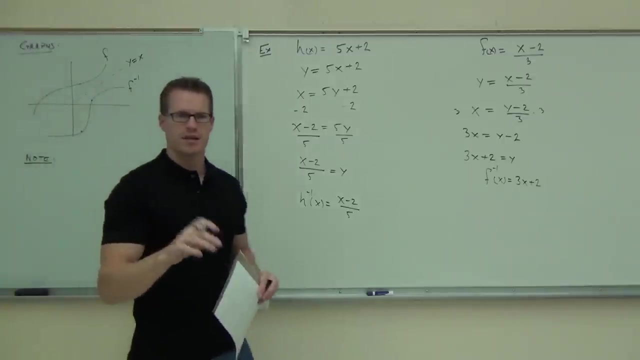 Otherwise you can't find an inverse. Now one last thing. Here's a way you can check to see if two functions are actually inverses. One kind of important note: Do you remember those compositions we did in the last section, 12 and 13?? 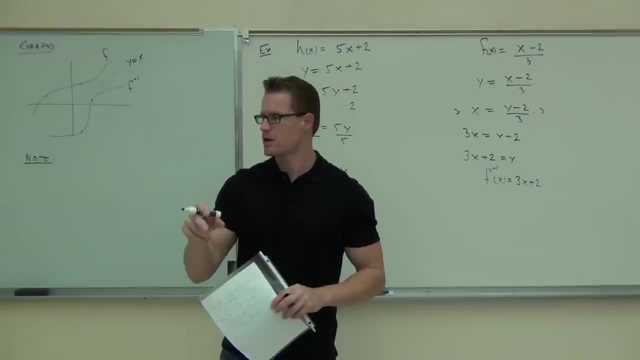 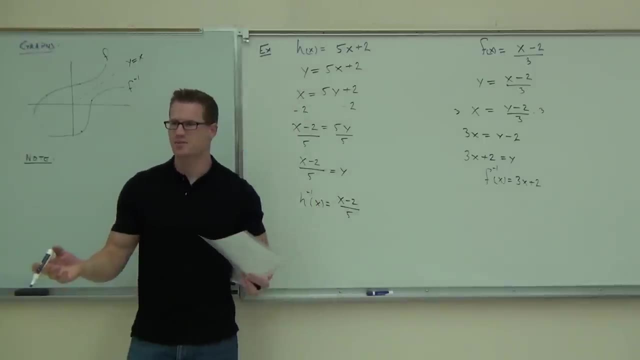 Yeah, The section 12.1, where you put one function inside the other function. A composition of inverses must give you out x. That's going to be kind of weird, Like wait x. I thought it was supposed to be like zero or one. 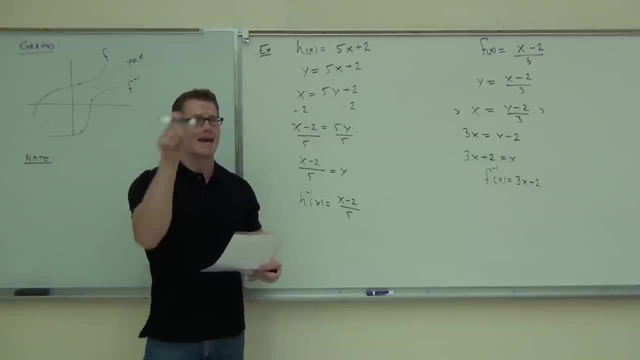 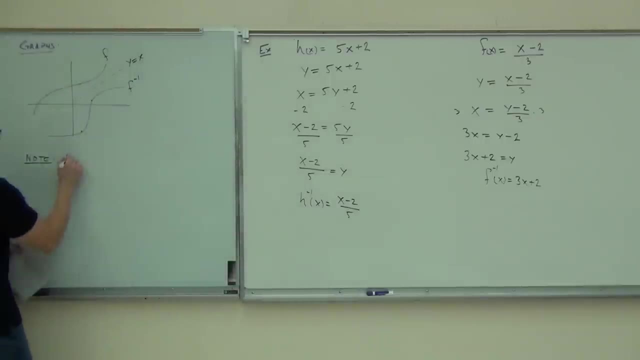 It should be nothing. Well, what are you plugging into a function? You're plugging in x. Right, The composition should give you out x. We'll see that in a second. The composition Of a function and its inverse must equal x. 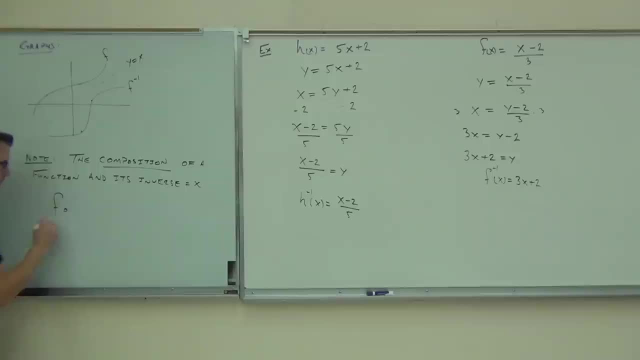 So, for instance, you familiar with that, the f with that little open circle F, of If I have a function and its inverse is equal to x, then I'm going to have a function and its inverse is equal to x. 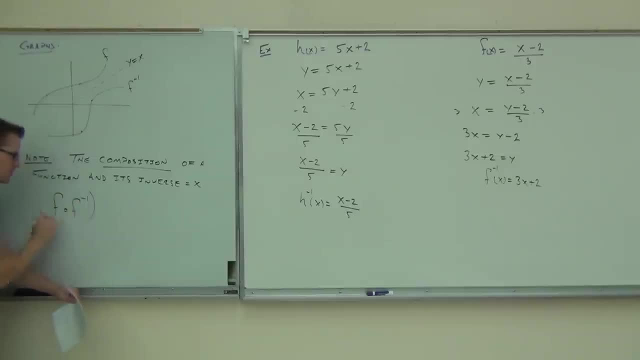 So, for instance- you familiar with that- the f with that little open circle, F of- If I have this right here- f of f inverse, which means I'm composing f inverse inside of f. that thing has got to be equal to x. 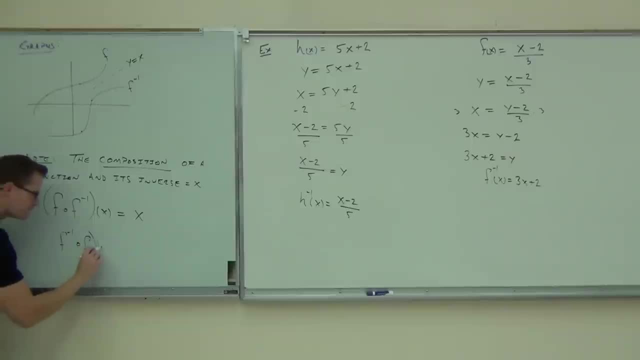 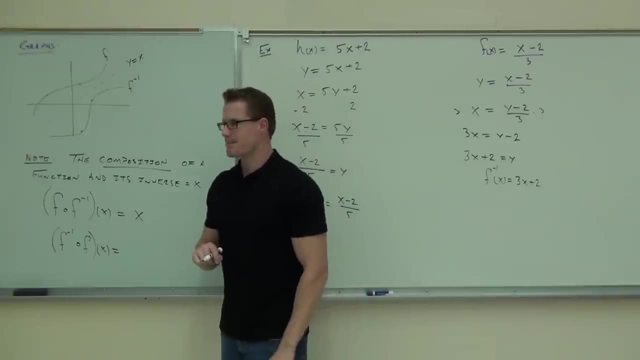 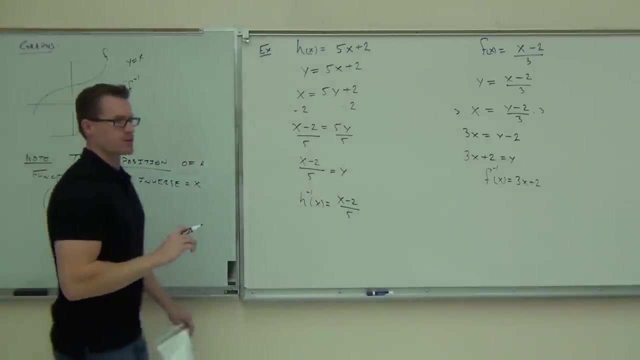 Same thing. if I do it in reverse. This is the only time in mathematics where you compose two different functions and they equal x. They equal what you're actually plugging back in, Or they equal the same thing in reverse. Do you remember all those times where we did f? 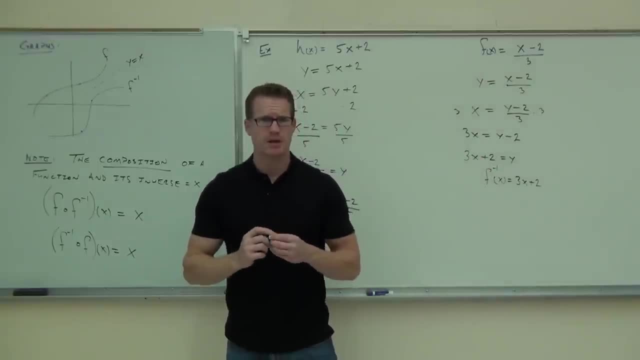 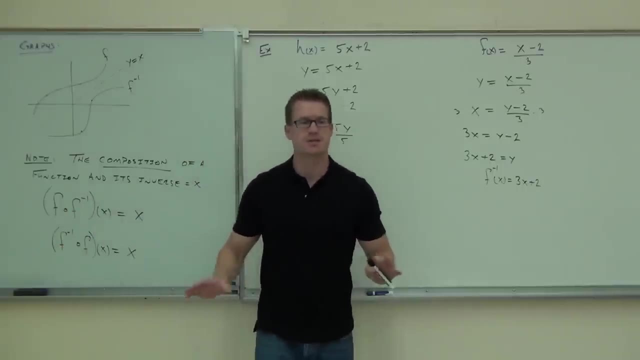 F of g and we did g of f and they were completely different. Do you remember that? This is the only time where you can reverse the operation of that composition and it gives you the same thing. The only time that that happens is if you have an inverse. 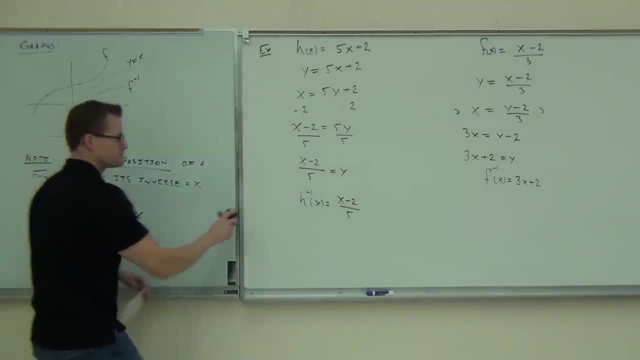 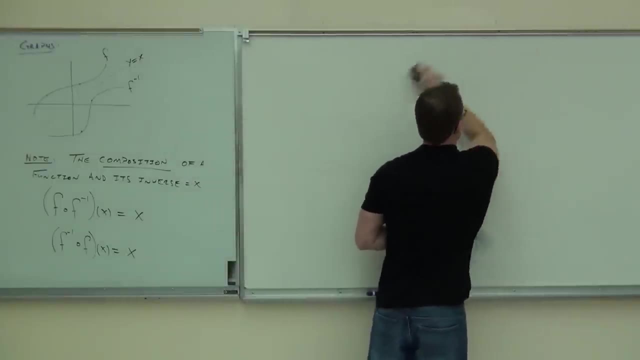 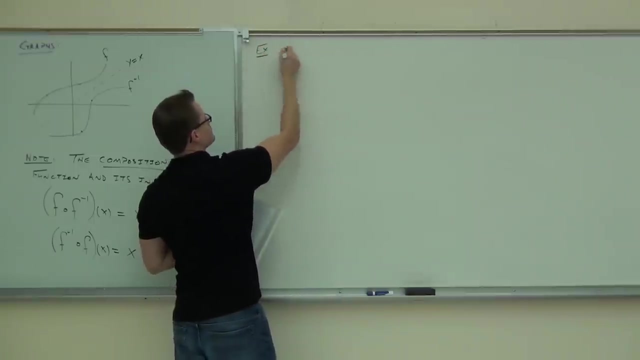 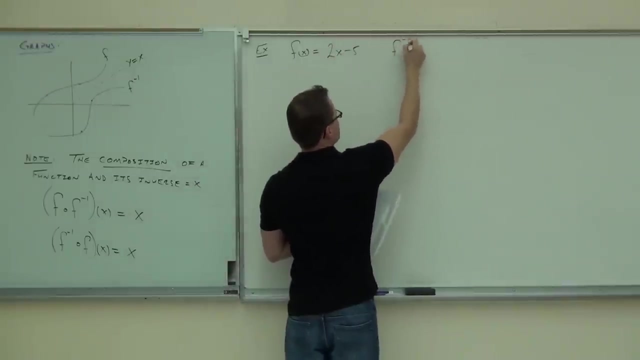 Let me give you one quick example on how this works. I'll show it to you And we'll be done. So let's say that I tell you: F of x equals 2x minus 5, and f inverse of x equals x plus 5 over 2.. 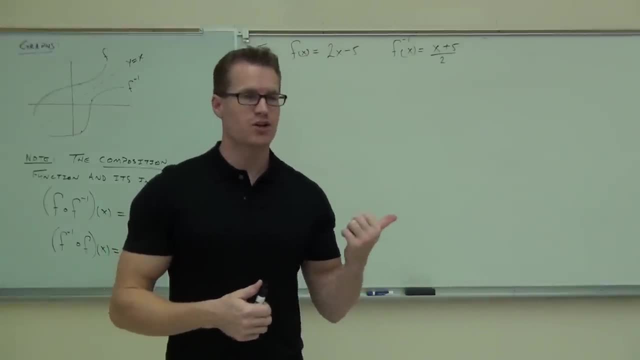 And I say, hey, trust me, those things are inverses. Are you going to trust me? Well, yeah, probably because I'm a math teacher and because I'm an honest guy generally, Generally, Generally. Yeah, White lies are just. 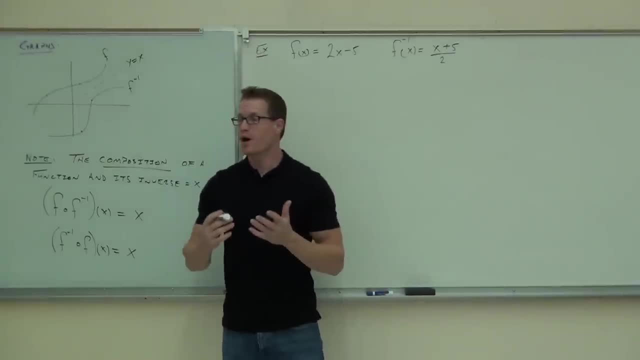 No, I'm not. I'm an honest guy, But you would probably trust me. But what would happen if I made a mistake? You've seen me make mistakes in this class, right? This doesn't happen often, But no, I'm just kidding. 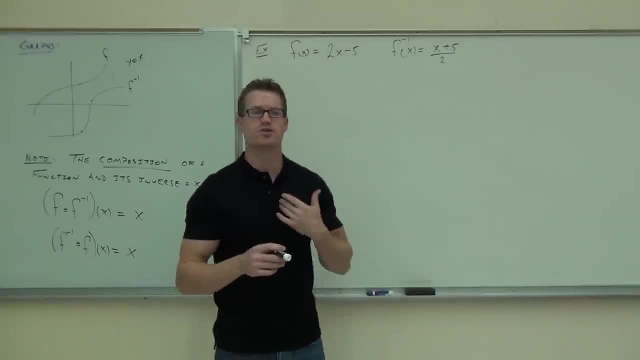 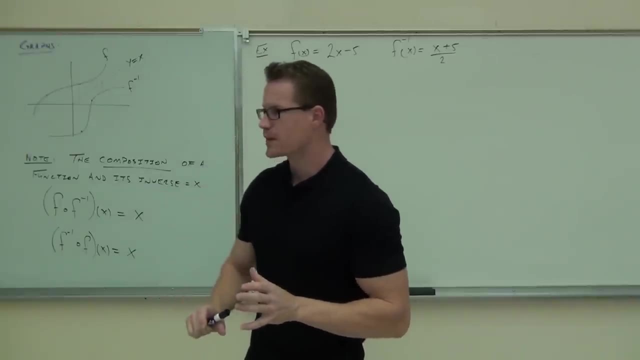 But it does happen occasionally. What if I made a mistake? Is there a way you can check my work? Is there a way you can check your work to make sure you actually found the inverse, without doing it over again, Because you don't want to just repeat the same mistake over and over, right? 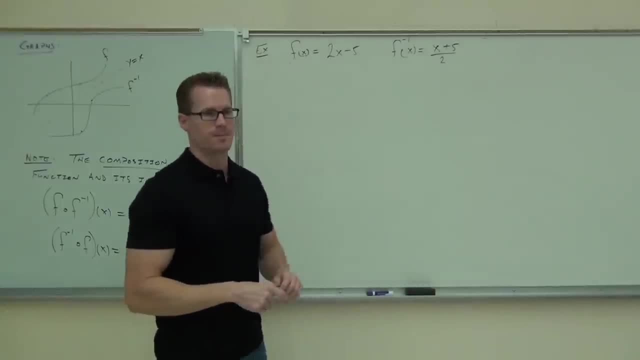 Because that won't show you whether you're making a mistake or not. There is a way. Here's the deal. I'll show you this twice. I'll show you each composition. I'll show you. they're exactly the same. You only have to show me one of these. 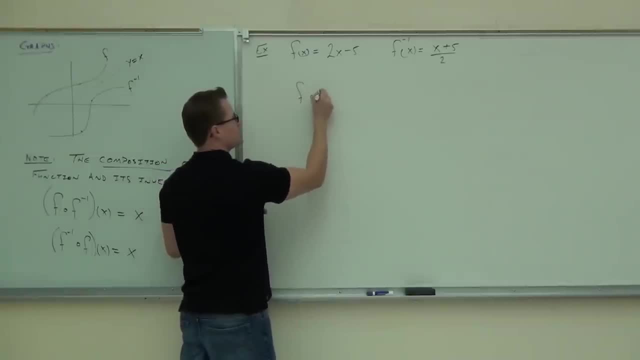 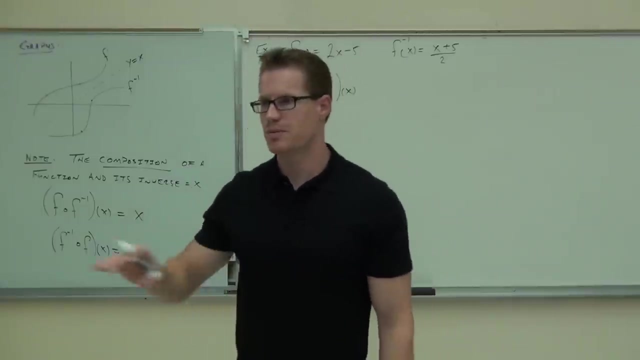 So it's your choice whether you want to show me f of f inverse or f inverse of x. Both of these will come out to the same thing. Now can you tell me, just by looking over here, what do these ultimately have to equal to prove that those are inverses? 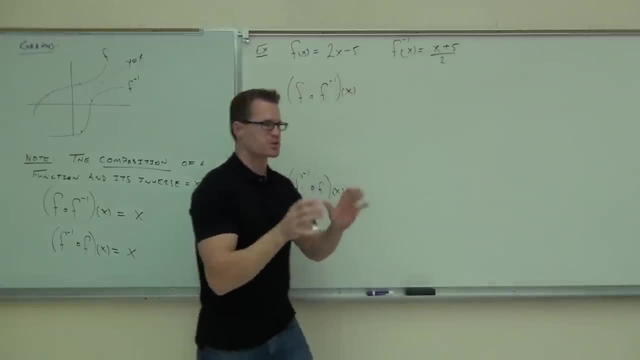 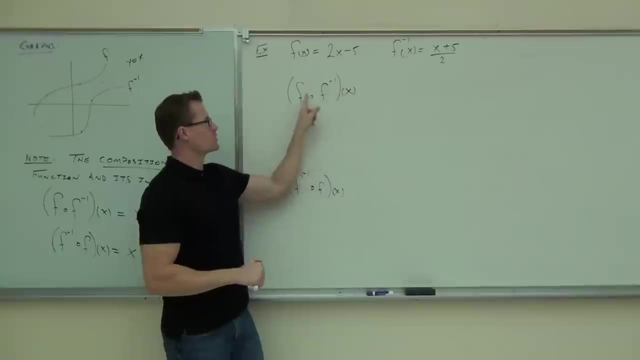 They've got to equal x, Why Think about it? Look at the board right now. Stop working for a second. What are you plugging in here? It's saying you're plugging in x. right, It's got to go through the function and the inverse. 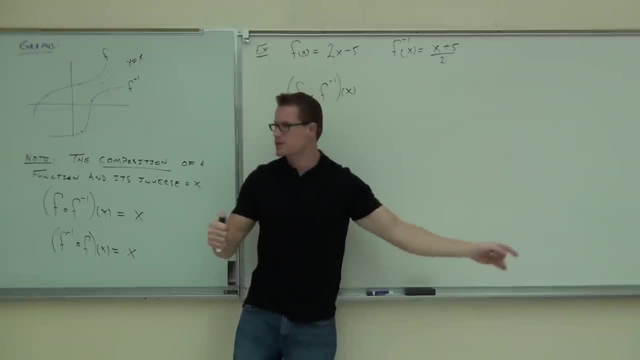 It's going to give you whatever you started with. It's going to give you out that x. That's why you don't get a 1, because you're not plugging in 1.. You're taking whatever value. I'm saying, That's x. 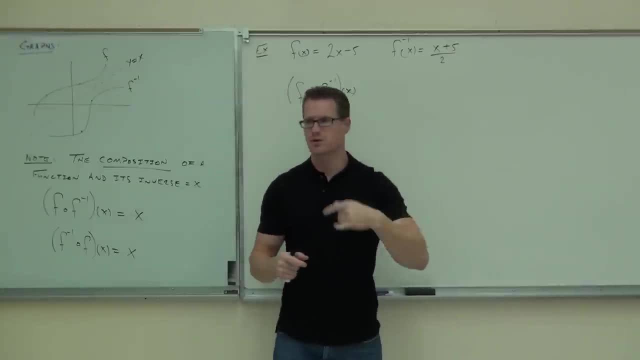 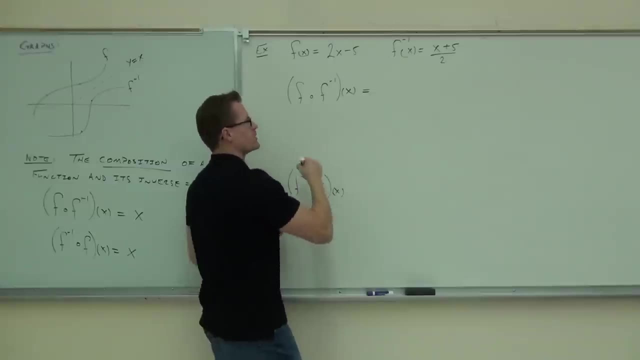 So this thing will ultimately give you out x. Now we're going to go through the function composition really quickly, because we covered it last time. If you're talking about f of f inverse- hopefully you remember this- We write this first as f of f inverse of x. 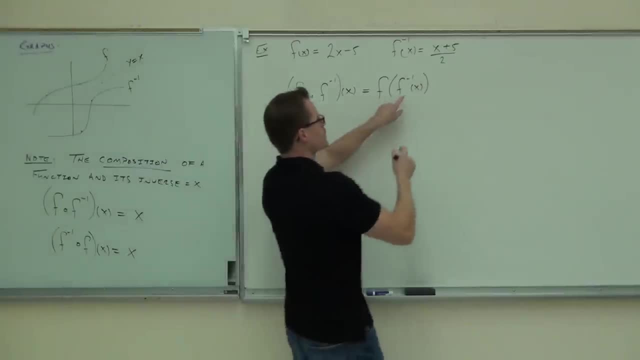 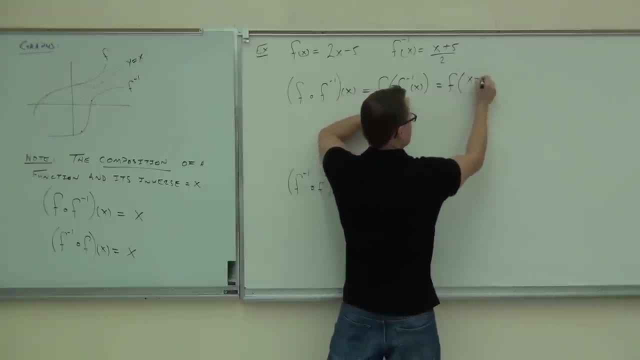 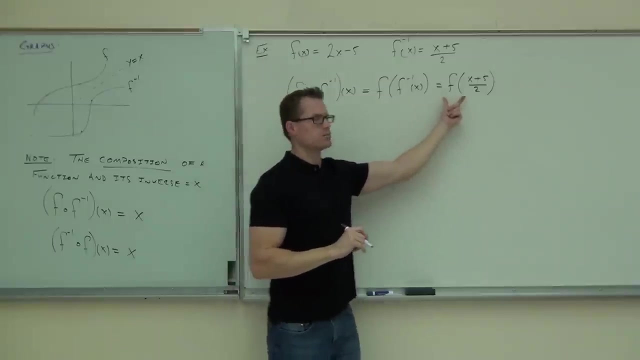 Do you remember that? Then it says: okay, you leave this f. You guys should be pros at this right now. You leave this f alone, but inside you're going to write f inverse. Still, so far, so good. So f inverse. you now write: well, f inverse. 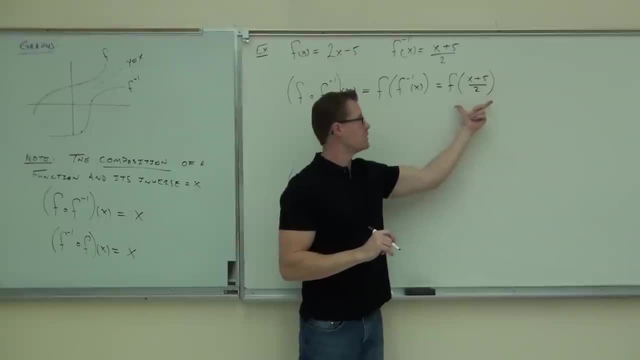 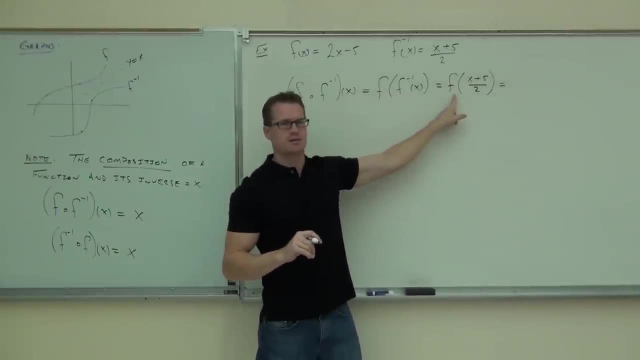 What's the only letter left on the board that represents a function. Are you with me? It says you're going to write f. You're going to go up to what's f say 2x, So 2x minus. is this coming back to you? 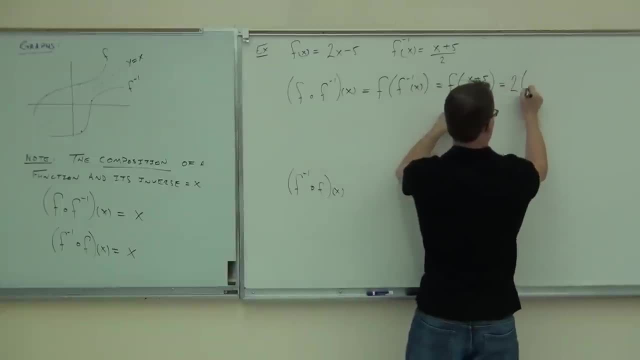 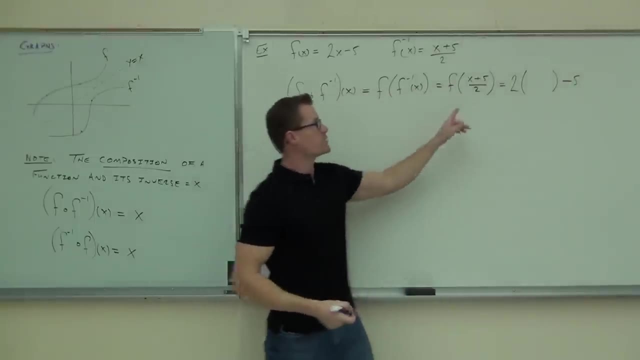 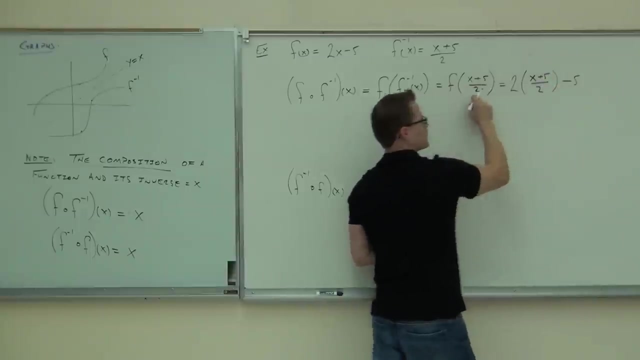 2x minus 5, that's 2 parentheses Minus 5.. Can you tell me what goes inside that parentheses? Well, that's exactly what we had in that parentheses. Now what happens? Do you see any simplification you can do? 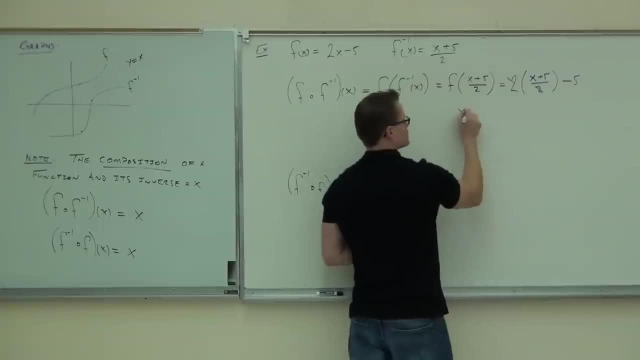 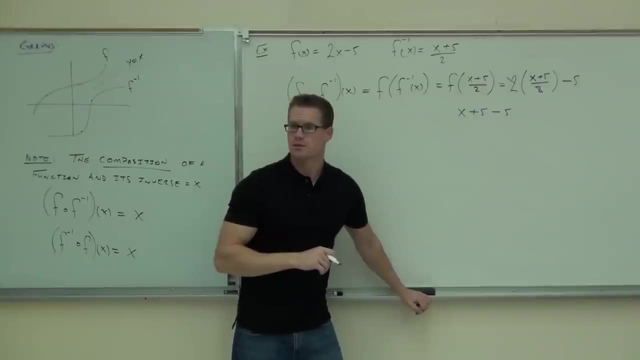 2s are gone, You get x plus 5 minus 5.. 2s are gone. What happens to the 5s? What do you get? So are these things in fact inverses. If you had gotten anything else besides x, would they have been inverses? 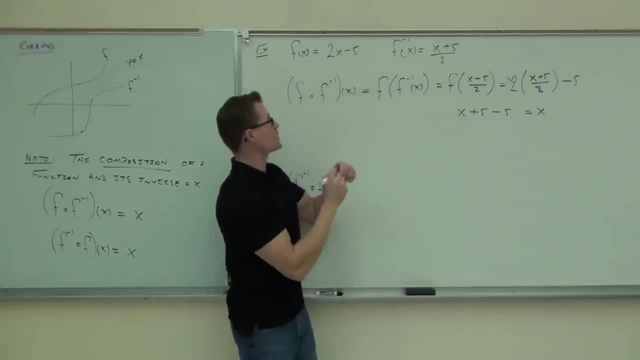 That's it. It's undoing what you plugged in. This said you started by plugging in x, went through both functions and gave you out x. That means the inverse actually undid the function. Now let's see if this works in reverse. 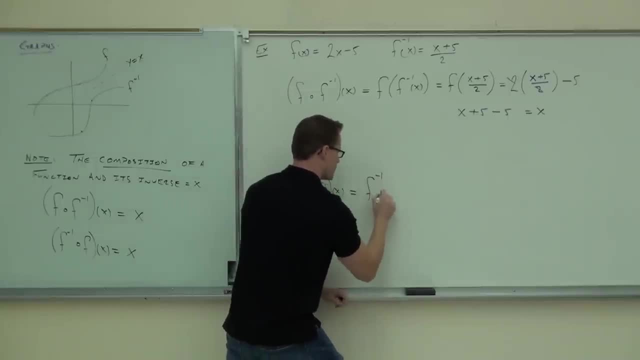 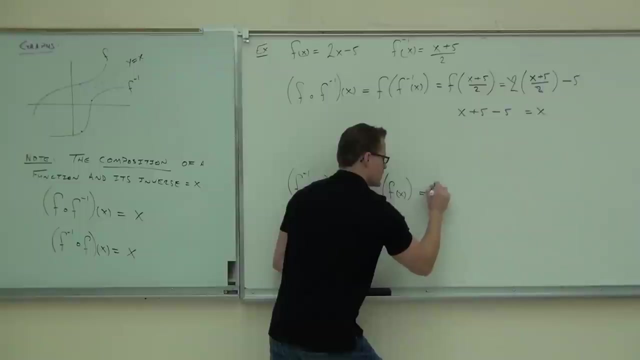 I'll bet you a billion dollars it does You need a new car, don't you? Yeah, f inverse of f of x. That's the same thing as this f inverse of f of x. We leave our f inverse and in the parentheses we put our f. 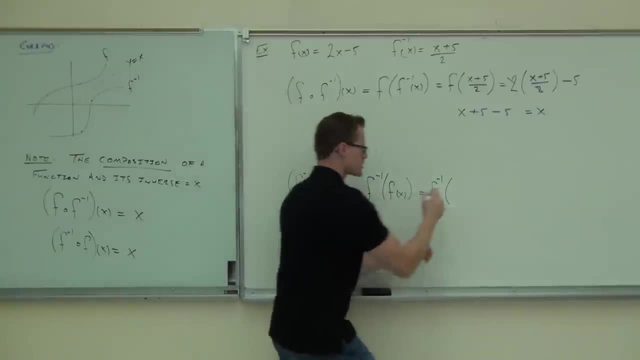 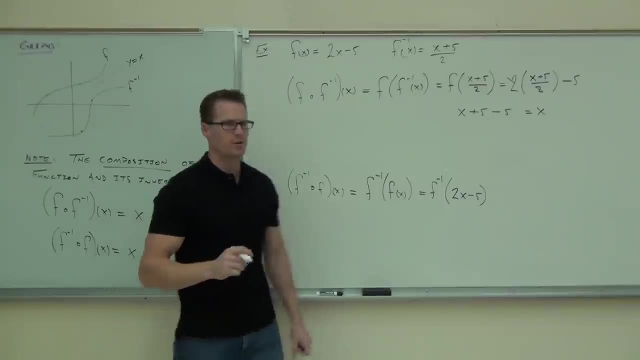 What's our f of x again? So we're going to put our 2x minus 5 inside, Inside of our parentheses. What now? We're going to plug it into the f inverse. Okay, So we look at f inverse. 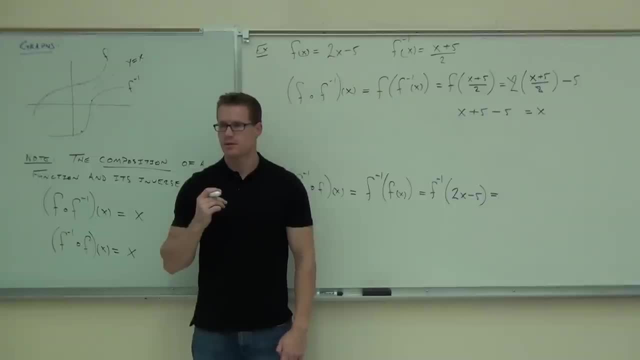 What's f inverse, say x plus 5 divided by 2. x plus 5.. So x plus 5 over x plus 5.. Are you still okay on this stuff? Parentheses plus 5.. I need to know. 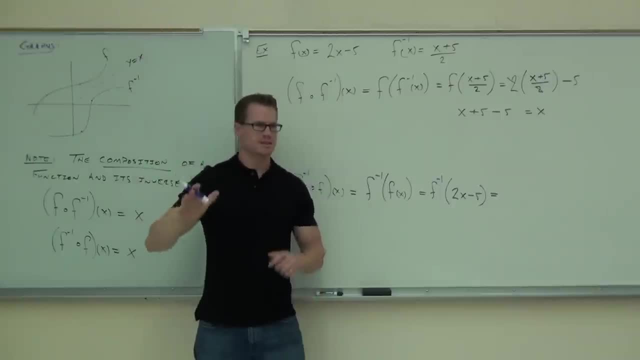 How many people feel all right with what we're doing here? If you're not, if you're like, oh not, so This is our inverses, right, This was our. You had to be okay at the 12.1 to be able to do this. 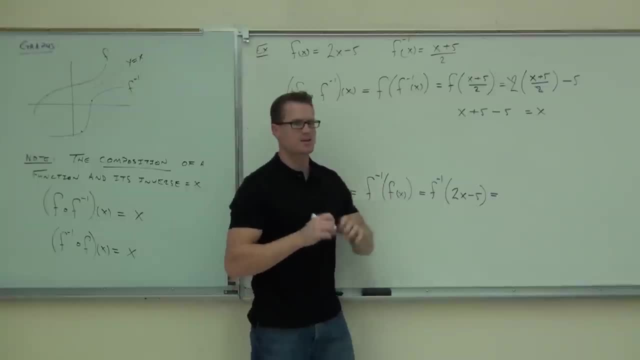 So we look back at our inverses. We say x plus 5 over 2.. Actually that's parentheses plus 5 over 2.. Can you see that this is actually the f? inverse? That really is Parentheses plus 5 over 2.. 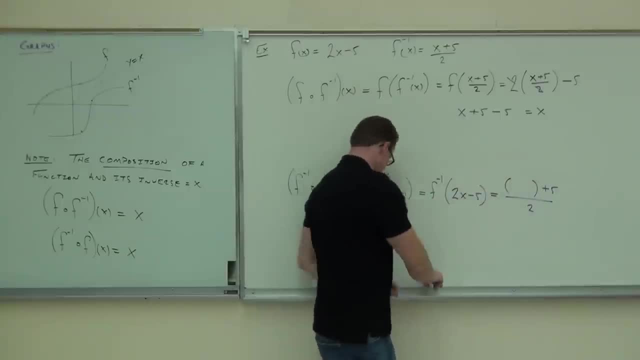 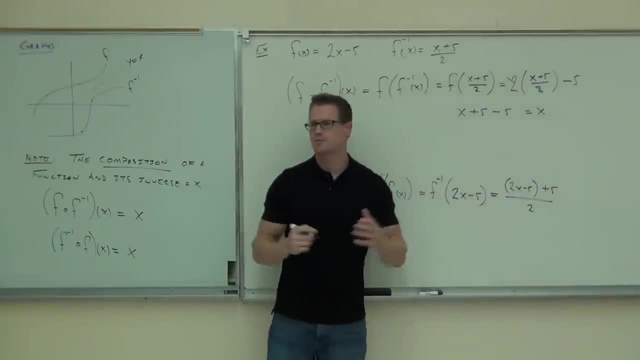 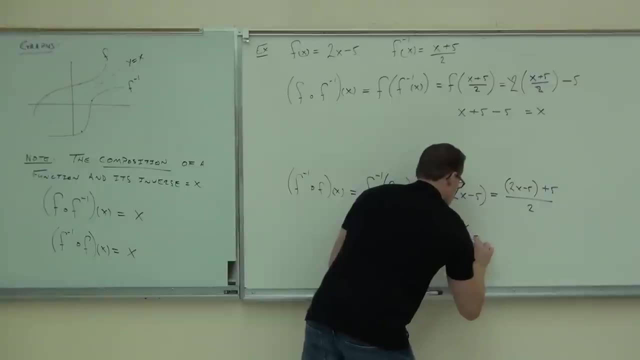 That's 2x minus 5.. That's 2x over 2.. What happens here? The 5s count to each other. on the 2s also. 5s are gone. 5s are gone, We're going to get 2x over 2.. 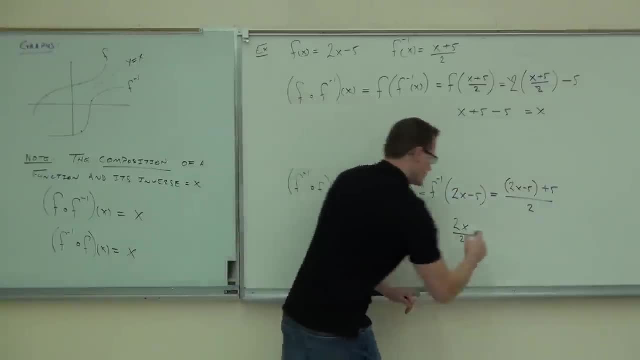 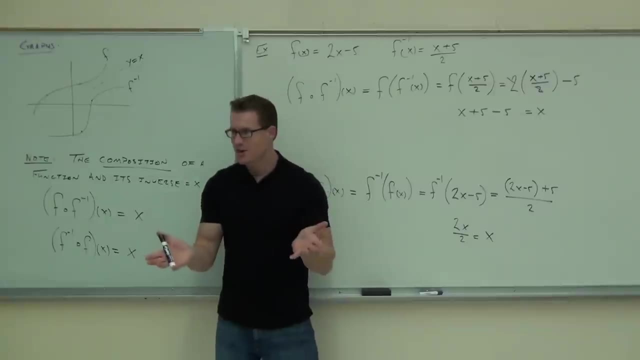 Of course, if we have 2x over 2,, how much is that going to give us? x. Did you come up with the same thing both ways? Yep, This is the only time in the history of mathematics where you will compose two functions two different ways. 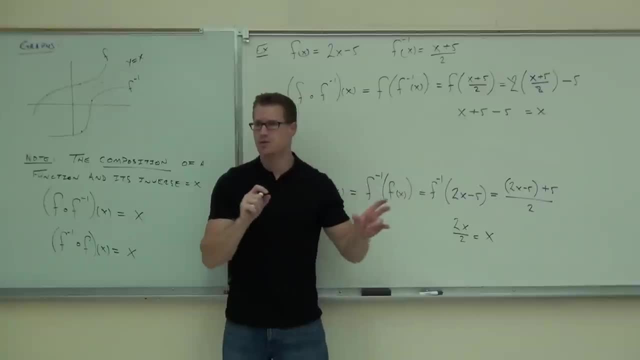 and we'll give you the same answer. The only time that happens is if they're inverse. That's it And that will be x. It will come up with x. Would you really feel okay with the idea here? So on our day today, on our section, you should know how to do a few things. 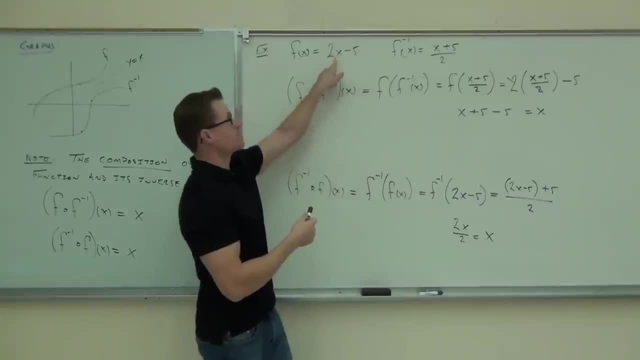 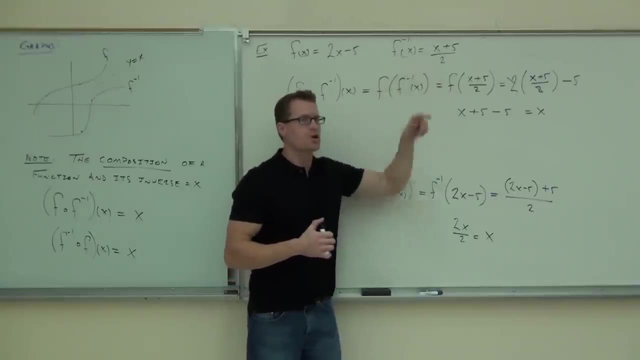 Firstly, you should know how to find an inverse. If I just give you this, you should be able to find on your own that thing. Not just that you can do that, Yes, no. Also, you should know that, graphically, all that's happening when I'm flipping my x's. 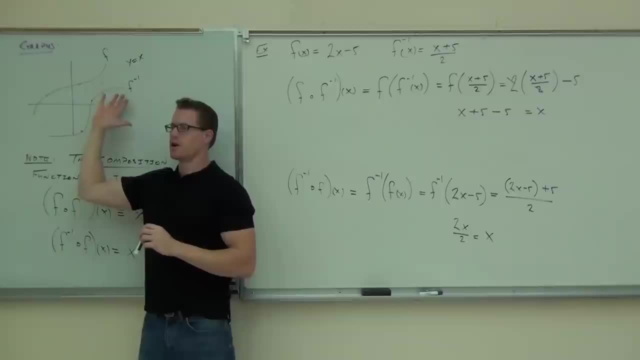 and my y's when I find my inverse. it's taking this function and reflecting it across a diagonal line. that's y equals x. That's the second thing. Are you guys okay with that? Yeah, Third and final thing, you should be able. 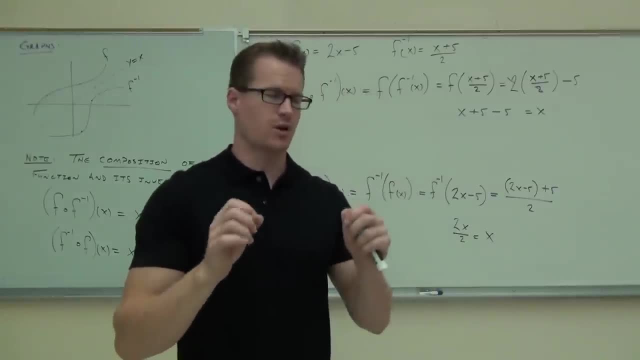 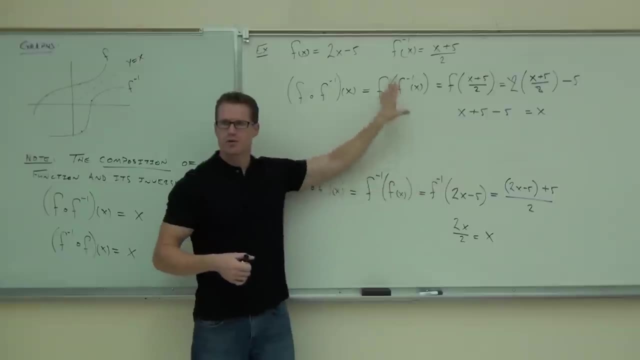 to check whether two things are functions- oh, I'm sorry- whether those two functions are actually inverses, by composing them, By taking one of them and putting them inside the other. Now do you have to show me both? No, I really don't care. 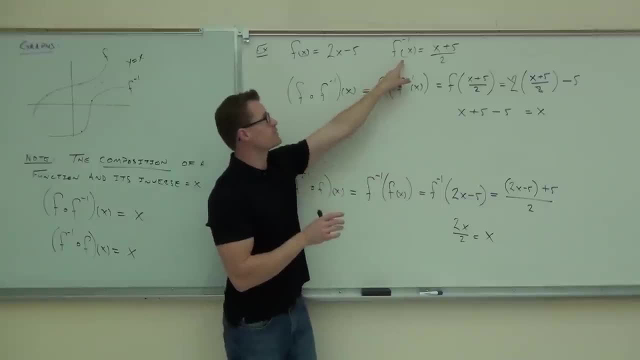 Just pick one of them and compose it. Compose your f inverse inside your f of x. If it comes out to x, it's an inverse. If it doesn't come out to x, it's not an inverse. So if you're a little sloppy on this work, go back and look at your. 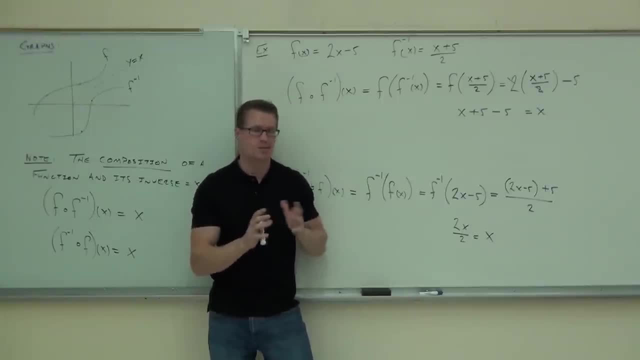 find those compositions from the last section. That's going to help you out, because that's all we're doing. We're just composing those things. That's why we went quickly through that. We've already done that. Can you please show me by a show of hands how many people feel pretty good? 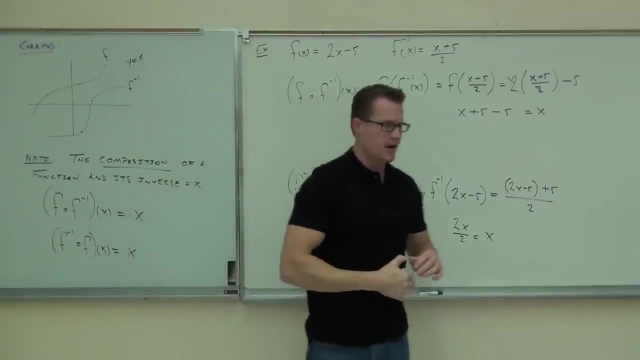 about what we talked about so far. Okay, good. Now there are some specific functions we are going to talk about. The first one that we're going to cover is the function of the inverse. 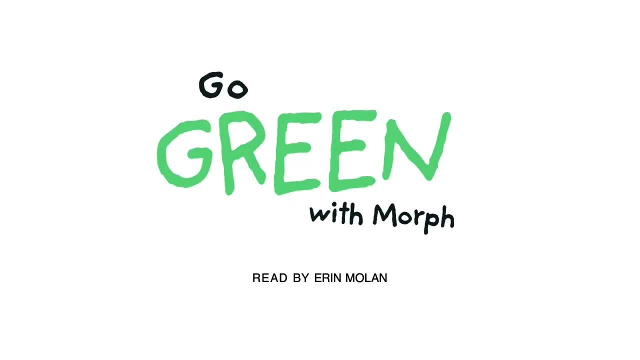 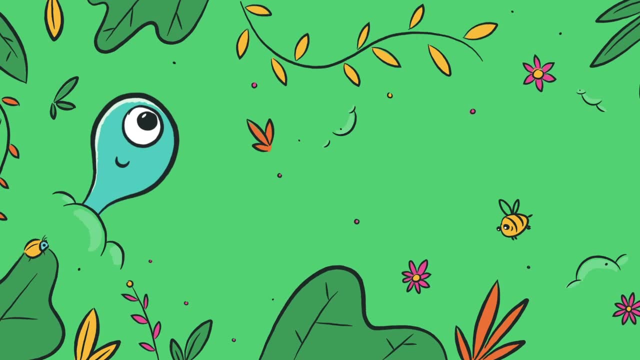 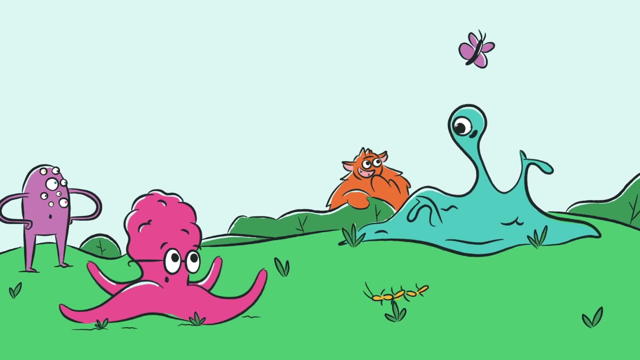 Morph's an eco-monster. He's green inside and out. It's rivers, trees and bugs and bees he cares the most about. His friends want to be green like him and help the planet too. There's lots of ways to help said Morph. I'll show you what to do. 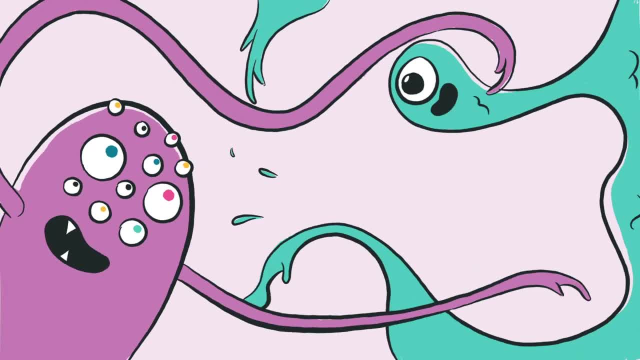 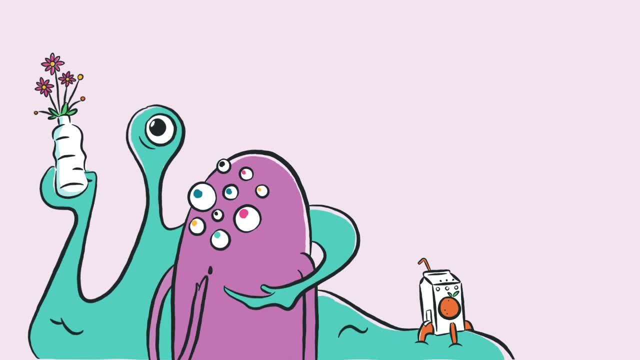 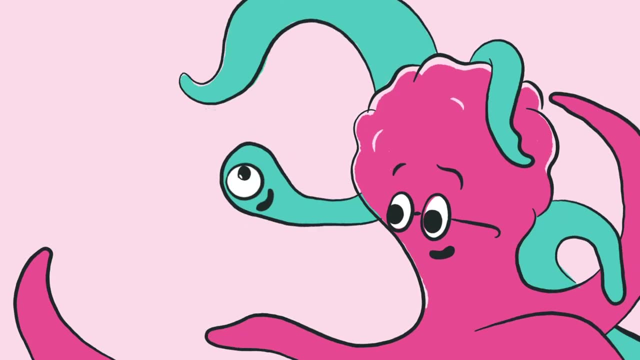 Let's be green together. It's easy if you try. Purple can be green, said Morph, and I can show you why. Always check the labels on your milk or orange juice. If they can be recycled, they can have another use. Let's be green together. It's easy if you try.